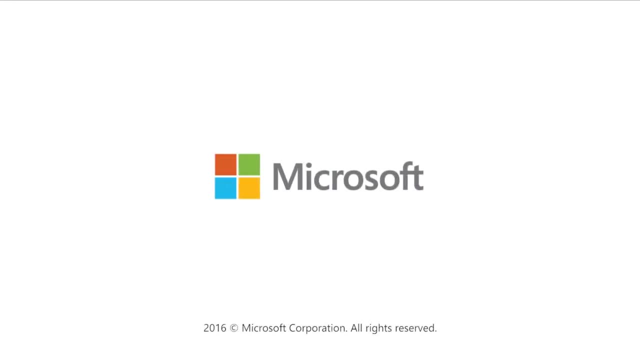 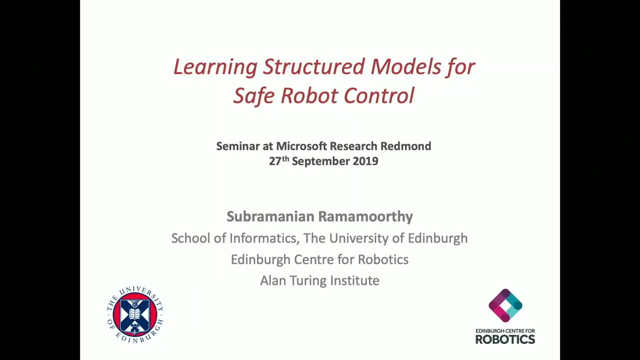 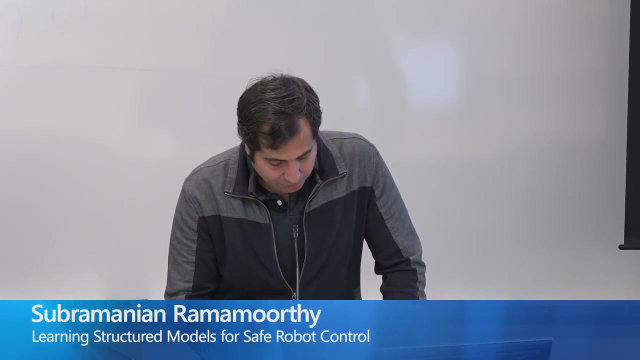 So it's my pleasure to introduce Dr Subramanyam Ramamurthy, who is a reader at the School of Informatics University of Edinburgh and he's also on an executive committee for Edinburgh Center of Robotics. So he did his PhD at UT Austin and since then he has been faculty at Edinburgh. He's also a Turing Fellow at the Alan Turing Institute and also a member of the Young Academy of Scotland at the Royal Society of Edinburgh. 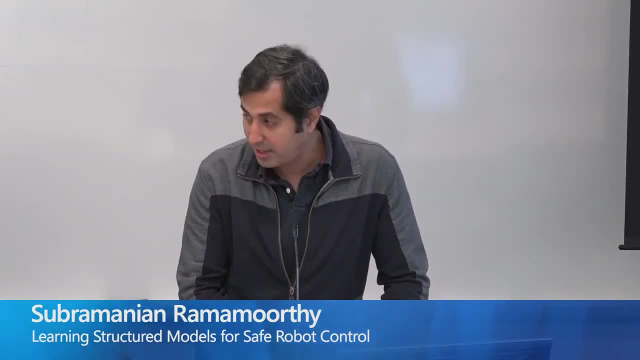 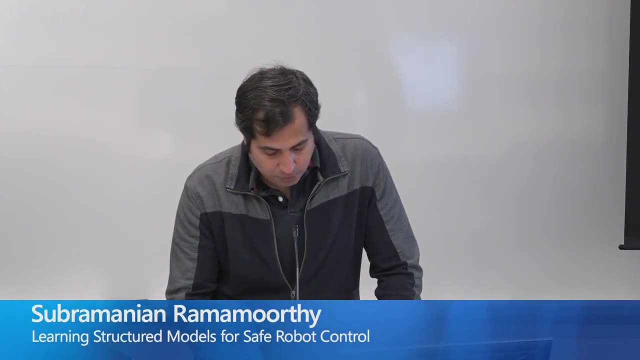 And if all this is not enough, he's also Vice President of Prediction and Planning at 5AI. So Dr Ramamurthy has done an immense amount of work, and his research focuses specifically on robot learning and decision-making uncertainty, And with particular emphasis on achieving safe and robust autonomy. So looking forward to your talk today, Dr Ramamurthy. 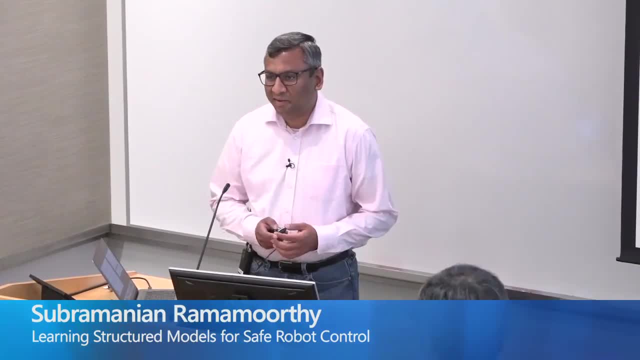 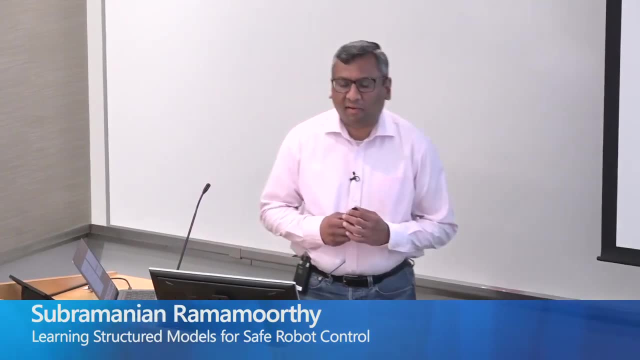 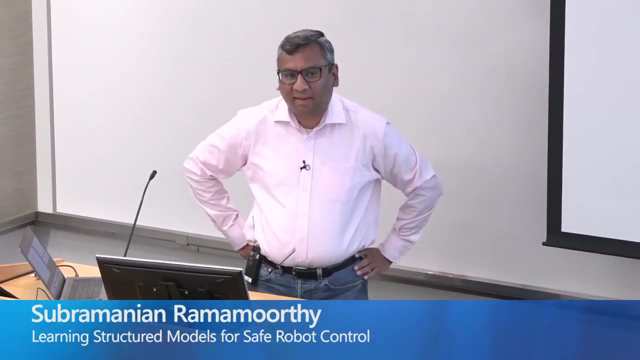 Thank you, Ashish. So it's a pleasure to be here. It's good to see some familiar faces and many new faces. So to follow up on the introduction a little bit, so I'm a robot learning person and with a little bit more robotics, and by that I mean that in the way that we formulate questions. 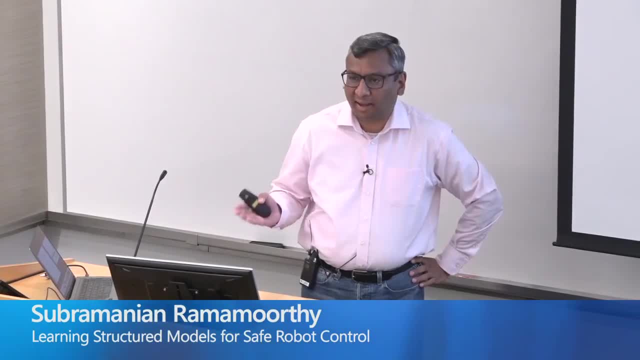 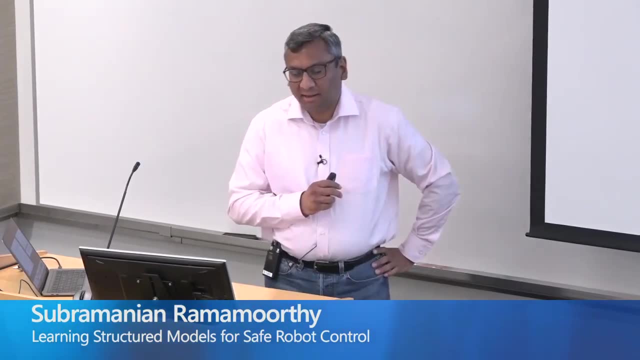 we really are interested in solving complete robotic applications. So it's not just that we are using robots, but we are actually interested in taking them out into the field. I'll touch upon this a little bit towards the end as well, but I thought I'll begin then from that perspective and tell you about where our questions are coming from. 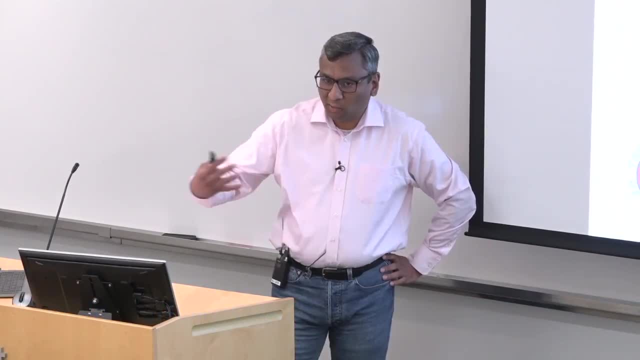 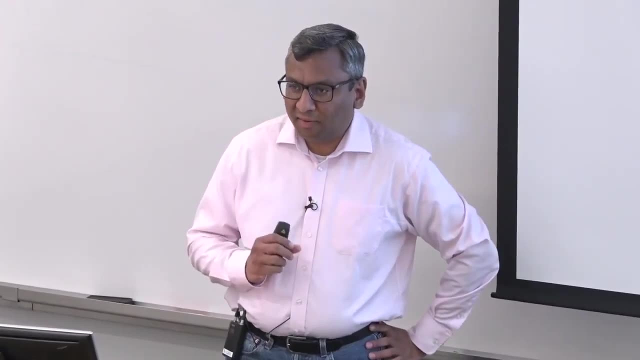 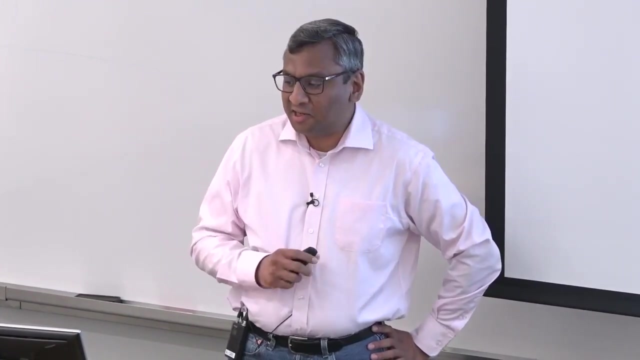 And then much of my talk will be on the machine learning methods that go into making these robots autonomous and safe. The other thing I might say is that I probably have a few more slides than I really want, So I'm quite happy to have discussions along the way, because the things at the very end are skippable. 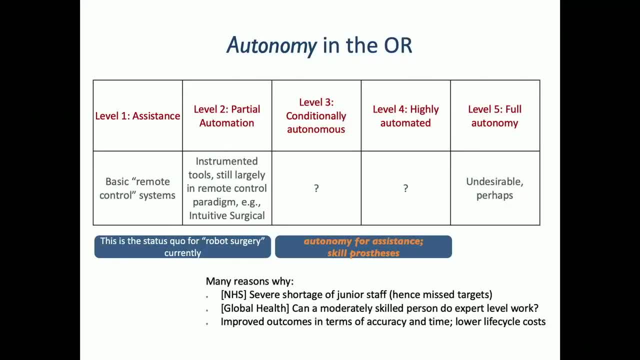 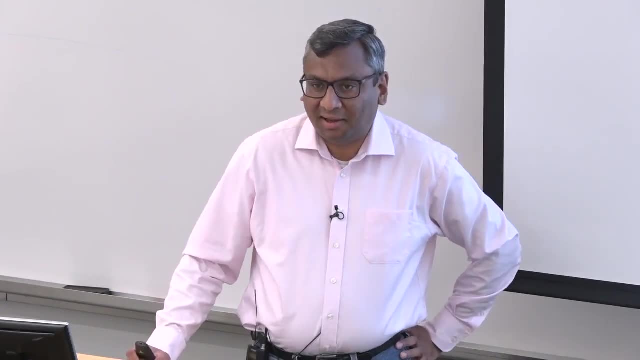 So, to start with, I thought I'll give you a little bit of a perspective on how I think about autonomy. So the idea of having a robot that makes decisions for itself, it goes back to the beginning of AI, So we've always thought about the idea that a robot 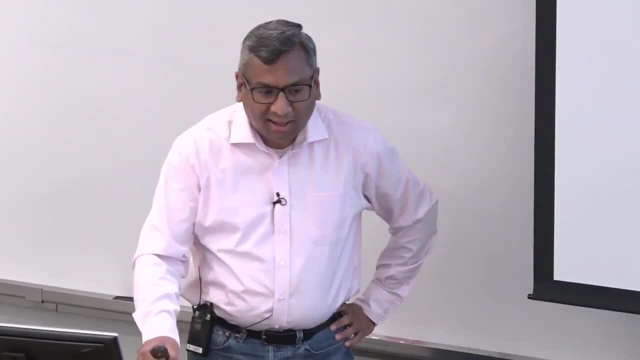 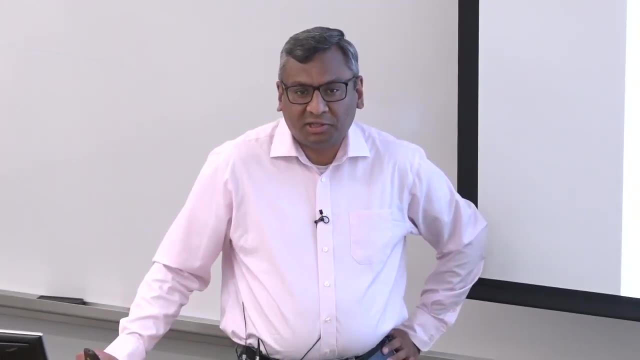 at least as AI researchers think about it, should have a lot of autonomy in it. But then when the rubber hits the road and when you take the robot to the real world, then the situation looks slightly different and then the questions look slightly different. 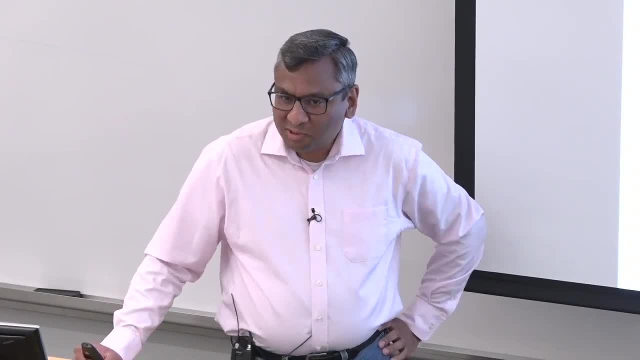 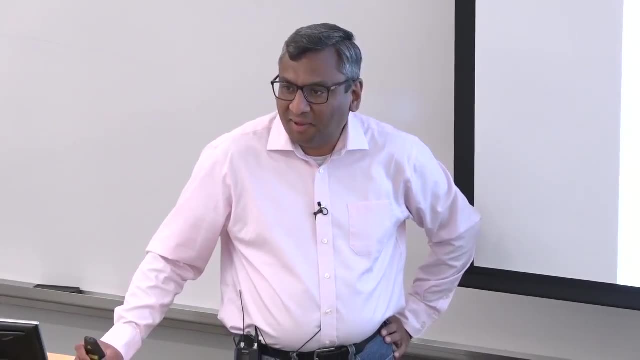 So I spend a little bit of time thinking about autonomous vehicles, and in that space there's a very clean classification that people have come up with, But since then people have adapted it to other applications as well. I thought I'll actually apply that classification to. 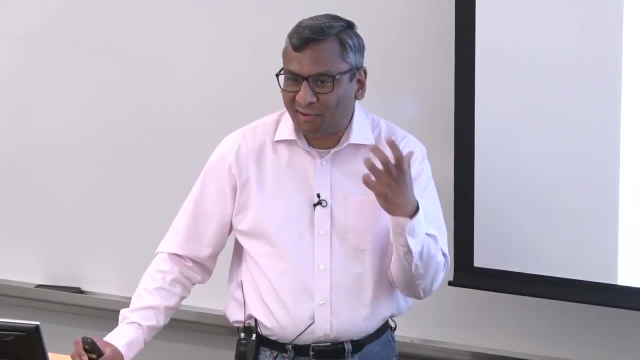 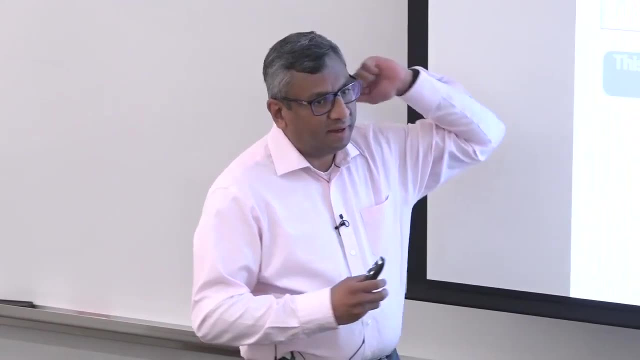 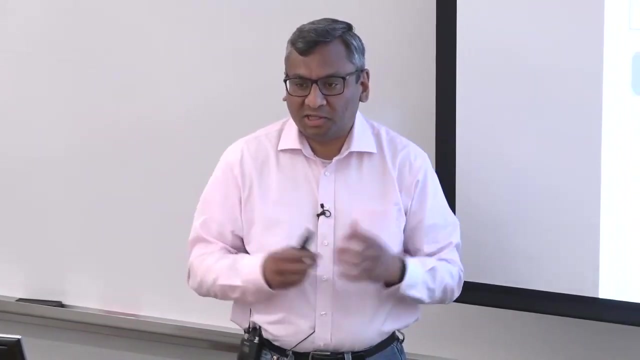 this other application of surgical robots to give you a flavor for exactly what people think about autonomy. So if you think about there being a categorization on the one end of the spectrum, you have what we would call assistance quote-unquote, which means that it's just really a basic remote control robot system. 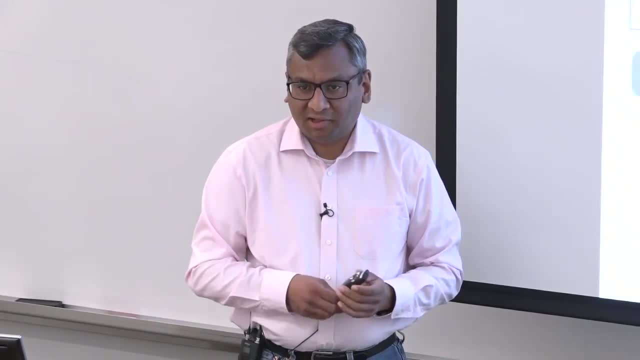 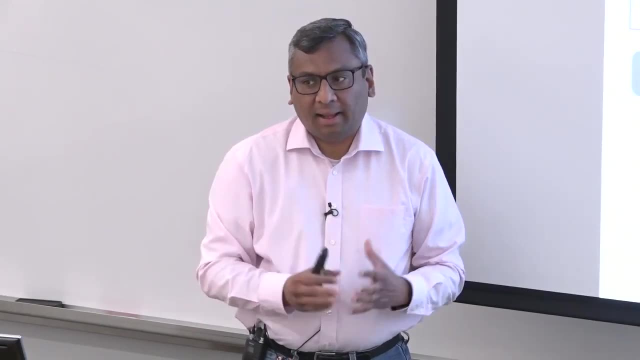 So if you're thinking about this being used in an operating theater, we're saying that the tools have a little bit of controllers inside so that if you shake your hand then the tool doesn't shake. It's not very sophisticated in the sense that. 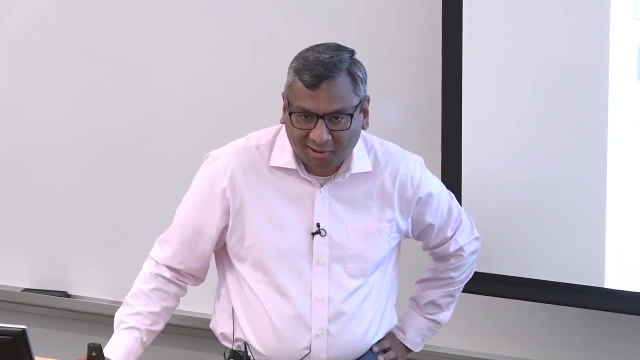 the tool will not do anything that you don't explicitly command. it will not do anything that you don't explicitly command. it will not do anything that you don't explicitly command. it will not do anything that you don't explicitly command. and if you make a mistake, 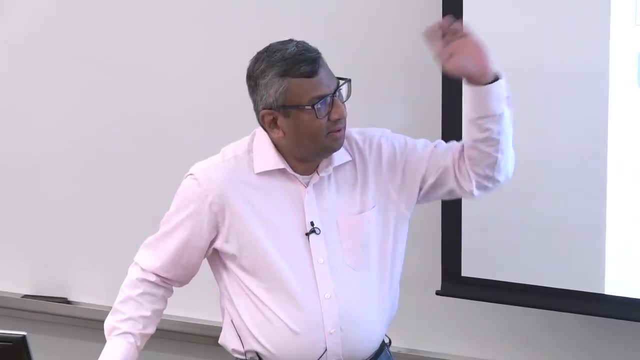 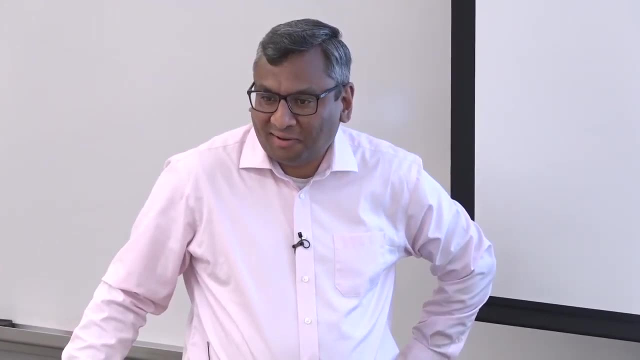 it will make a mistake. That's one end of the spectrum. The other end of the spectrum, which is science fiction, is that there are no surgeons anymore, As a lot of people advocate on Twitter. all of these people have not been trained. 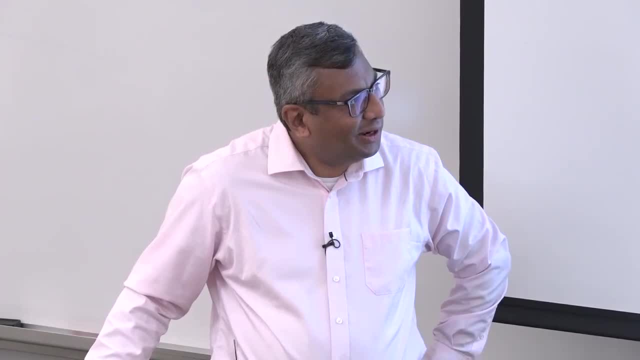 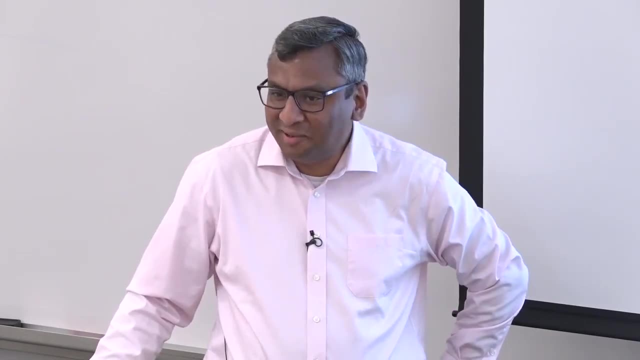 they've gone away, they've disappeared and robots have taken over the world. For a variety of reasons, especially in this domain, you might agree with me that that's maybe not quite desirable, at least not yet, and there's no appetite for it socially at all. 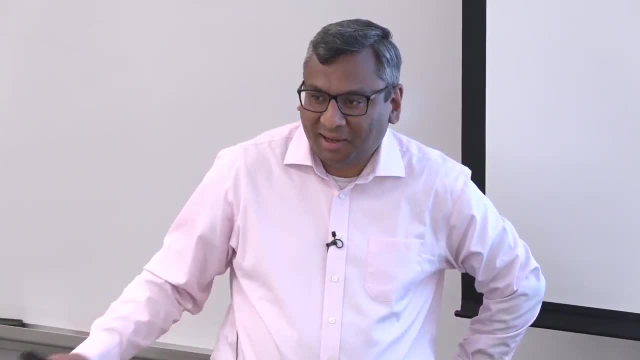 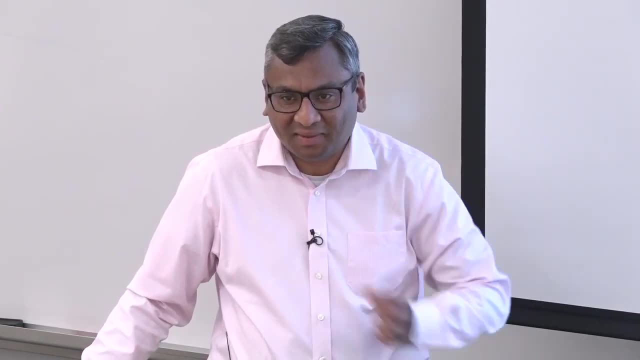 Also, when I sit down and speak to my collaborators who are neurosurgeons and so on, I don't see any evidence that in my lifetime we're going to hit level five. So really we are in those question mark territory. That's where we are operating. 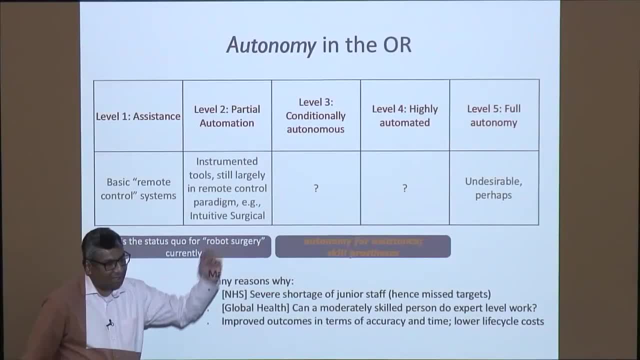 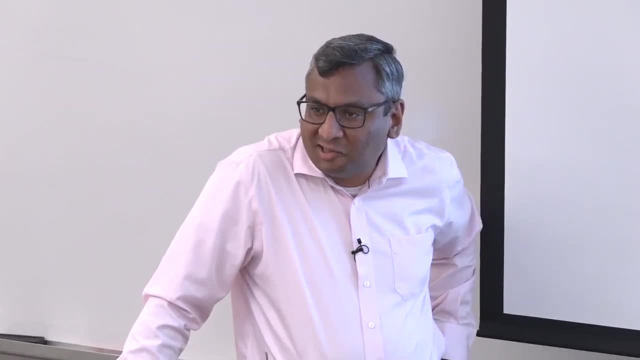 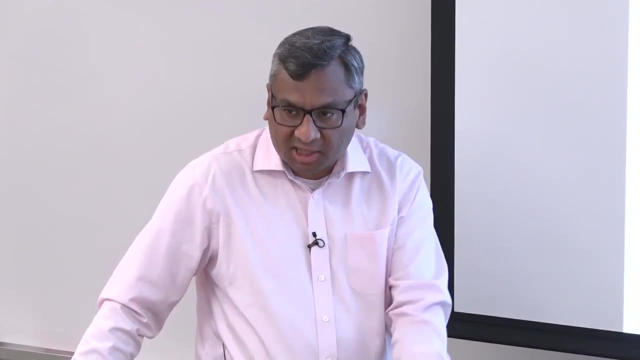 Sort of the boundary of where we are is the kind of thing you might see if you search under robot surgery in Google, which would be devices like intuitive surgicals, Da Vinci robot. What these robots do is they take over quite a bit of low-level sensory motor control. 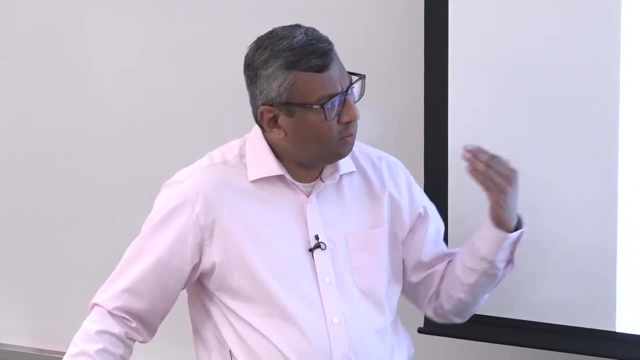 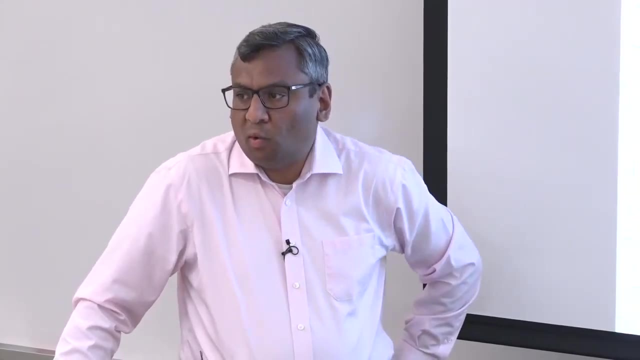 and then they leave the decision-making to the user. So the question is: can you push the boundary from just dealing with the low-level control a little bit towards the decision-making side, and then what might you want to do? There are a lot of social reasons why we want to do this. 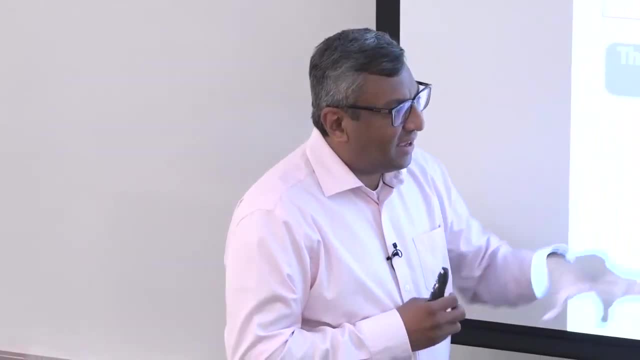 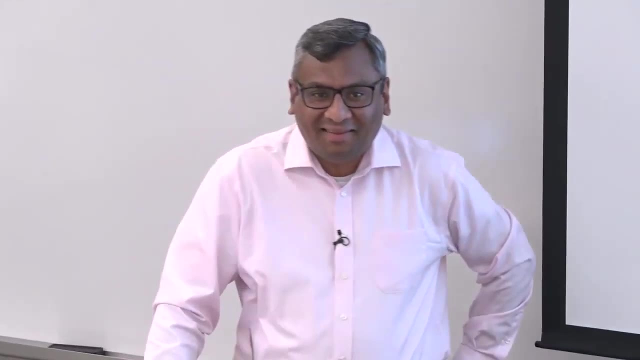 So in the UK context, which is where I'm situated, there's actually a serious skill shortage. So, unlike worrying about taking people's jobs, we actually have the opportunity to do that. That's the opposite problem, in that surgeries are actually being 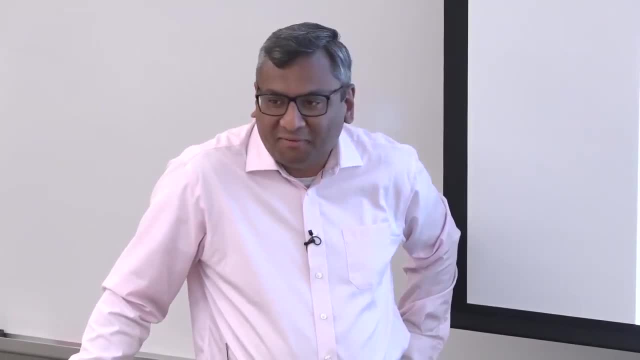 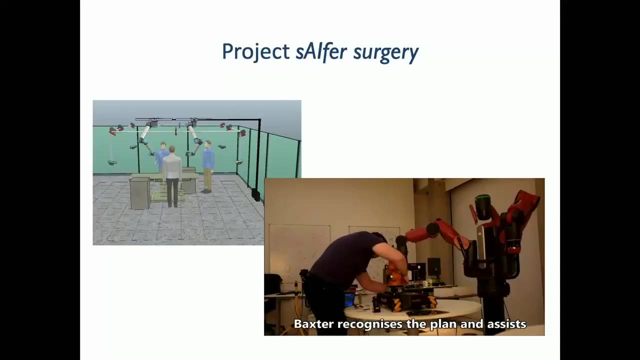 postponed because we can't find enough of a team. So it would be perfectly fine to build such a system Now, from a technical point of view, as a roboticist, when we start thinking about what actually we might want to do. So here's a very basic example of 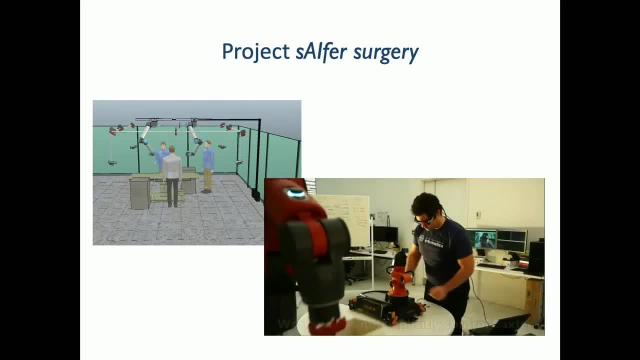 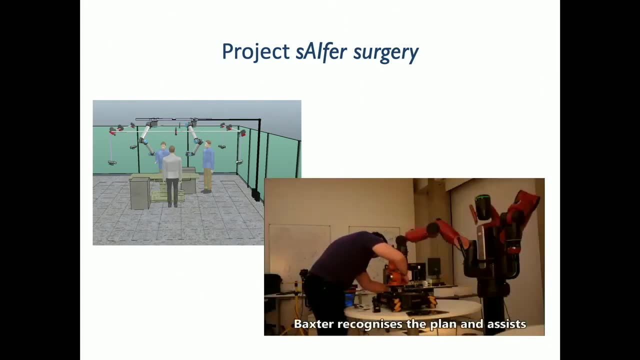 the kind of assistance you might want a robot to do. This is not surgery. This is actually assembly in more of a manufacturing context. But this is in my lab and that's my PhD student, Svetlin, and what's going on here is that you have 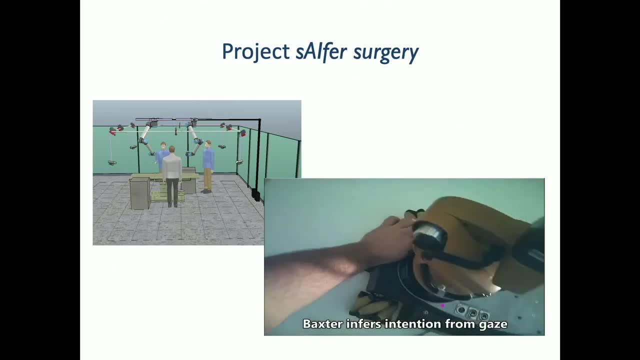 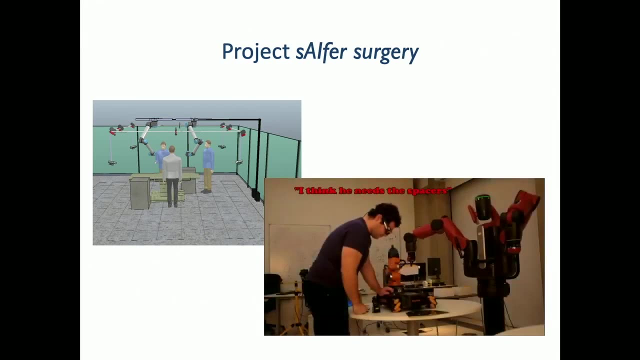 this Baxter robot that's trying to help Svetlin as he's assembling another robot, His sequence of movements, it's a plan, So he's going through. pick up this part, put it on top of this. once I have it, get something else, assemble it, and so on. 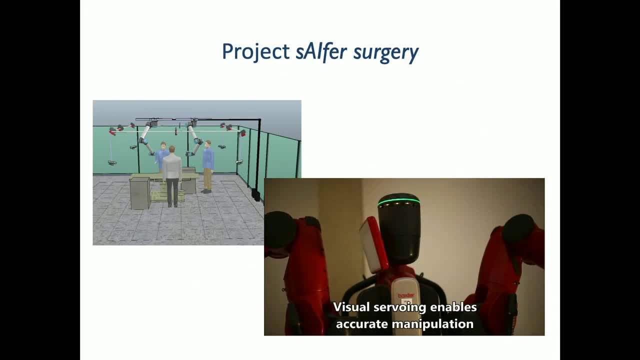 So it's something that you could specify at a high level, but there's a lot of low-level complexity to be dealt with. What the robot is doing is, from vision and eye tracking, it's estimating what this plan state is and then depending on 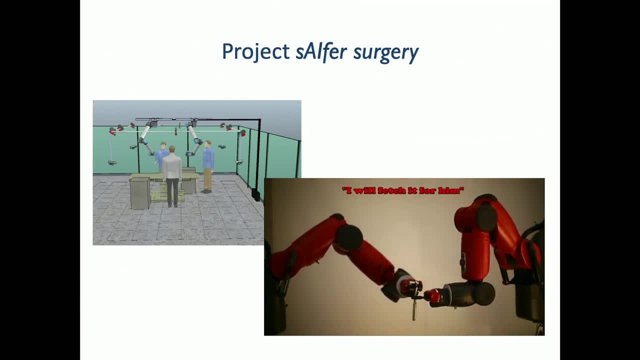 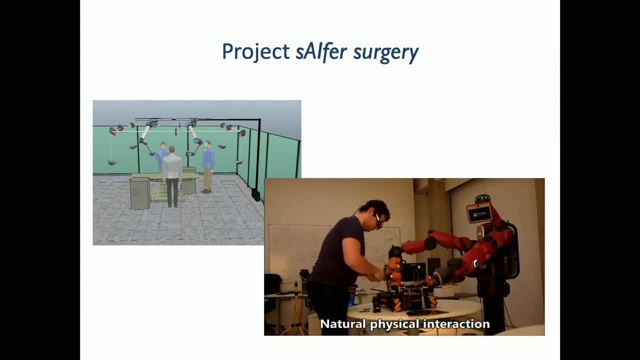 what that current plan state is in the execution cycle, and this has branches and so on. Based on that estimation, it's taking what would be an appropriate action, and this business of what is appropriate has been told to it ahead of time. That violet dot that you see, there is us fusing vision and eye. 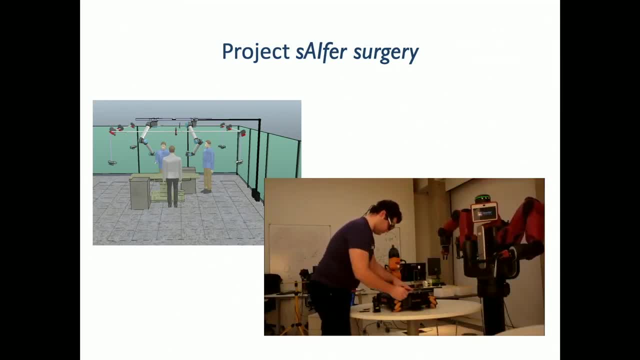 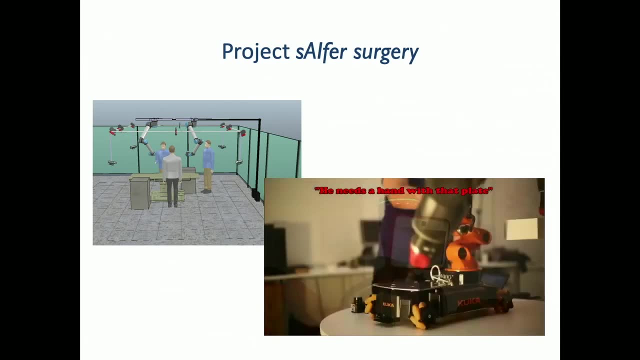 tracking and putting it in 3D so that we can visualize what's going on. So that's a basic example. In my lab currently we are setting up a more serious setup which would mimic an operating theater, and we are trying to look at whether we can automate things that are done by 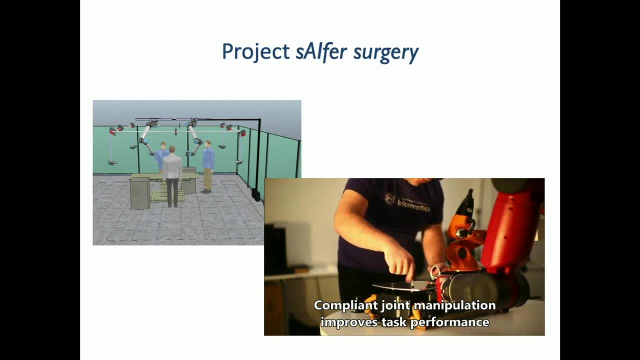 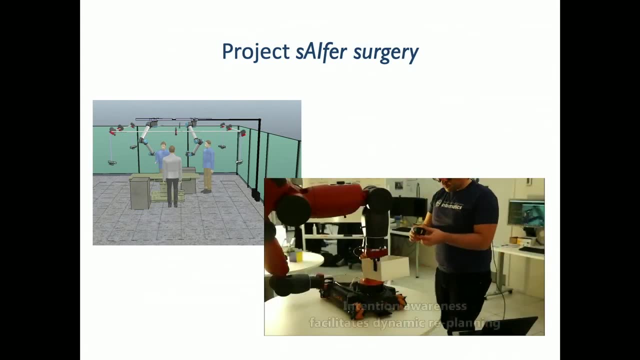 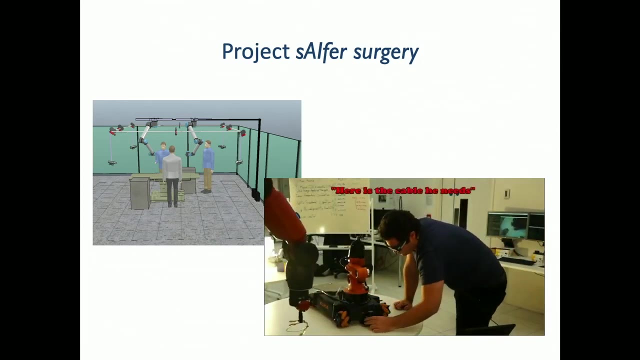 a typical nurse and a junior surgeon working our way up. The point of picking an example like this is to motivate questions, not just in terms of wouldn't it be nice if, but asking: what would these people really want and can we actually deliver that? 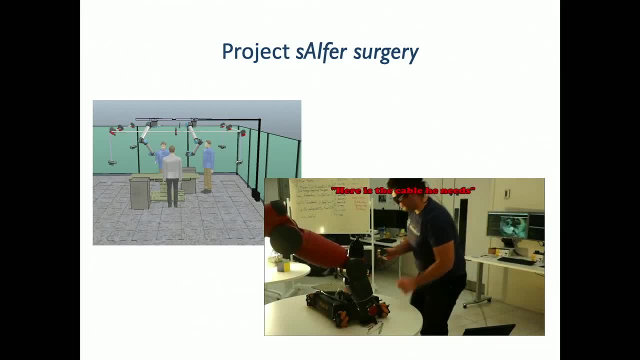 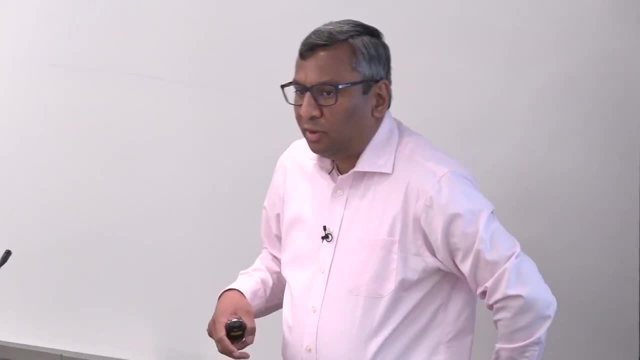 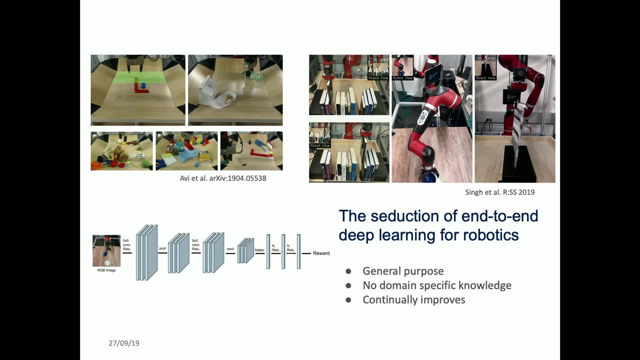 Now, looking at it from another point of view, of the actual tasks involved. there are grasping tasks, manipulation tasks and so on. I think many of you are probably aware by now that there's a lot of excitement in the robotics community about the use of Deep Neural Network methods. 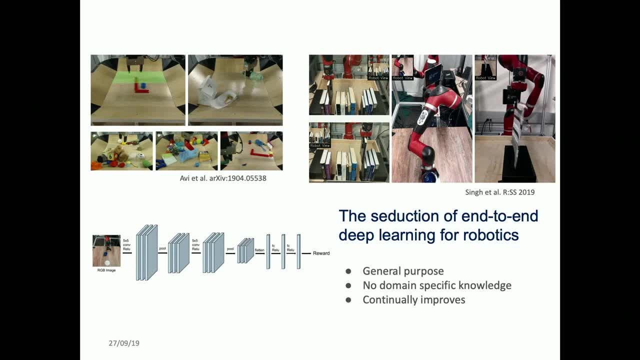 So here are videos taken from various groups around the world doing really exciting things with robots. So people are really able to do interesting things, particularly when it comes to specialized tasks like grasping arbitrary objects and figuring out what the physical properties of objects are, and so on and so forth. 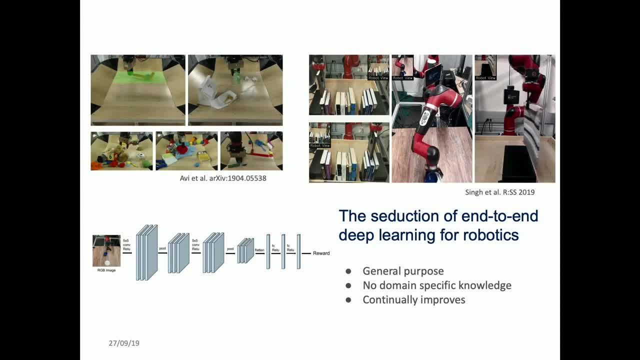 In the more extreme version of this, when you think about it, what people are excited by is the fact that there is the possibility of having a completely general purpose mechanism which doesn't need any domain-specific knowledge at all, and then it just continually improves. 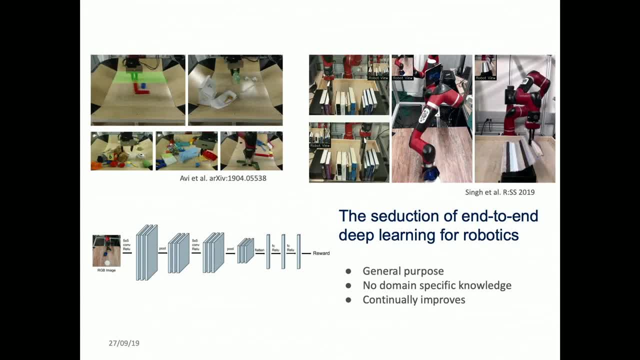 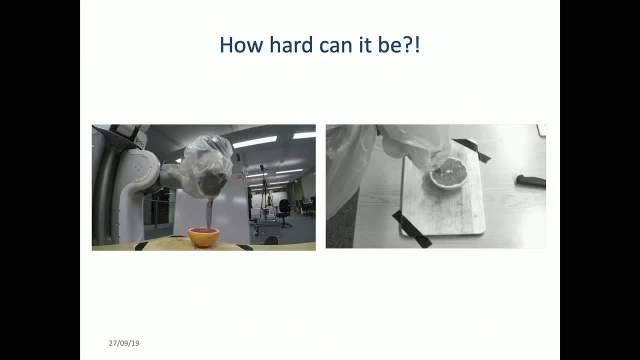 That's what one is trying to do with a typical reinforcement learning setup. But then if you look a little bit beyond the label, you'll find that actually it's not so straightforward. I mean as somebody who runs a robot lab. here again this is back to my lab- 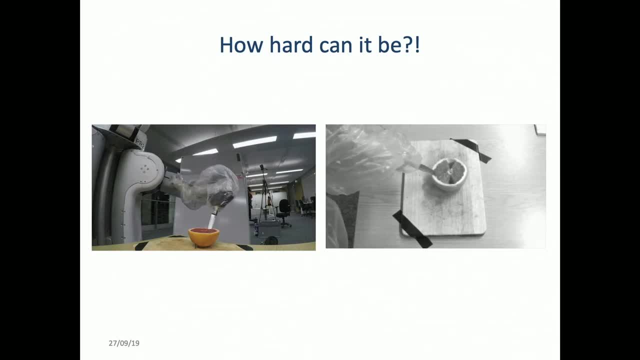 this is one of my robots, and this is a task that we picked as what we would consider to be the most basic task that would interest a surgeon. It's only after we did this that we got meetings with the surgeon I work with, So the task here is to scoop out a little slice of grapefruit. 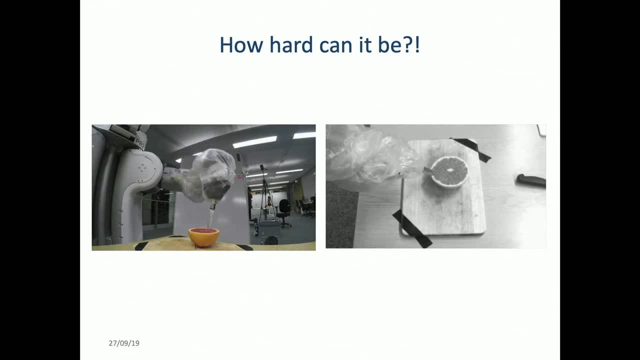 We took away the job of the second hand, so the grapefruit itself is pinned down to the board, But you still have to make some very careful judgments about how you want to move the knife and exactly what the force profile should be so that you can achieve this task. 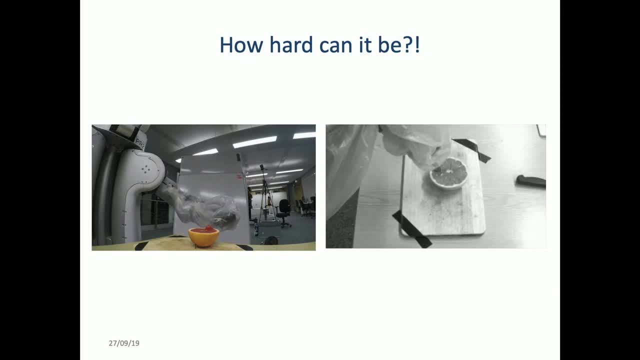 It's not as trivial as it looks, So we do it effortlessly, but we only do it as adults. Although it's just cutting fruit up, it's actually quite interesting because for the surgeons, they consider this to be step zero of what is actually. 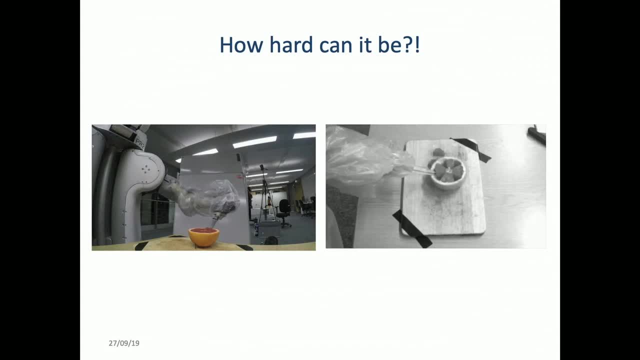 tumor removal. if you flip the hard with the soft, this is how a tumor looks in your brain, And so when I look at a problem like this, there are three things that you should note. The first is the fact that the modalities that 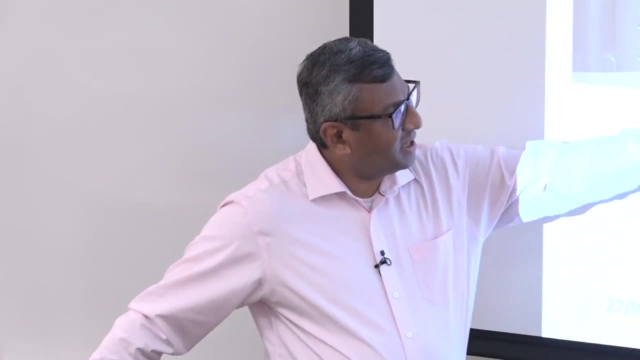 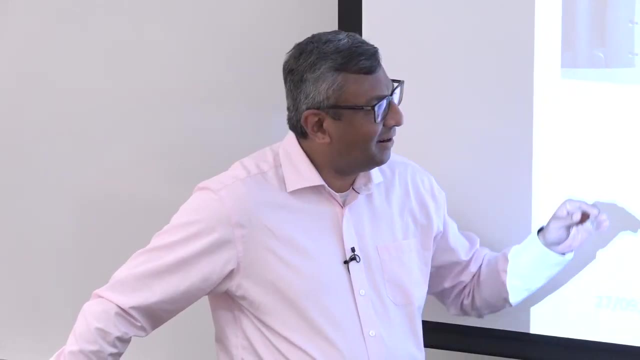 you need to complete this task are quite diverse. In fact, except for the very first point at which you insert the knife, vision is largely useless, in the sense that once the knife is gone and you don't know exactly what's going on underneath, 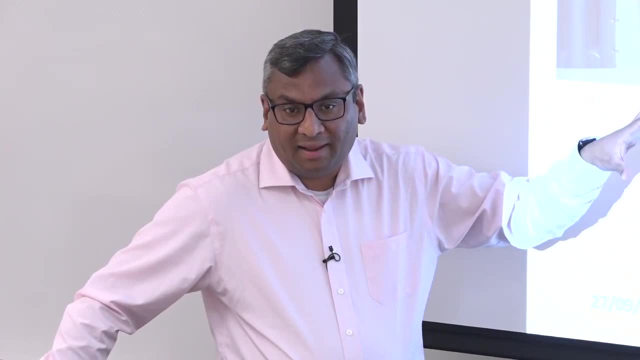 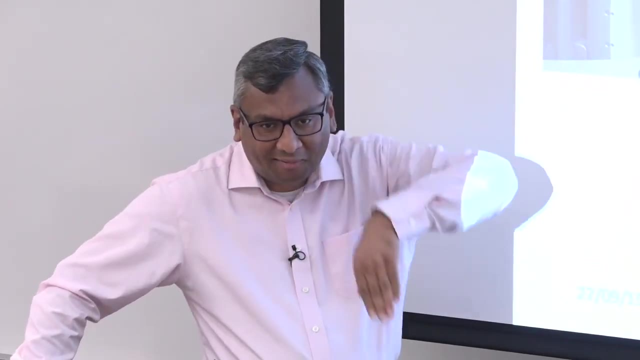 So a lot of it is in the haptic channels. But then for the haptic channel you don't have an exact model because it's just a fruit. You don't know what the internal irregularities are and you're trying to somehow find what that space is. 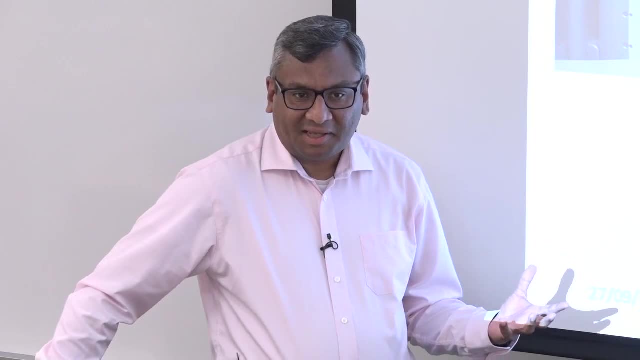 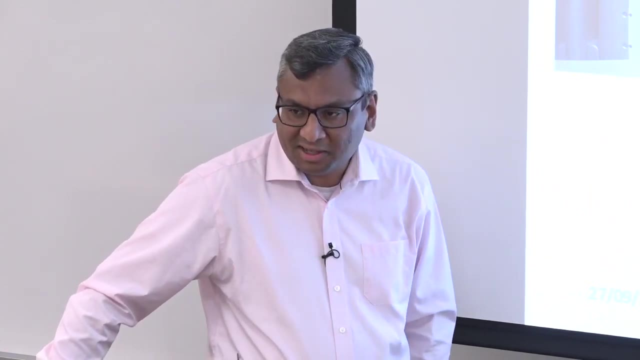 We don't have that much data in a domain like this, because we have to find the fruits, we have to find the demonstrator, we have to find everything. So we're not talking about billions of examples here. we're talking hundreds of examples. 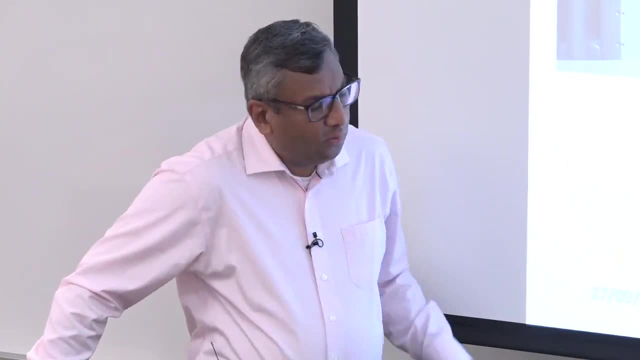 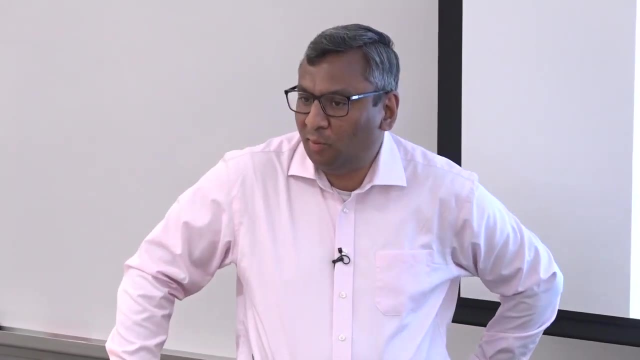 That's pretty typical of most domains we work in. So we have to think very carefully about how we want to set up our models, how we want to adapt our methods, what we want to pre-train, what we want to borrow, Which means that we can't just go in. 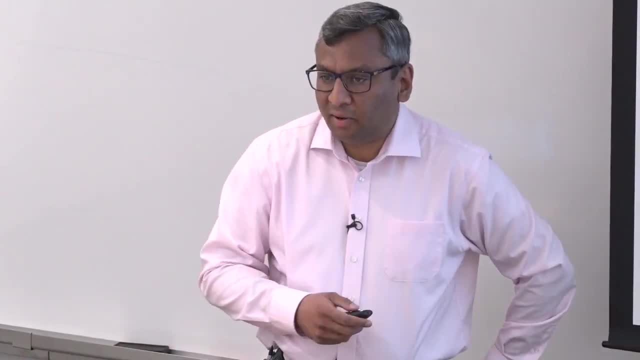 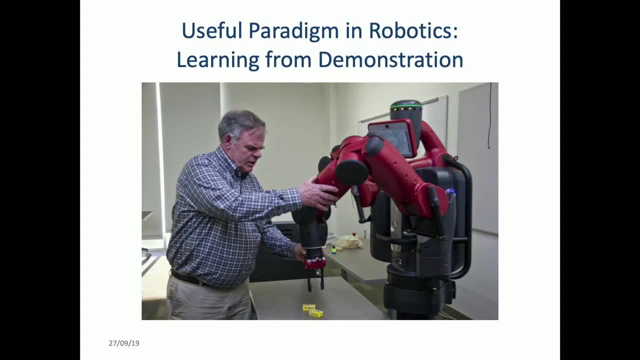 quite so naively with the use of the methods. We have to think a little bit about our methods Now in the robotics community, once you lay out all of these problems. the approach that quite a few of us pursue actively is called learning from demonstration. 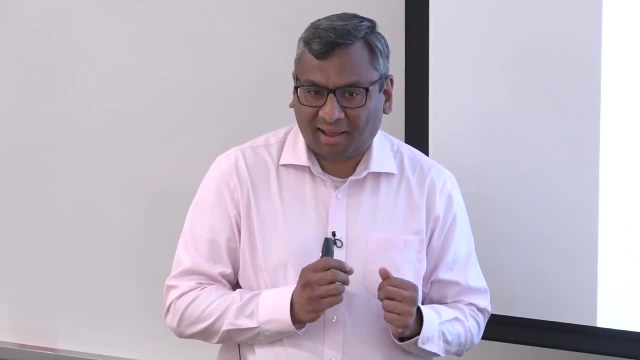 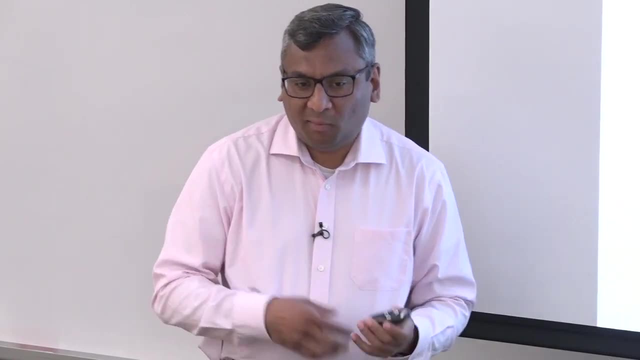 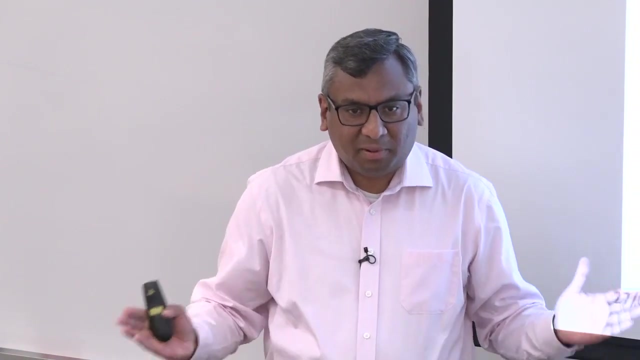 So, in the same way that supervised learning and certain forms of unsupervised learning are the dominant ways of describing a vision problem In robotics, probably one of the most exciting approaches for robot learning is to say that it is realistic for us to ask a human expert to give us examples of how a task is performed. 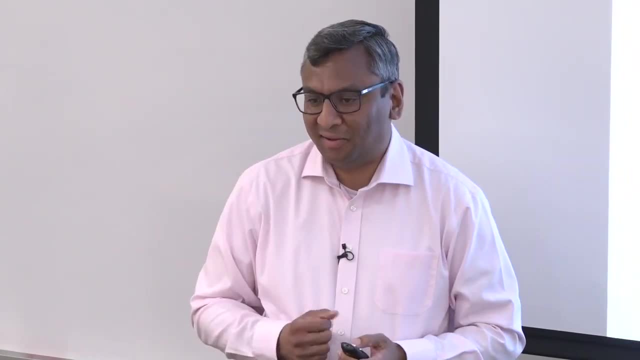 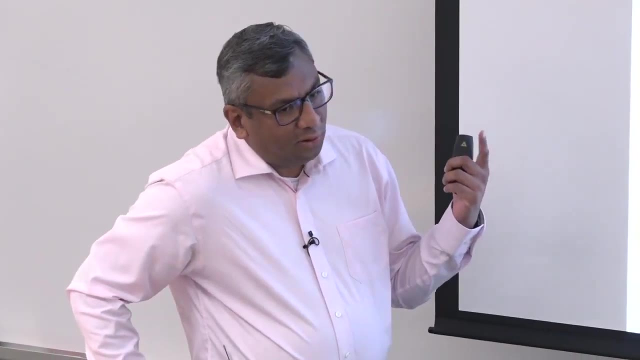 In that case, it's realistic for us to say: here are a collection of fruits, please cut them up for me, and we can get a normal person to do that much. Then, having done that, what we want to do is to pick up everything about what was the task. 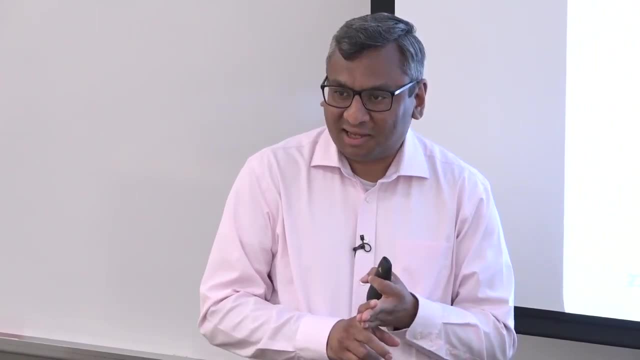 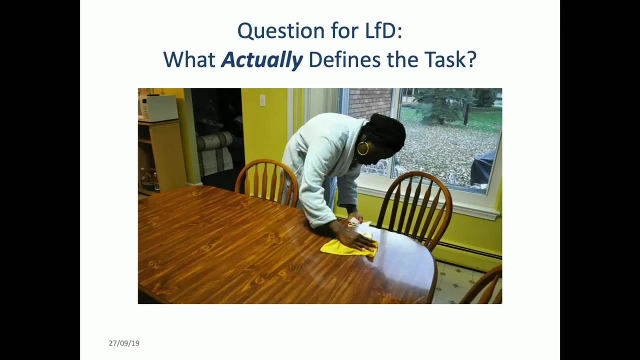 what variables were important, what specification describes this task and how do you want to actually perform that? So that's what we want to pick up from all of this, But then this question of what exactly is the task is not trivial. So here's maybe a typical snapshot from just day-to-day life. 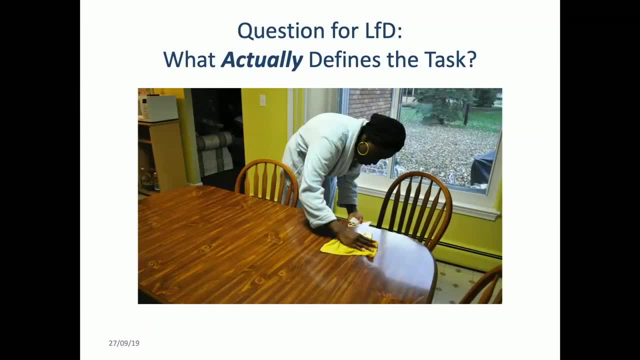 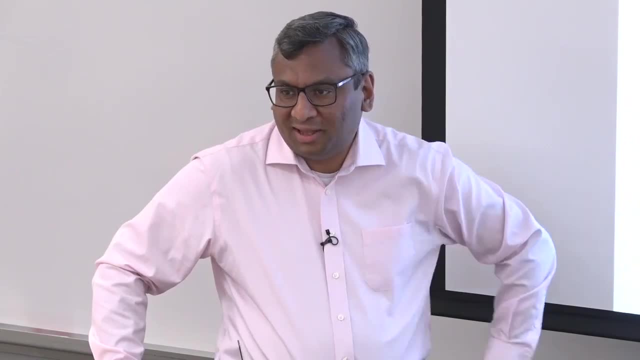 This lady is cleaning the table. If I just showed you maybe like a sequence of images like this in a video and I asked you what's the task, then you would say, okay, what she's doing is to move the sponge so that the dust comes off the table. 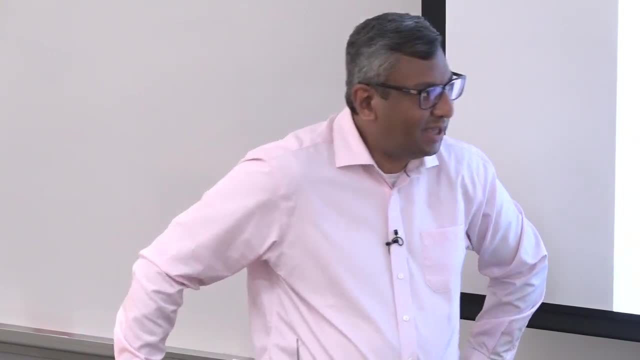 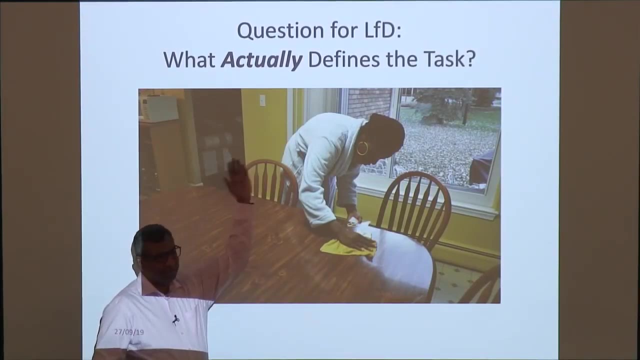 But then I ask you: are there specifications that you didn't pick up and you'd say, yeah, you have to apply a certain amount of force, otherwise the cleaning isn't going to happen. You have to control your velocity so that the dust doesn't spray all out. 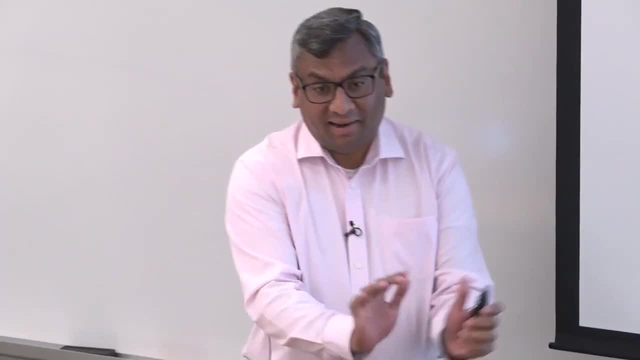 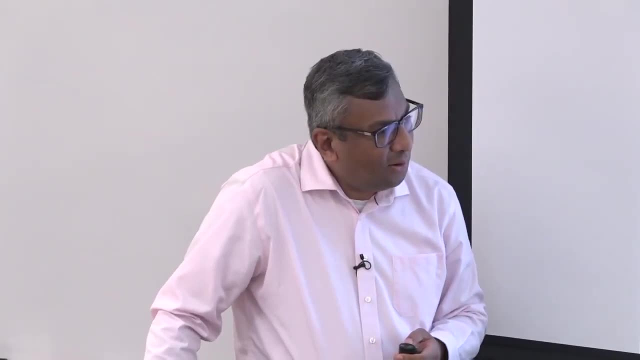 You have to make sure that you hit these regions. These are all hidden away specifications that are in the data. but then you can't just have it for free. You have to think a little bit about how you're going to get this Then. extreme examples of this might be like: 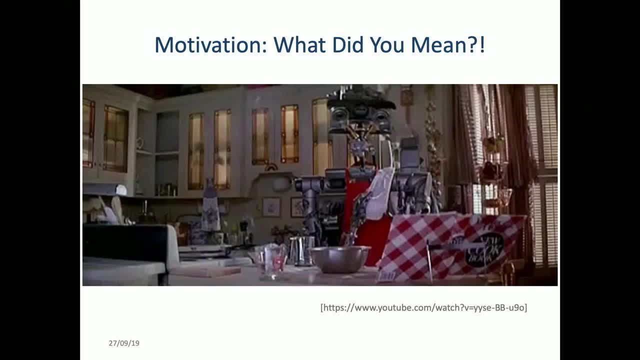 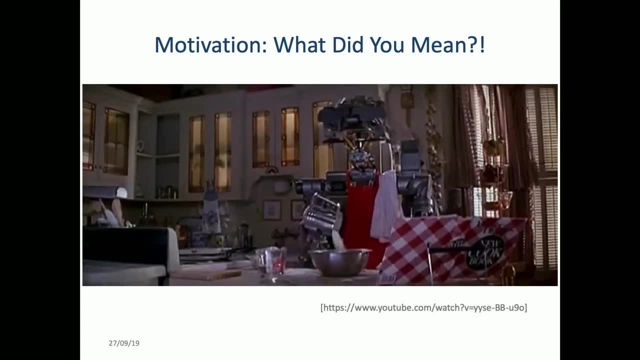 this. I don't know if do I have audio? Okay, So if I have audio, let's see: Fluffy pancakes, flour milk. In any case, I won't dwell on it. So for the people who are here, 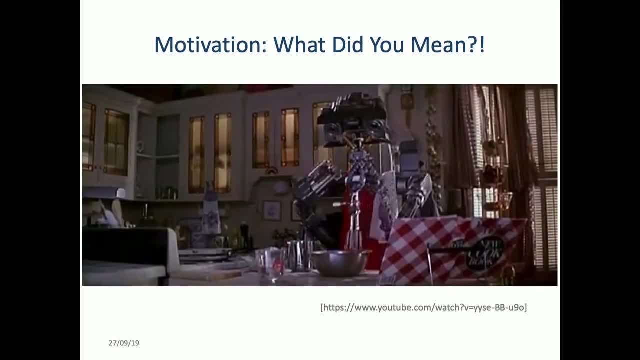 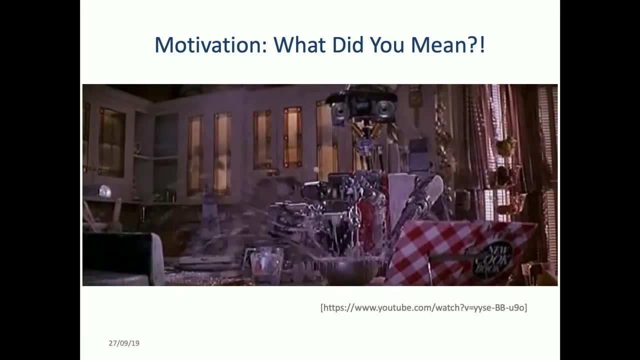 you can hear it, But the point is, here's an example taken from one of my favorite movies, which tells you that I'm a little bit older. What's going on here is that the robot has been given text instructions. Not only has it been instructed a little bit, 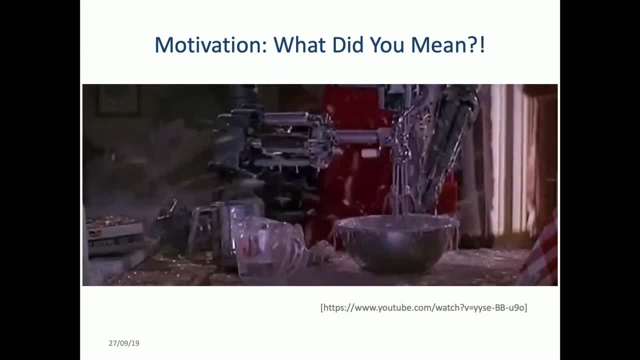 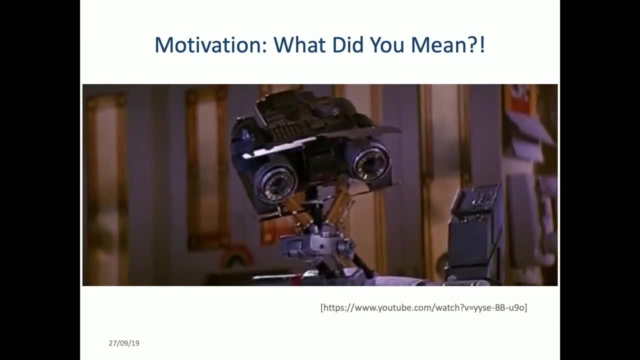 it's been given a recipe. What the robot is trying to do is to just follow the recipe It's been told: do this, do this, do this. it's doing it At each point. what makes this funny is that it has left out something about the specification. 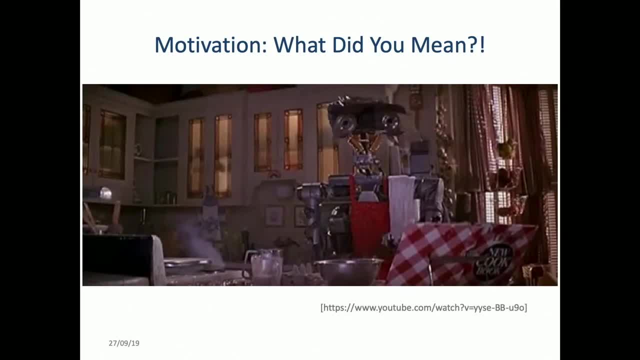 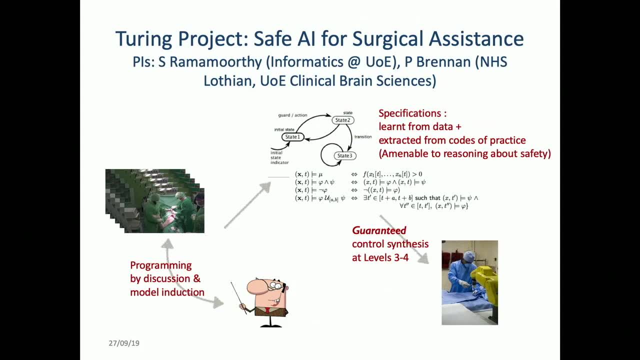 Things we take for given common sense. So the real question is: how are we going to get at all this and what do we want to do with it? So, by way of introduction, the way in which all of this is coming together for me is that I'm currently working on 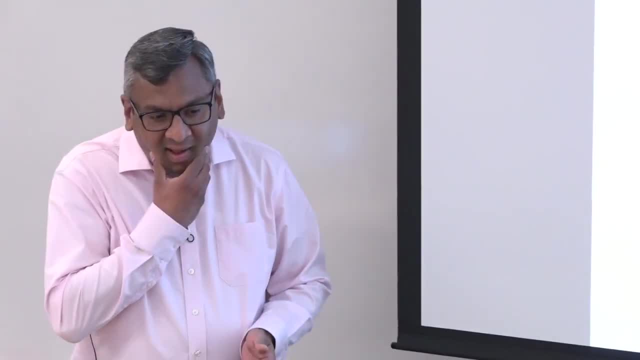 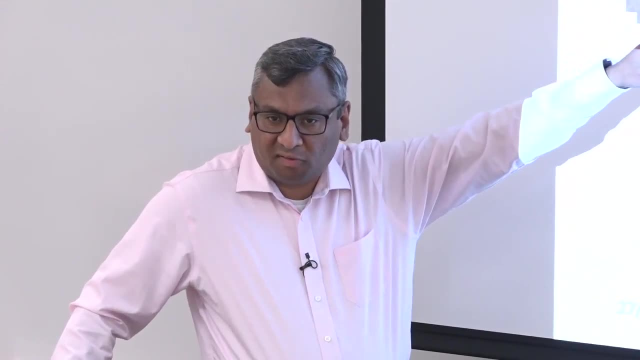 a project in collaboration with people in the medical community, Where we are looking at this cycle of: how do you go from expert demonstration to picking up what might be useful specifications from this, Finding ways in which you want to encode that representation and then reason about that representation? 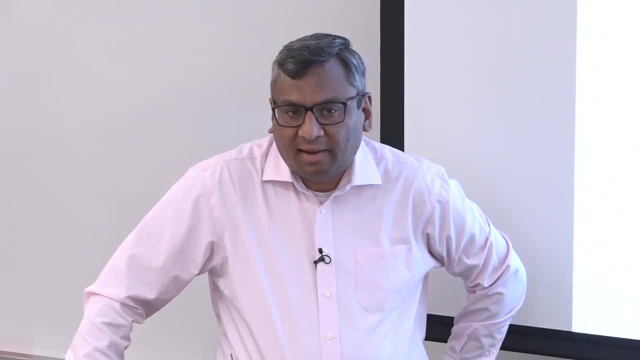 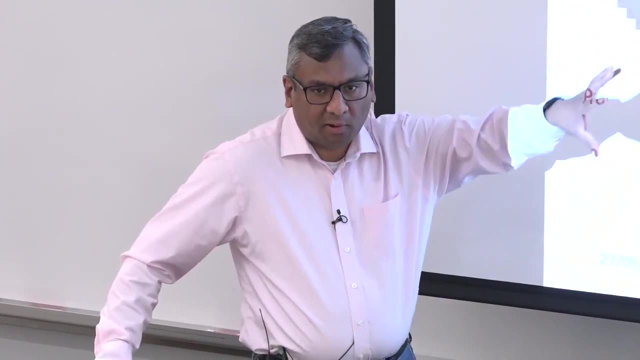 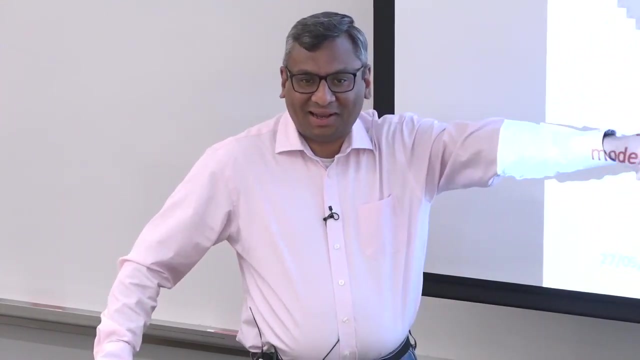 Then finding ways in which you can synthesize controllers that then respect these specifications. So the plan for my talk today is I'll show results from a few different projects that go through this chain. The challenge in a couple of years is to bring it all together so that I can show you. 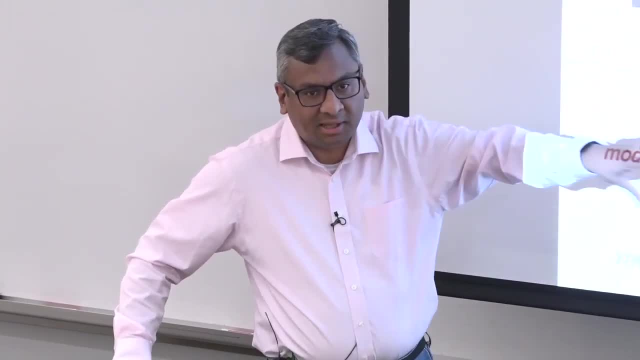 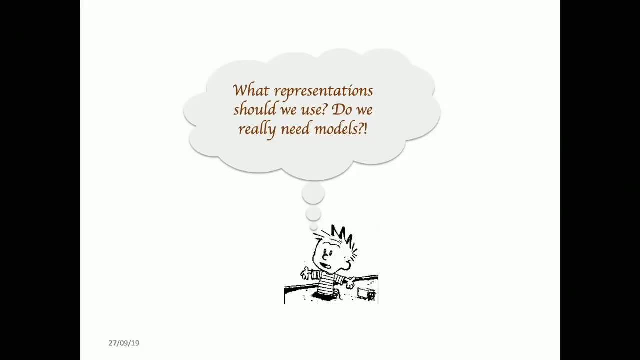 one slick video that does the whole thing. Today I'll show you bits and pieces that cover this landscape. So the big question, of course- and this is every time I go to a robotics conference- the last time I was at RSS, the last time I was at Coral- 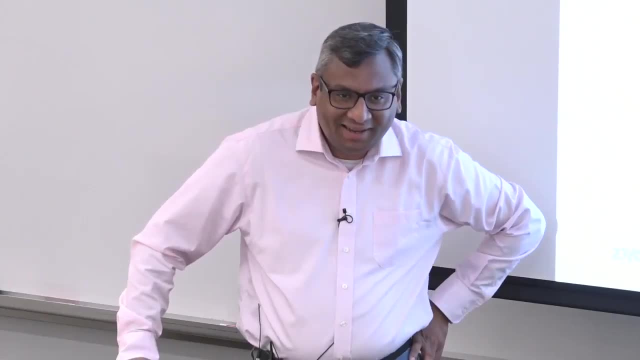 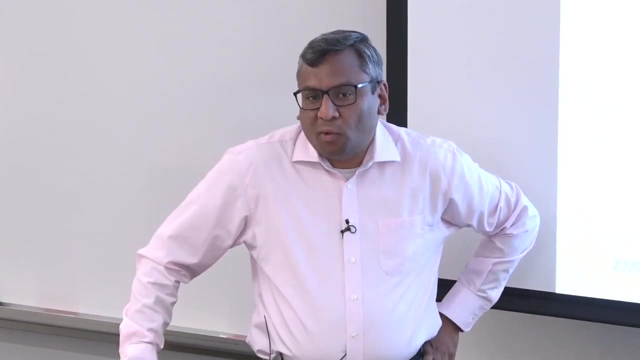 there's always a debate about what are good representations. Do we need representations? Should we be using models? This seems to be like the perennial thing that we all keep talking about. A lot of what I talk about will pertain to this. I have a very particular view of this. 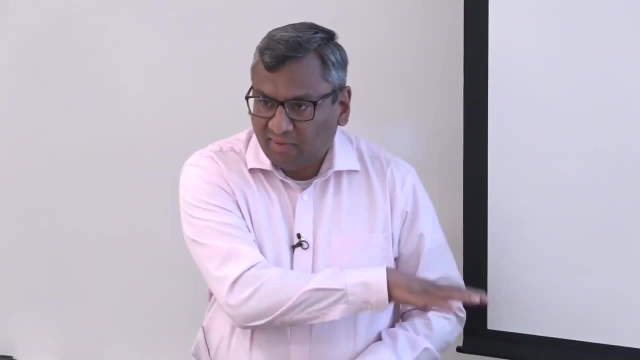 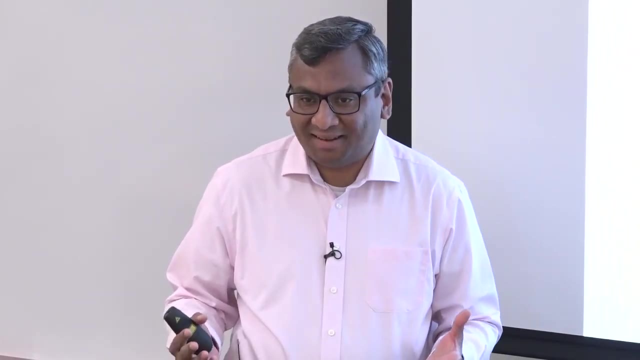 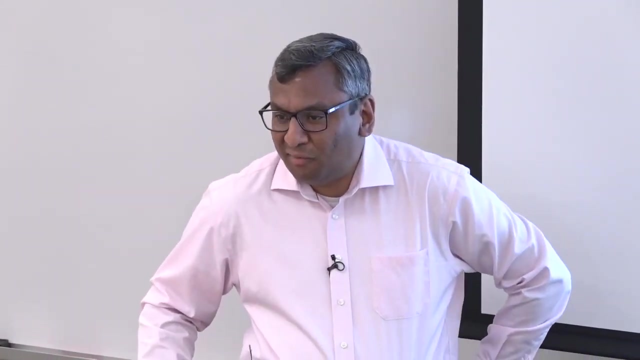 which is that if we want to get robustness in the sense that I'm hinting at with my introduction, then you really should use some useful representations that encapsulate common sense. I mean because we are driven by the application. it's not negotiable that you 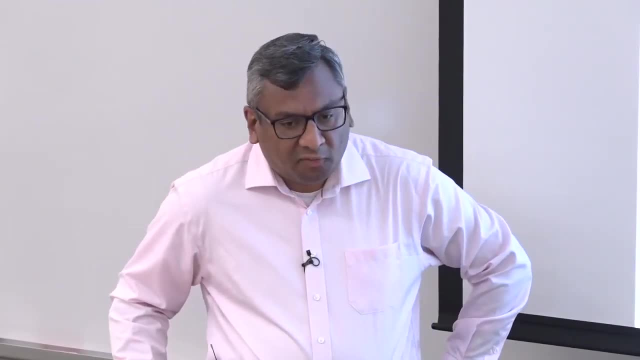 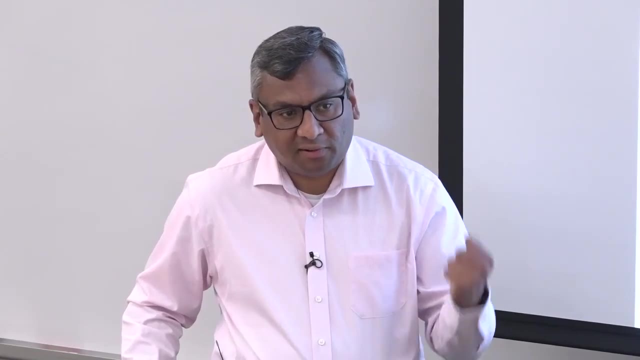 have to structure your models in a certain way. But we go further than that and our point of view is that there's plenty that we've learned as engineers from physical models, from control theory and from various principled approaches to reasoning about systems. 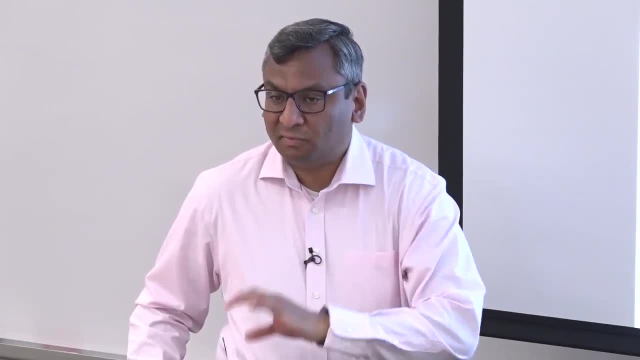 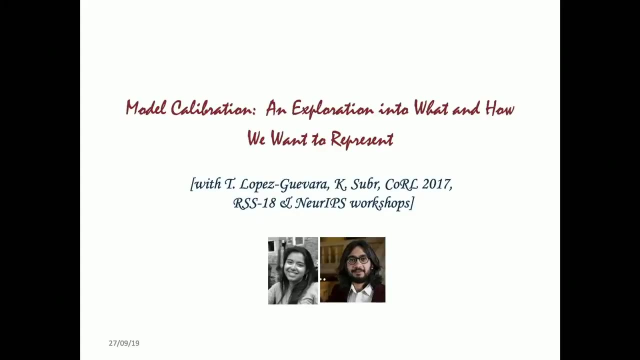 that actually can be brought to bear on this, if you can find clever ways of combining that with more modern neural network-based methods. That's what we are setting out to do. So, to start with, as a preamble, I'll show you a glimpse of results. 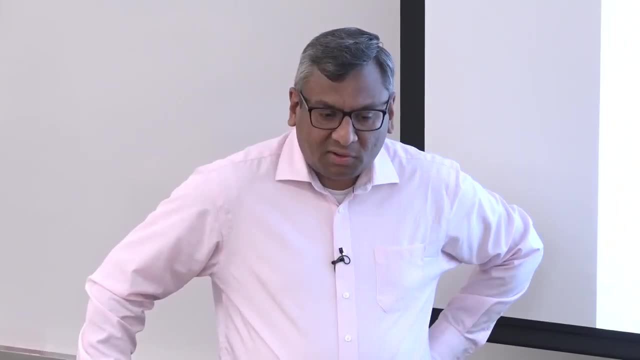 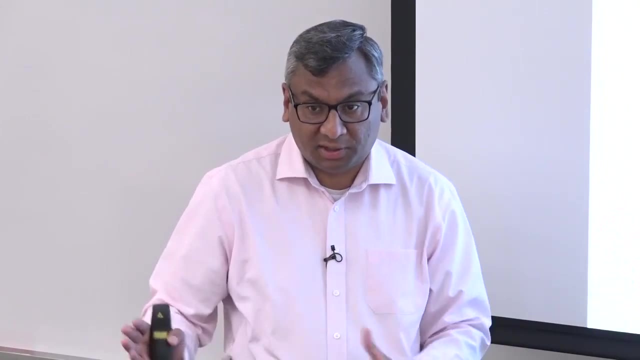 from an earlier project that get to this question of what do you want from models. What do we mean by models? Because the word is so overloaded that it means literally different things to different people. If I spoke to a statistician, all they mean is a description of a distribution. 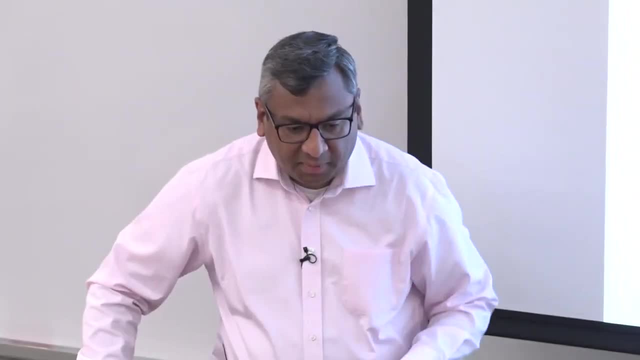 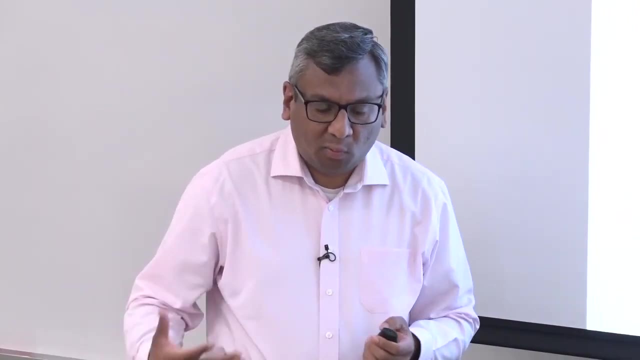 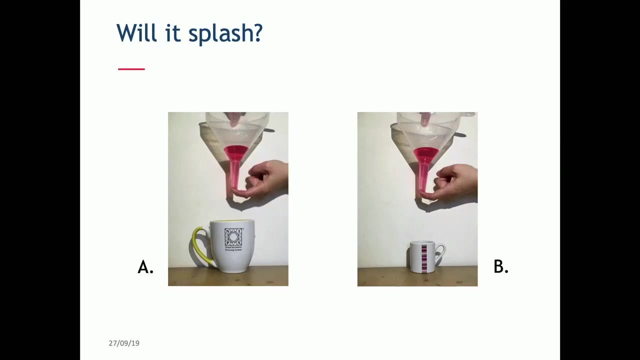 Gaussian is a model, Then if I speak to engineers, they might talk about a complete system. So what exactly do we want to describe in terms of models? I thought the way I could get that across is to talk about a task that we played. 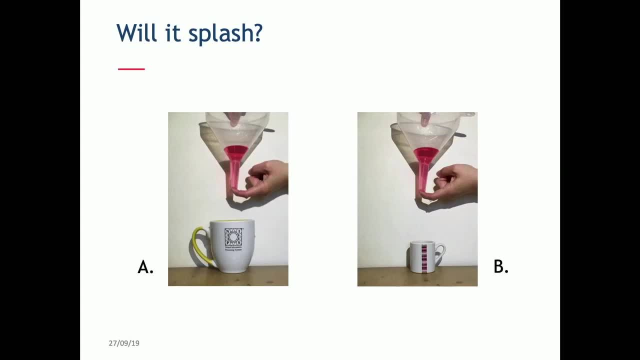 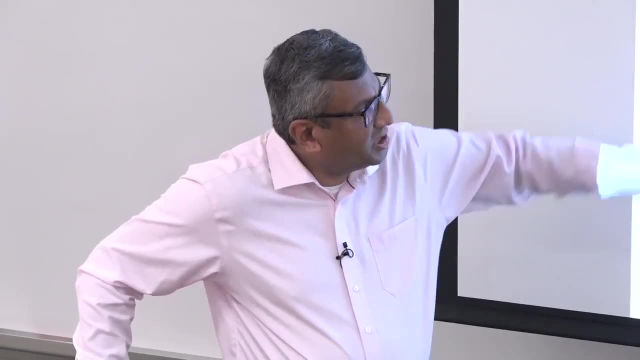 around with our robots. that's inspired by what people might try to do. So imagine a situation like this: You have possibly a number of different types of liquids that are filled into those funnels, and we're asking the question if the finger was taken out and 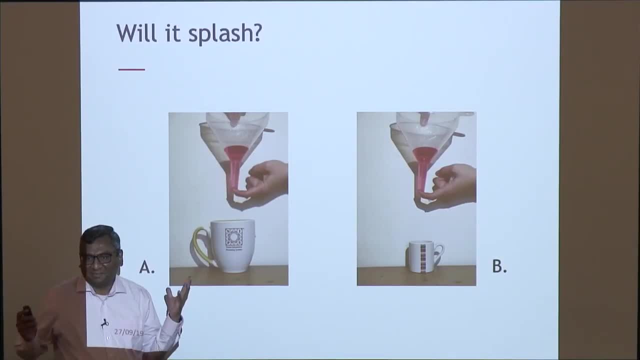 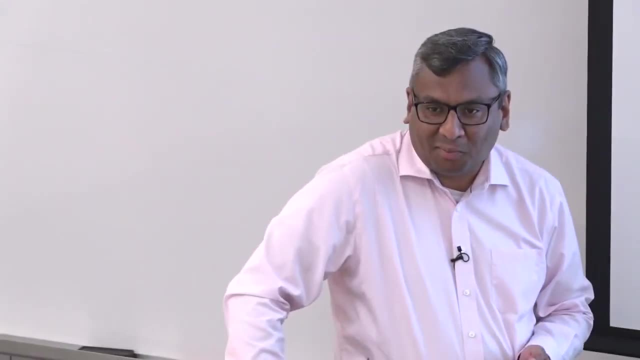 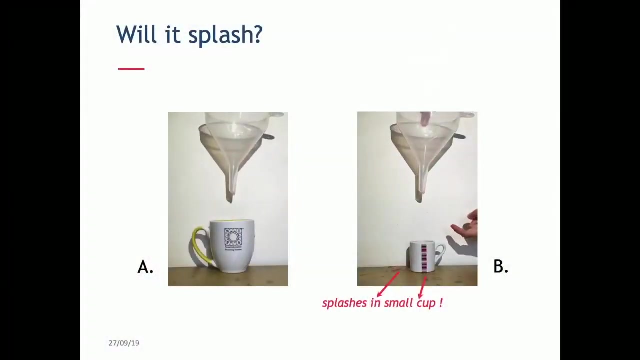 the liquid were allowed to fall into the cup, will it splash? So it's a straightforward question. It's the kind of question that is so intuitive that you could imagine asking small children and they would give you perfectly sensible answers. So here's what would happen. 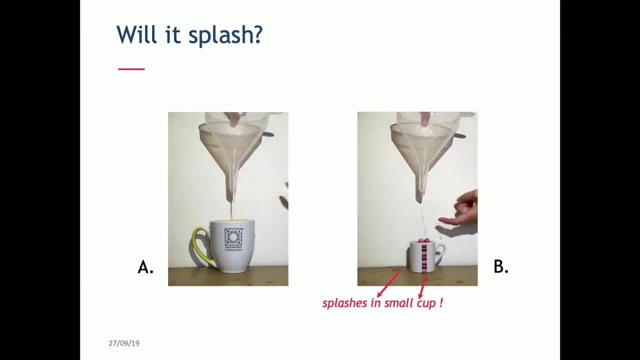 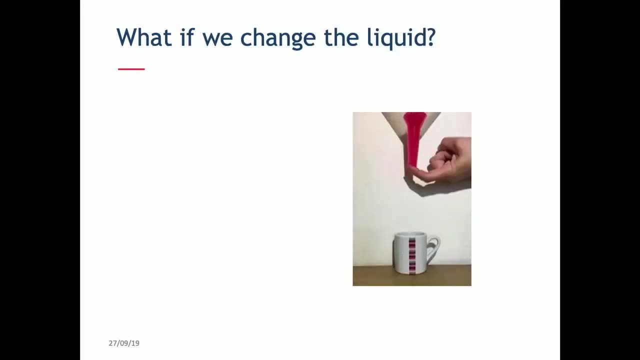 It depends on the size of the cup. It splashes a little bit if the cup is too small. If you have a giant container, then it doesn't splash. We all know this and this would have been your intuition. Now, if I tell you that I have a different kind of liquid, 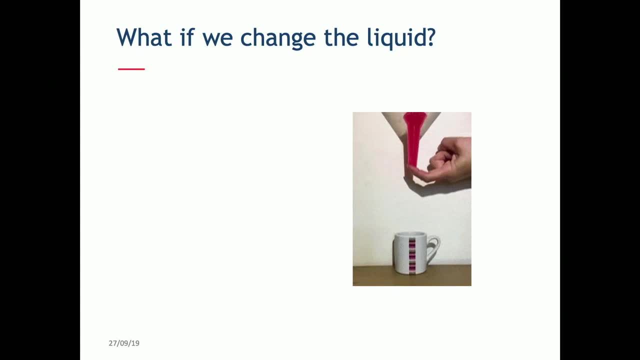 maybe the viscosity has changed. is it going to splash In your head? you have some reasoning that says, well, it depends on what the viscosity is and so what you might do, especially if you're allowed to think about it a little bit. 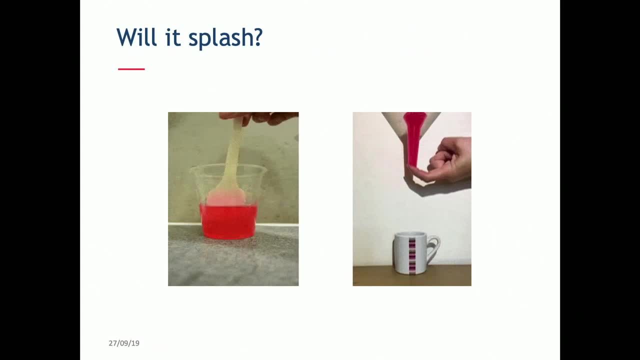 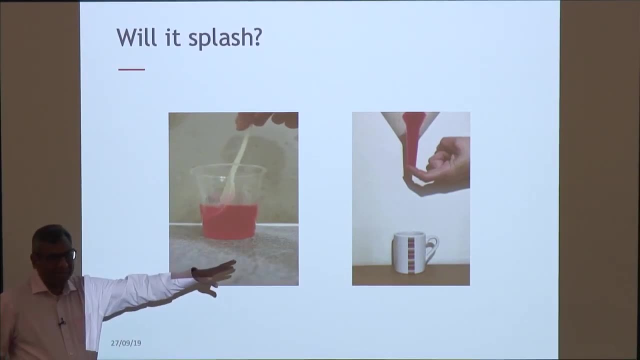 is either simulate or perform some kind of an experiment like this. that says the last time I played with this liquid. if it behaved like that and if it was thick and sticky, then most likely it won't splash. If it was loose and free to flow. 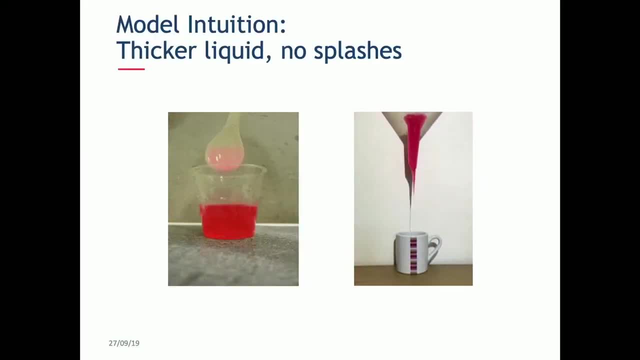 then it would splash. So this is what happens: because such a thick liquid doesn't splash, it actually cleanly stays inside. Okay, This is a kind of reasoning you have to do if you want to do planning for the things I'm talking about. 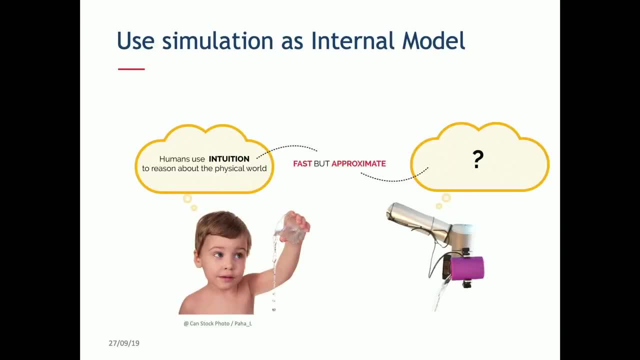 Okay, So how does this reasoning actually happen? So the claim here is actually that you have to have some models. At the very least, you have to have some level of intuition and common sense models. This is a claim that has been advanced very 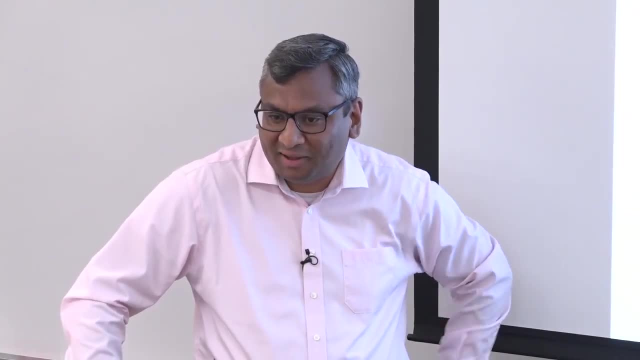 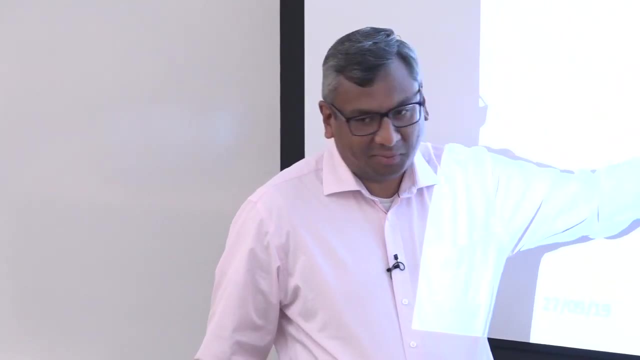 effectively by groups such as by Josh Tenenbaum at MIT. In fact, those examples are inspired by things I've seen him say. I'm not really going into exactly what is inside the brain of the human. I'm more asking what would be effective ways for. 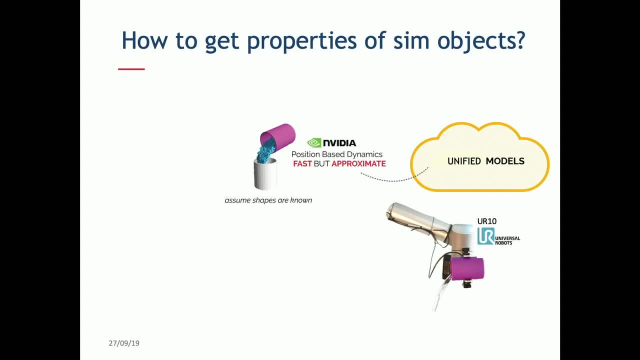 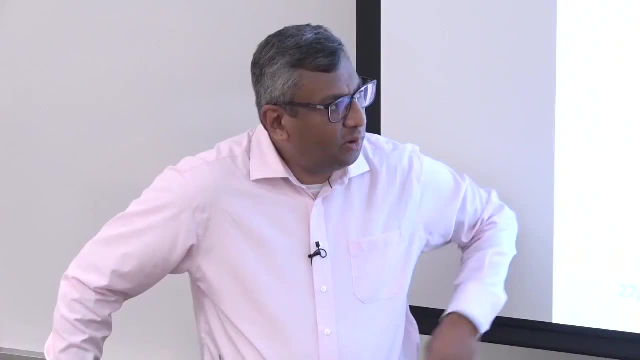 engineers to acknowledge this and somehow do things. So in this particular experiment, what we did was to say: okay, so we're going to build up some kinds of models. So in our case, the model was in the form of a simulator. 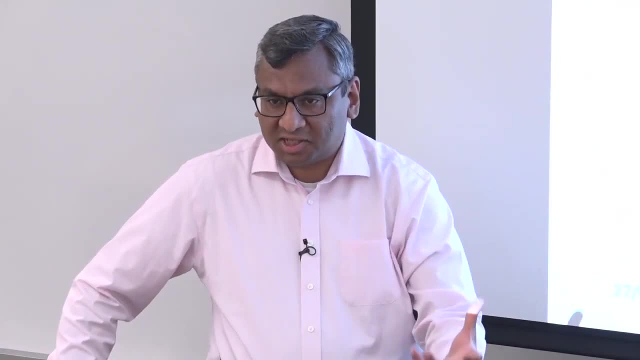 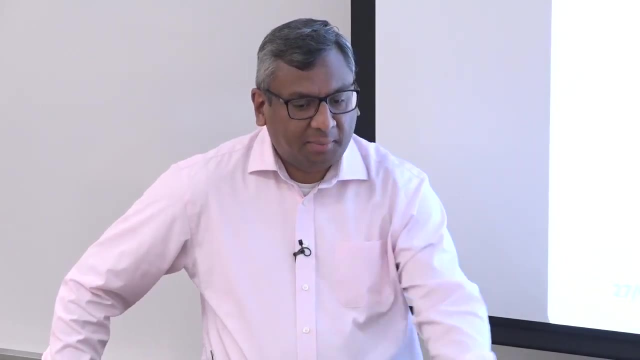 and the simulator had certain parameters about this task that had been given, such as the shape of the object, descriptions of the fluid. Then what we wanted to do was to calibrate that simulator to reality and then, having calibrated that, use that in a planning process. 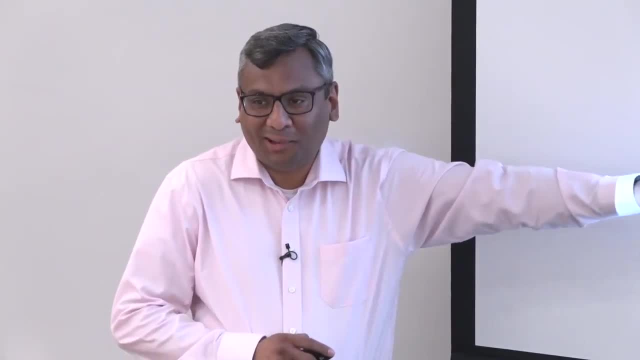 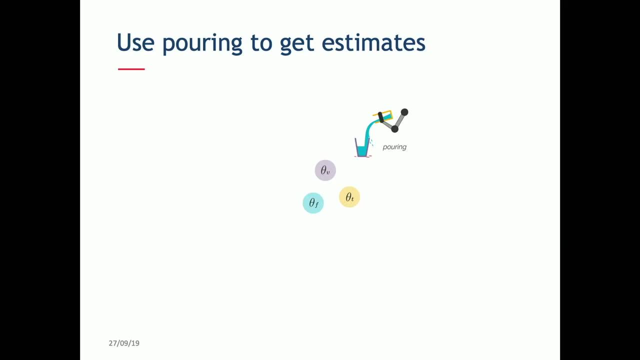 Because this is not the core focus of my talk. I won't take you to the details of this method. I just want to give you a glimpse for what I want to capture in a model. So the first thing you notice is that when you're thinking about what 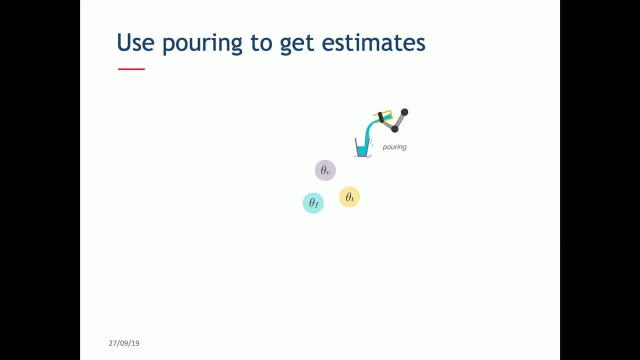 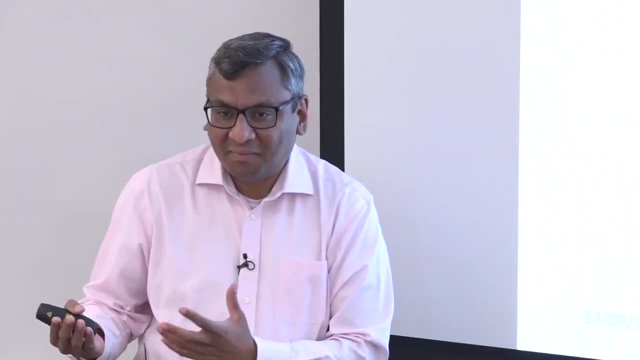 the simulator should encompass and what you want to represent about it. you realize that the properties you want to get right depend on what the task is. If you want to worry about whether it's going to splash or not, it depends a lot on viscosity. 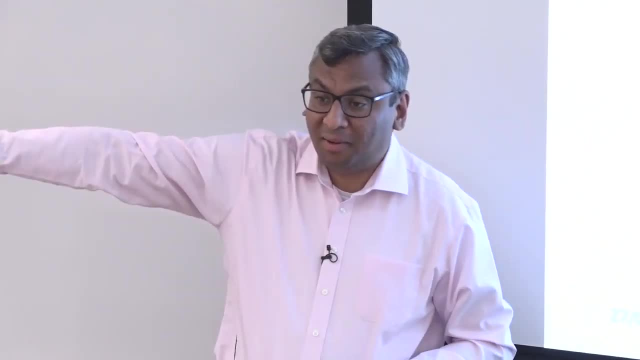 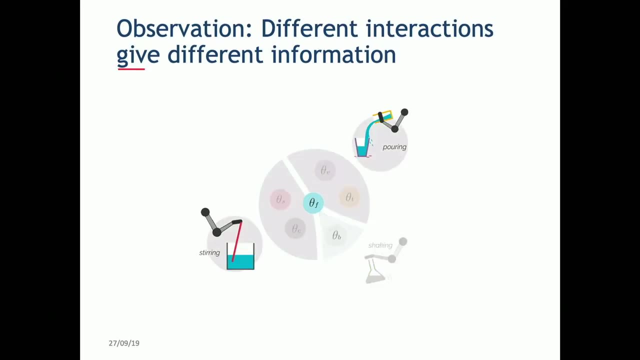 If you wanted to represent something about its visual appearance, maybe it depends on something completely different, like surface tension. You also realize that different tasks have possibly things in common, such as my observation that you can first stir and find out and then use it for pouring. 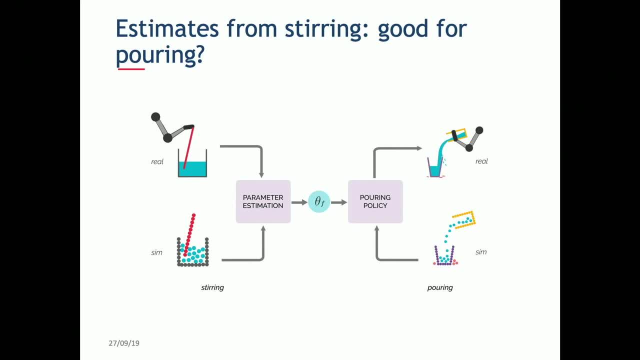 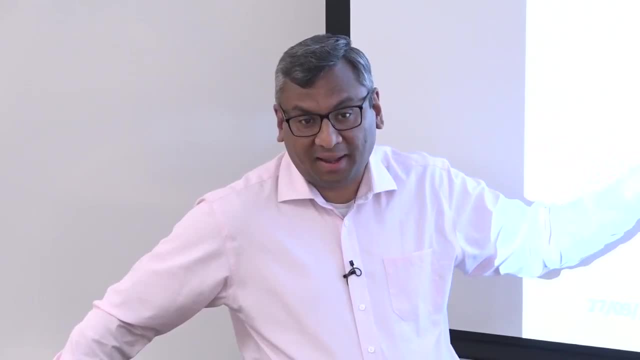 That's exactly what we did in our experiment is that we were looking at ways in which you could do parameter estimation with one task and then transfer to another task. So this is now a fundamentally deep kind of transfer, and that I don't just mean when you change the viscosity of this. 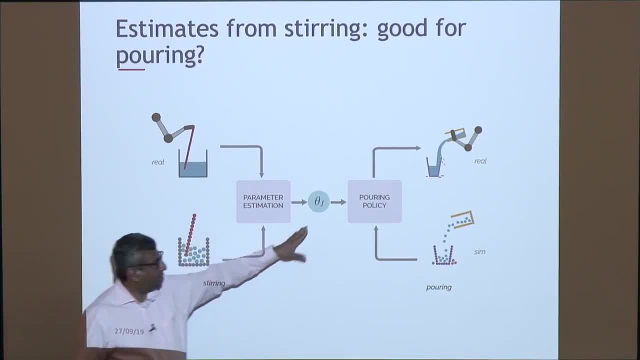 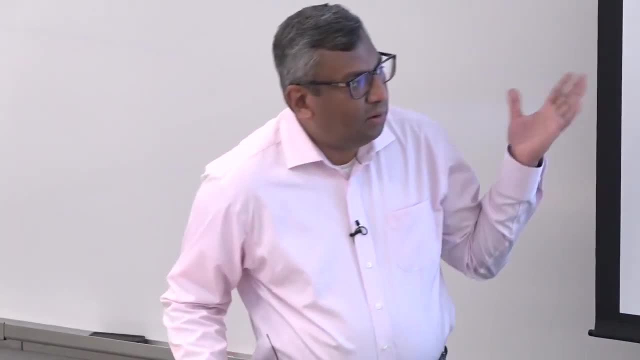 still stir in a certain way. I mean, use this to figure out something underpinning which then informs how you do a completely different task. To an engineer, this kind of a diagram would just seem obvious. Yes, this is what you do. 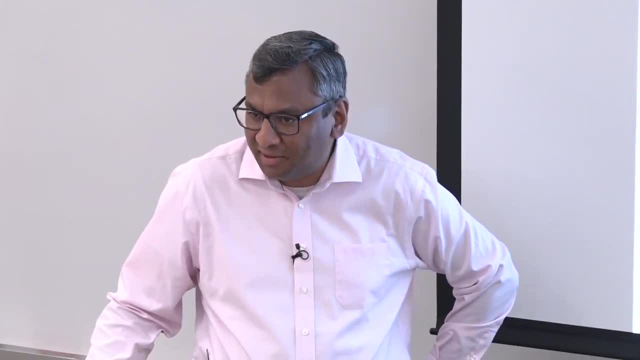 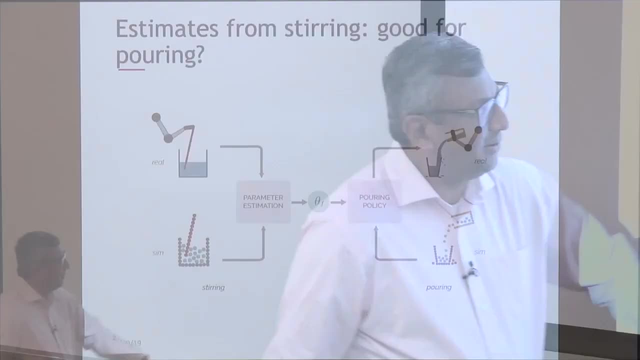 I think most humans behave like this and cognitive scientists would agree. But somehow in the robot learning community, especially when you think about machine learning, there's a lot of controversy about what you want about this. so the claim I'm stating upfront is that to me. 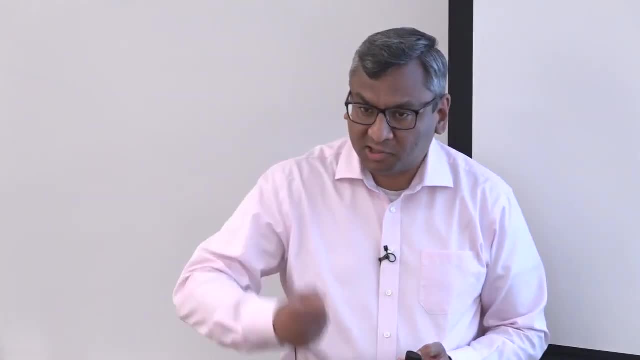 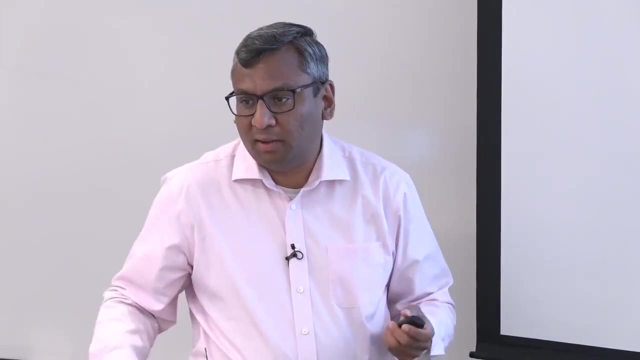 the utility of having good models that somehow capture structure in a deep way is the possibility that it allows this level of generalization and reasoning, and that's why we would like to have them. Then we're trying to ask how we want to marry that with other things. 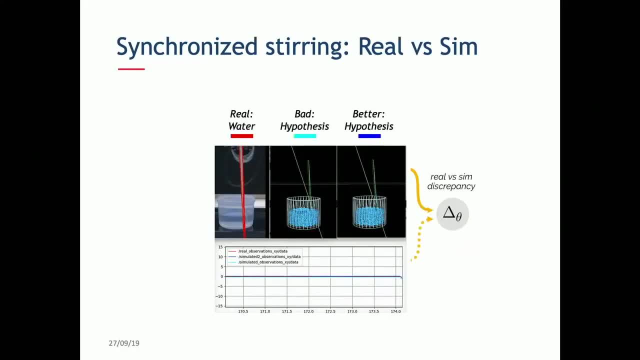 So, for instance, the way in which we actually did this is that we took actual data from how people are stirring liquids, we looked at the realized behavior in a number of different simulators and then we perform a Bayesian optimization loop to figure out what the best parameters are. 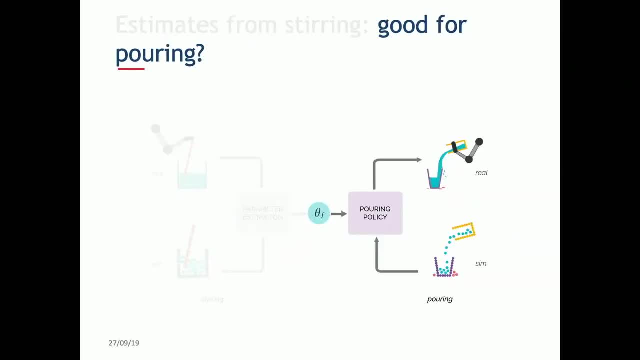 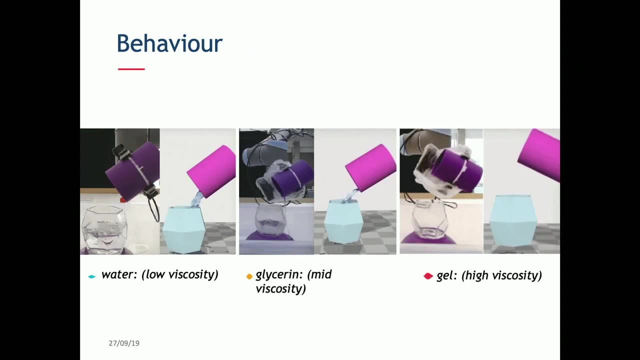 There's one example of how you might reason about a model, and then that allows us to optimize pouring policies. Good question: Yeah, That theta F now limits the kind of transfer that you can, also Absolutely Yeah, So that's important. 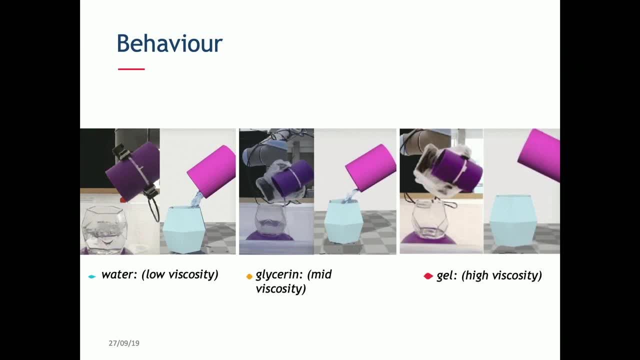 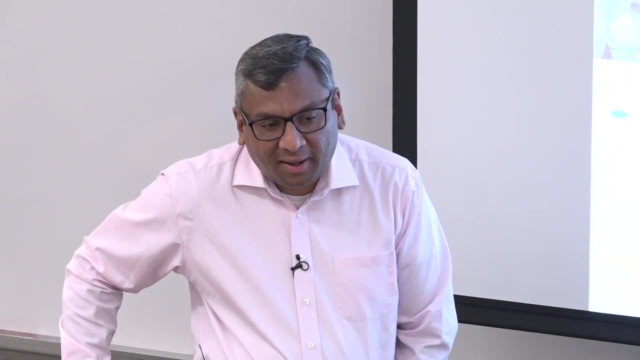 Yeah, So this is exactly the point. is that, just like historically in engineering, you would have had 10 years of debate about what are good parameters? I think that the point I'm saying is there's no getting away from some of that thinking. 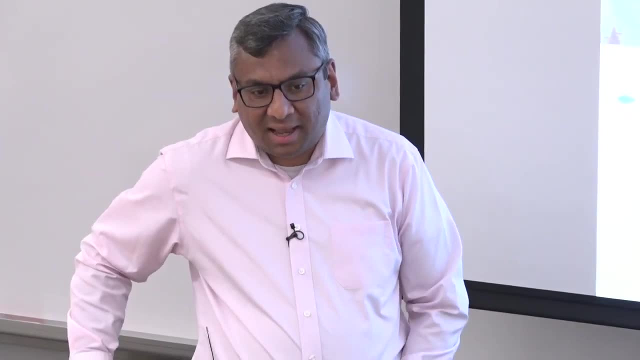 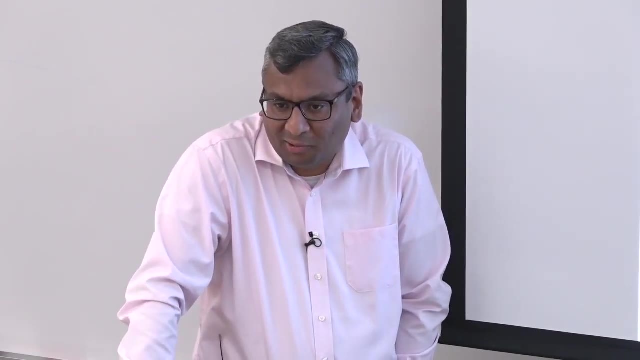 you have to do that thinking. The question is, can you find theta Fs that are coarse enough that you say just enough of what you want to say and then let the model do the rest of it? So it's in that balance. So here what we're showing, 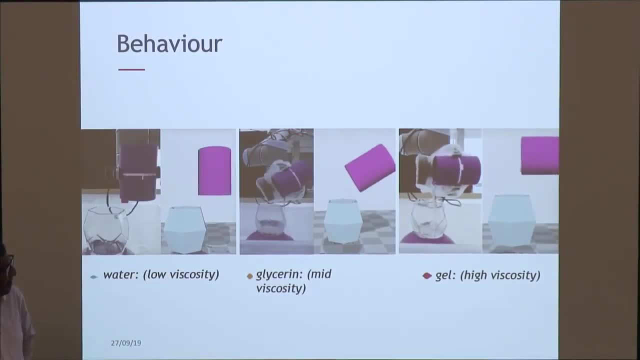 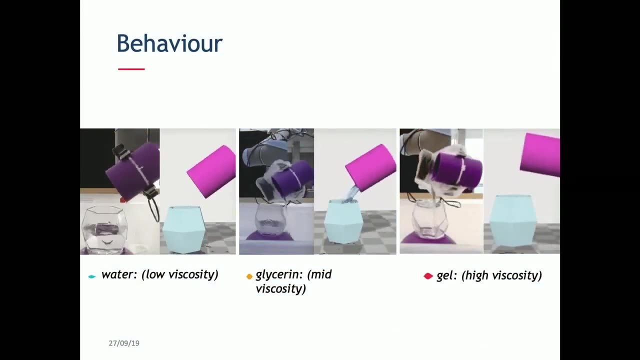 and this is all. the left side of each of these is something in our lab. is the robot, having figured out these kinds of properties, how it figures out how to pour in the most effective way with the least amount of splashing, with this being its internal representation? 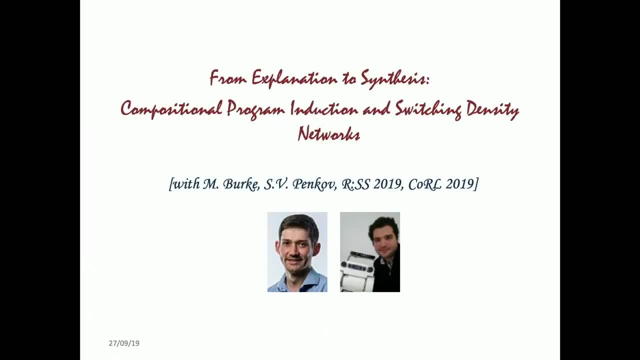 Yeah, So that's what- yeah, go on. Can you give a bit more details about that internal simulator? I'm trying to get a sense for what was the parameter space? How was that simulator? So it really is just an NVIDIA Flex simulator. 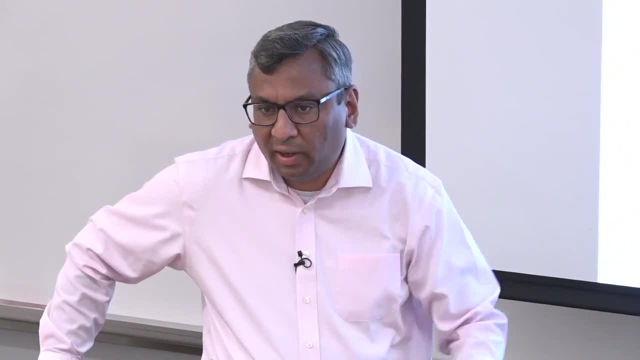 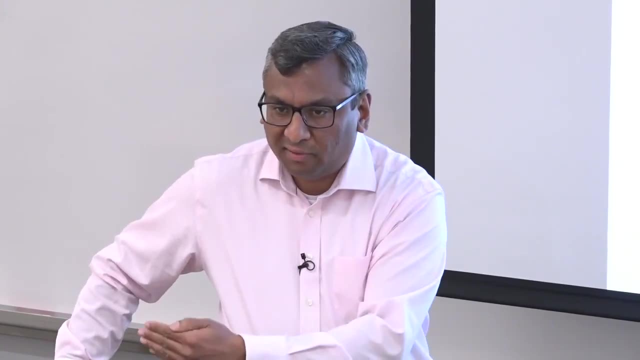 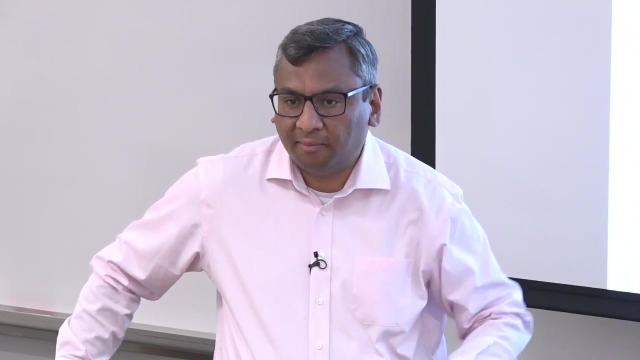 with a kind of particle-based approximation to the fluid. In that interface we are given high-level parameters that correspond to all the fluid dynamics parameters. So viscosity is an example. So what we are really playing with. there was viscosity, So how high-dimensional was that Bayesian optimization landscape? 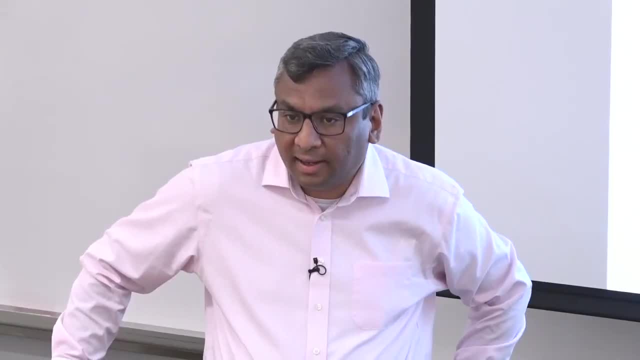 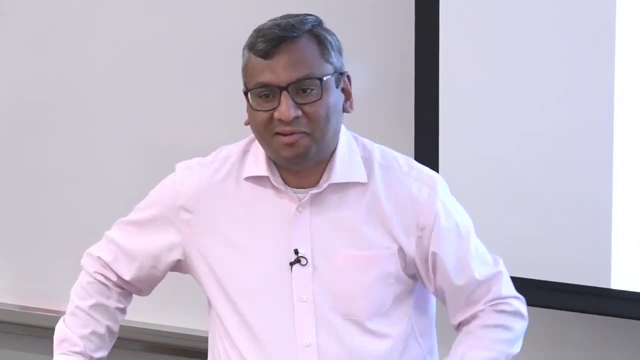 It wasn't very, because we were only searching over that low-dimensional space of parameters. It could get high-dimensional if you want to explore with a lot. Actually, when I get to my main result, which is what I'm talking about next, I'll tell you a little bit about this dimensionality question. 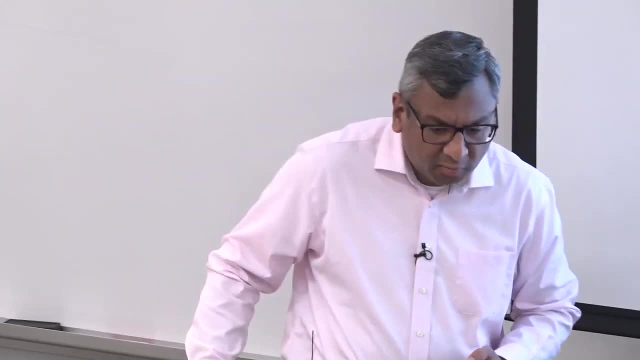 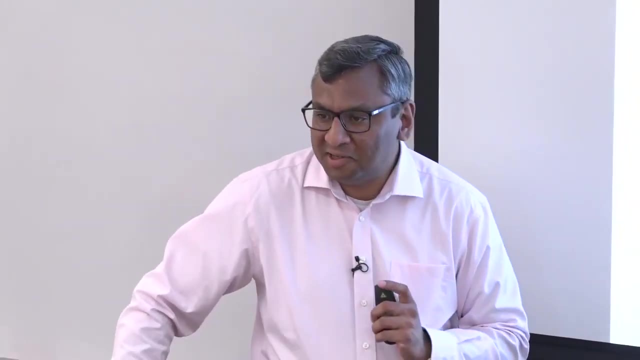 So that whole preamble was to give you a flavor, for kind of shake you up a little bit and say: think about models in this way. So models are not just things that are hyperparameters in a network, but there actually is more to it from the physical point of view. 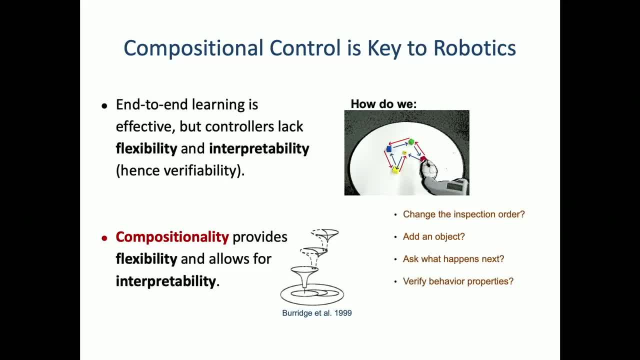 Now I want to take you a little bit more into kind of robotics-specific things. So in the robotics community we've been talking about these kinds of representational issues for very, very long time. So in fact my PhD thesis work was on learning to walk. 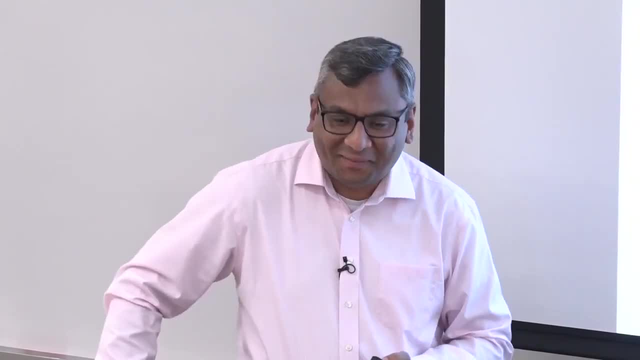 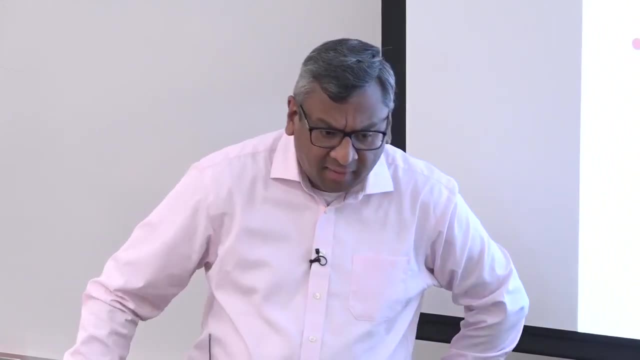 Before we had things like atlas, so it was still a worthy question for a single, solitary PhD person to ask. So I was looking at things like learning to walk, and there's been some very, very elegant work that's been done by people like 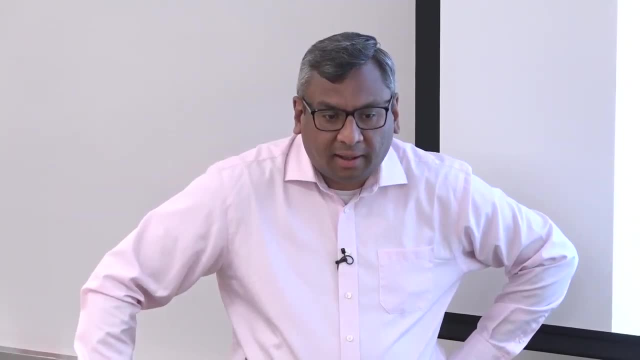 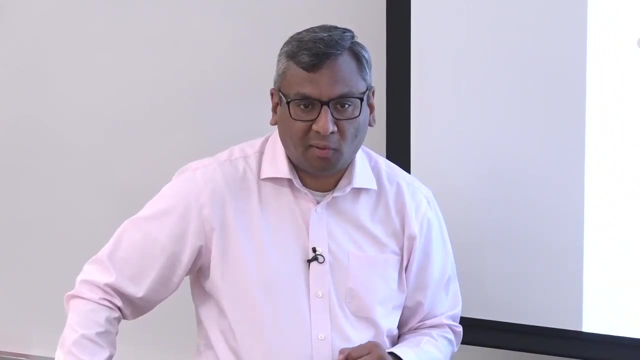 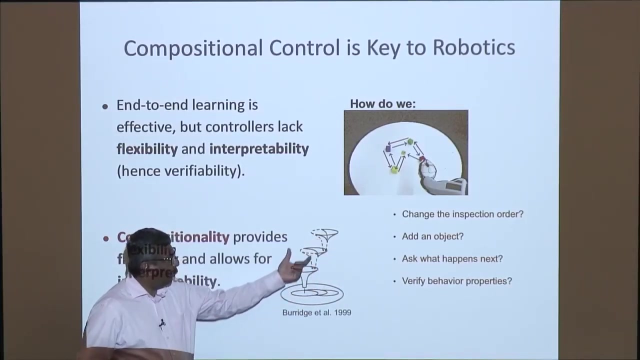 Dan Kodacek and collaborators, who showed that a good way to construct controllers and a good way to describe biological behaviors of the same control phenomenon is to think in terms of a hybrid control representation, something like this, where what this is depicting to you is the movement from: 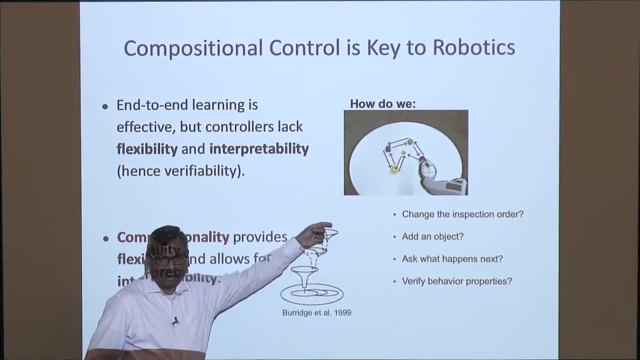 an initial state space to a final set of states over time. So time flows from top to bottom. So if I initialize the system anywhere in a large state space and I run the controller for some amount of time, then the controller ends up in a small set of states. 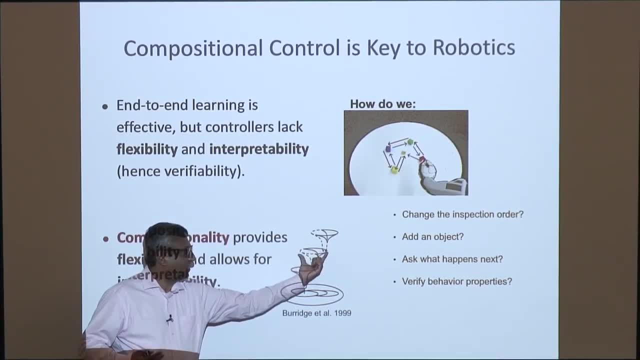 That's what controllers do. Then that small set of states sets me up in the next one and next one. So you can think about what a large task compositionally in terms of a smaller set of this, where the representational question, the equivalent of picking the Theta F, becomes what funnel? 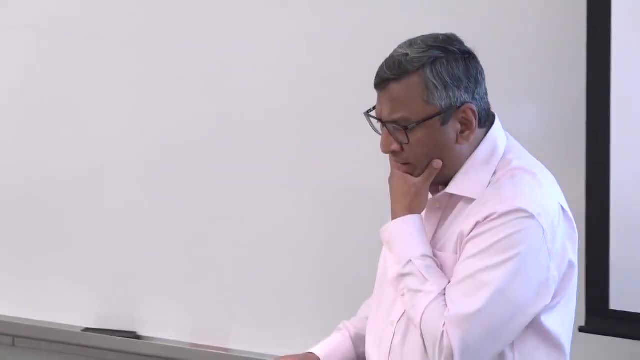 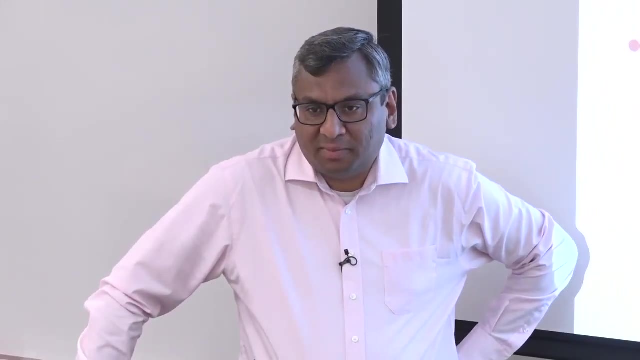 what shape, what switching logic, and so on and so forth. This constrains you, but it constrains you in just about the same way as picking a basis function in function approximation, in that, yes, you're making a choice, but then the choice allows you to do quite a bit. 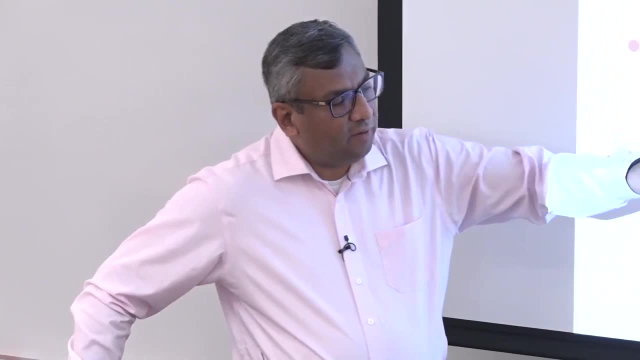 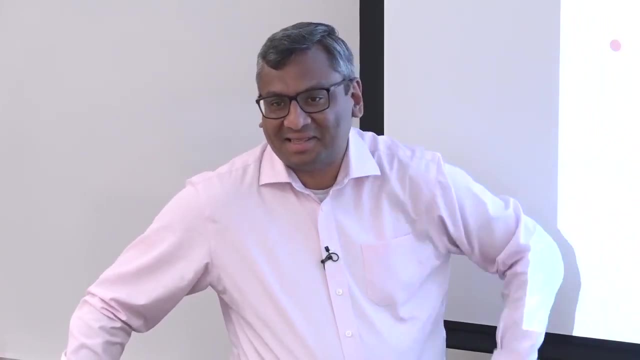 So what we are trying to ask is to the extent that when people have handcrafted controllers- and in fact today, if you look at Atlas doing its backflip- it still is doing that. It's the same first author in the same company. 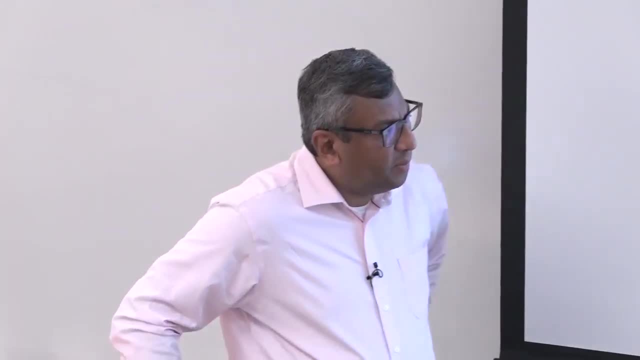 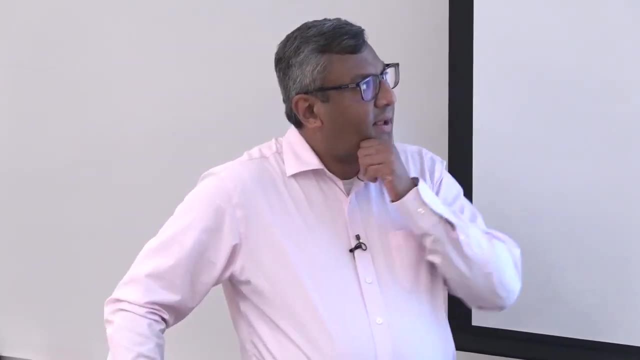 So when you have these kinds of representations that are working well for people, can we somehow use that inside a learning model, and would that give us any real leverage? So we are interested in having flexibility in the sense of being able to answer questions like this. 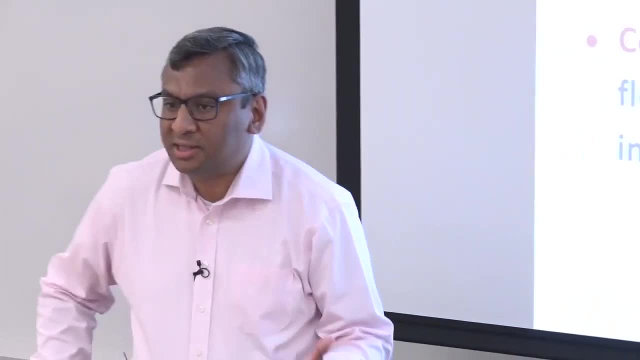 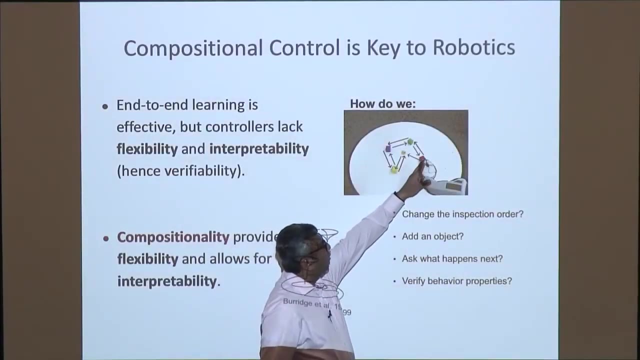 which I would claim would be hard for us to answer unless we had some kind of structure. So if you want to ask a question like so, in this case the task for the robot is to go from one object to the next in a sequence. 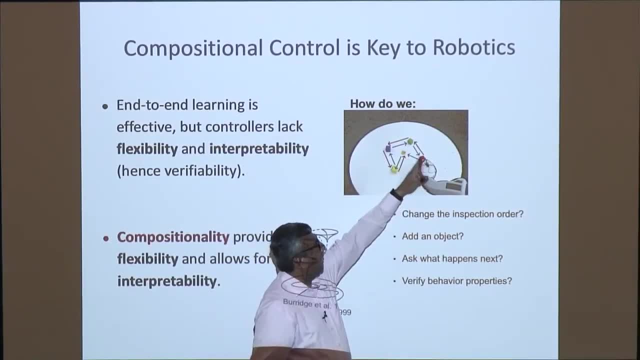 and if it hits a certain kind of object it should flip around. So it goes A, B, C, D, E, and if it hits E it should go back around, and then it just does this in an infinite loop. 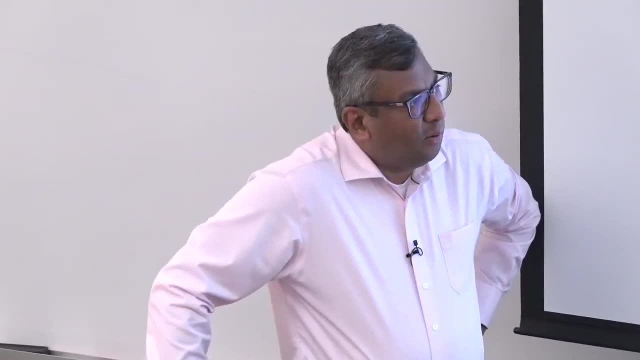 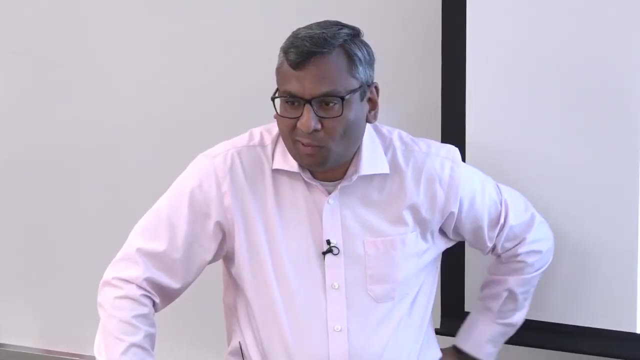 It's a trivial program you could write If I wanted to ask a question like: what would happen if I move my objects around? What would happen if I insert a new object? What would happen if I wanted to ask: will this ever terminate? 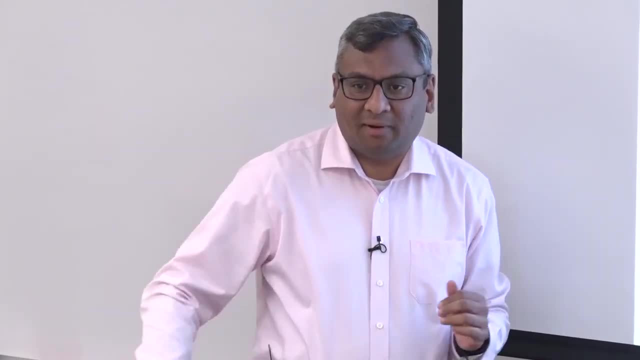 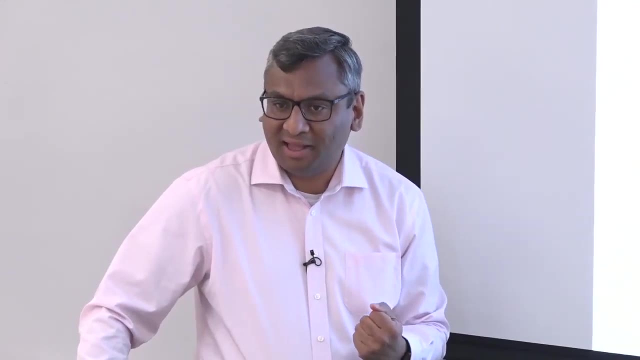 Things that a regular engineer I would just ask. naturally, There's simply no way to answer such questions if you leave everything implicit. So you have to somehow elicit the structure so that you can reason about it a little bit. What we are arguing is that if you're sensible about your choice of controller structure, 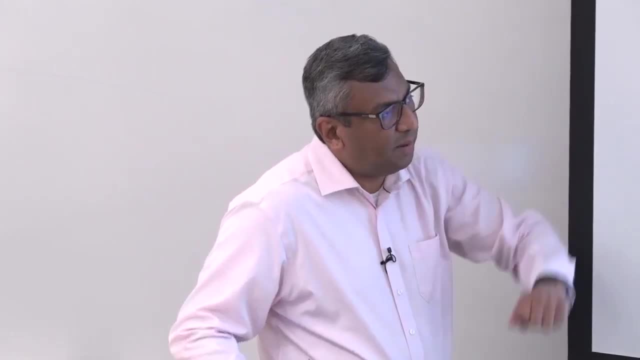 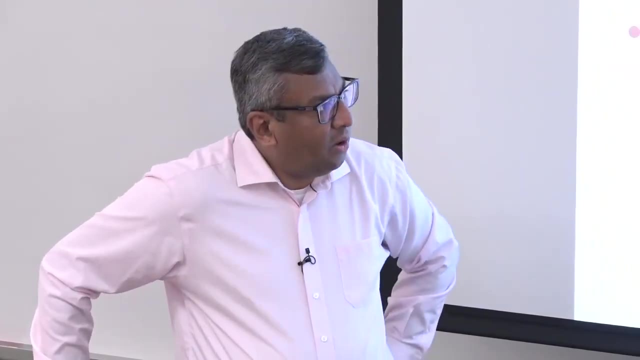 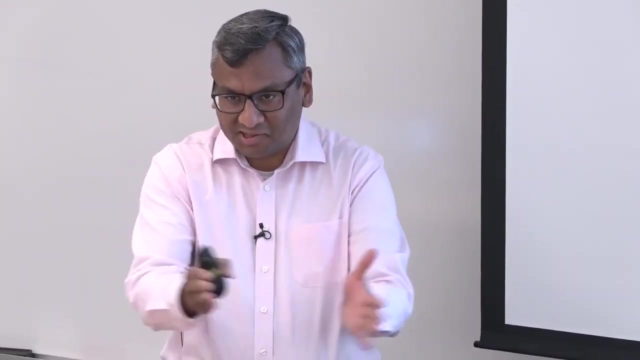 there are ways of marrying this. So, with respect to that particular inspection task that we cooked up, it's a tabletop inspection task with a collection of objects. What we want to see is: is it possible for us to go from a human demonstrating this task, not actually telling us what the task is? 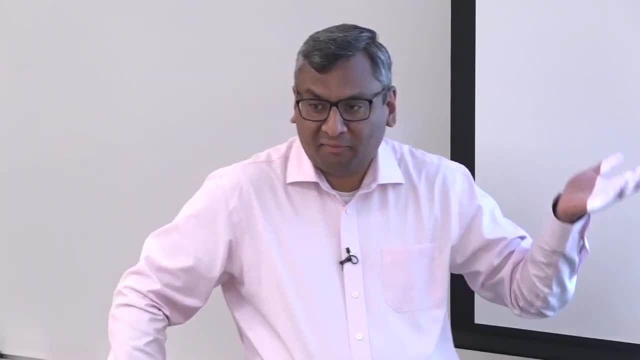 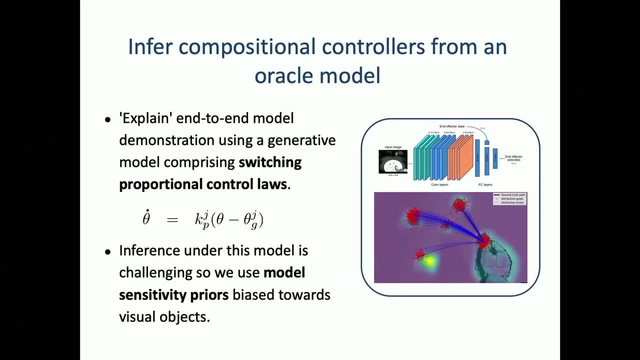 just demonstrating it and is it possible for us to do system identification of this full structure, including the low-level controller and the high-level switching logic. So here's how we go about it. So we actually exploit the neural network models where they are strong. 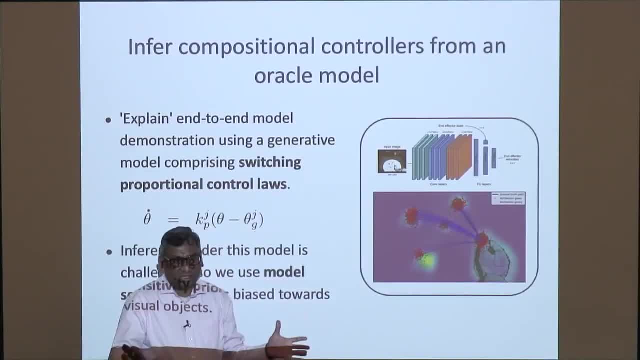 which is to make local predictions about. in that whole sequence I have 1,700 or so frames in a typical demonstration. If I gave you the input image, could you tell me what would happen? What would happen next? I just want to make local predictions from pairs of images and next, velocities. 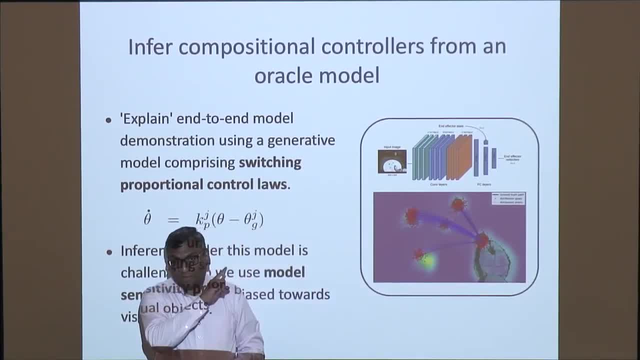 This network is not powerful enough to represent that whole program that I showed you because it doesn't have memory, can't represent the logic, but it's good enough actually to make sort of decent local predictions. We use those local predictions to figure out what matters in the image. 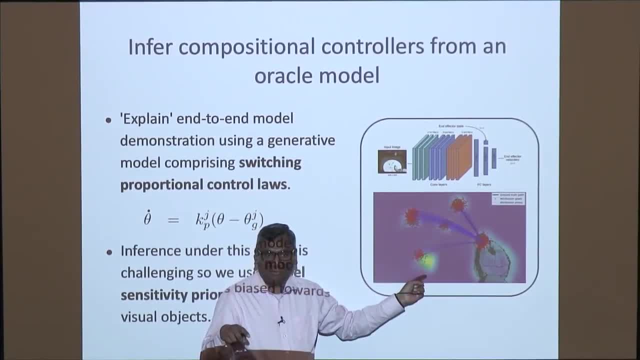 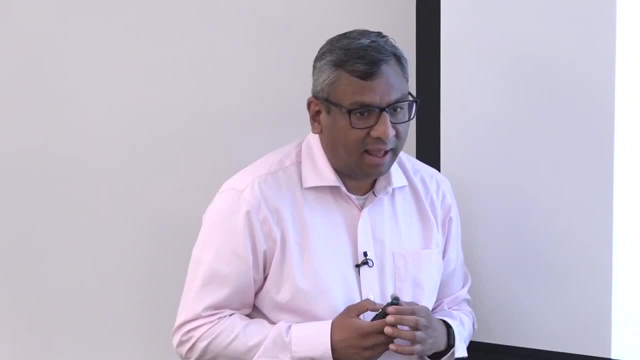 because nobody told us that there are objects in the image and where they are and all of these things. They were all left latent. We just have as a structural description that everything we want to describe can be thought of as some sequencing of local funnels. 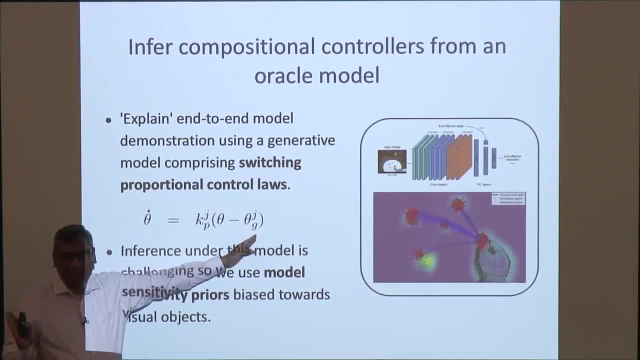 where the funnel is essentially just a proportional controller to a control theorist or a particular kind of parameterization of a function to a statistician. So we're saying our underlying task model is a collection of these switched together, I don't know with respect to what and to where. 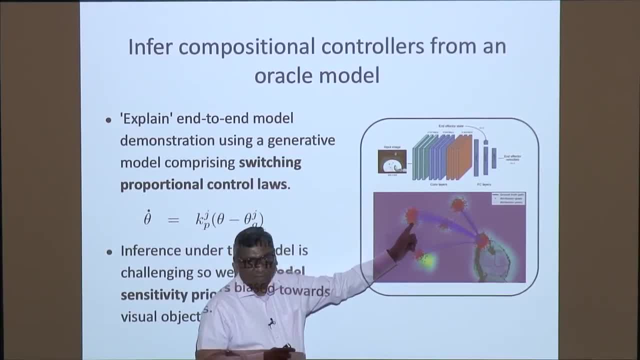 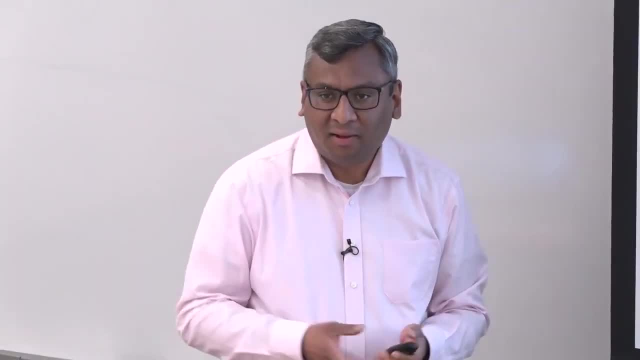 So we can pick that up by doing sensitivity analysis on a collection of this and then representing it in a sequential Monte Carlo fashion and trying to figure out what must be going on underneath. So I found out that these are all salient places by looking at the sensitivity of this network. 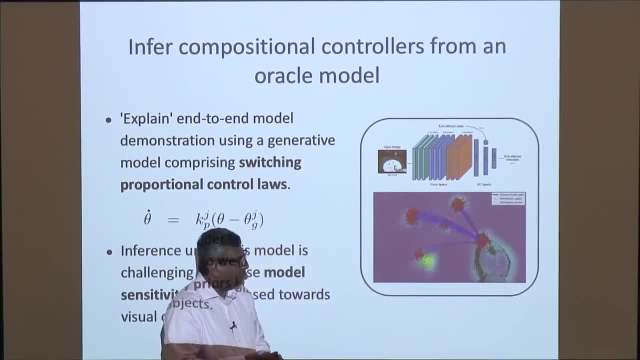 and then that gives me a collection of hypothesis, for if my robot is moving like this, is it moving here, is it moving here, is it moving there? and each blue line represents one parameterization, or something like this. So that's my task model. 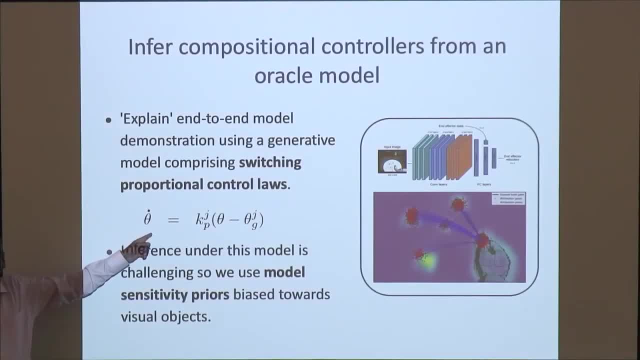 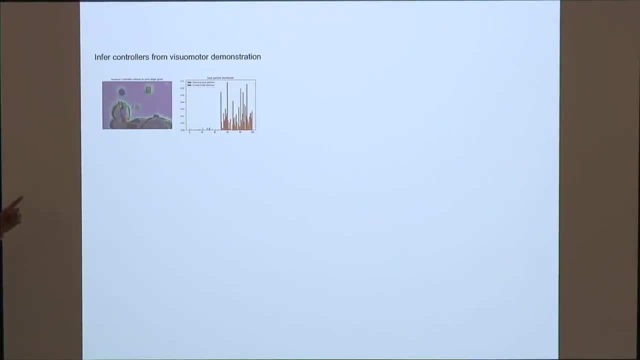 So I've put in structure, in the sense that I've told it that this is a useful basis. Beyond that, I'm letting the model learn for itself. So this is what it looks like. So here's a typical video of the demonstration. 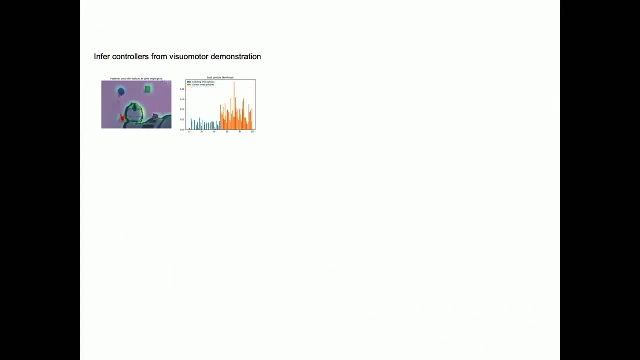 and what this is telling you is the number of controllers that are being picked up. You shouldn't really worry about this. What this is telling you is that, by looking at diversity of the controllers, if the predictions are sometimes here and sometimes here, then I know that that's a time to introduce switching. 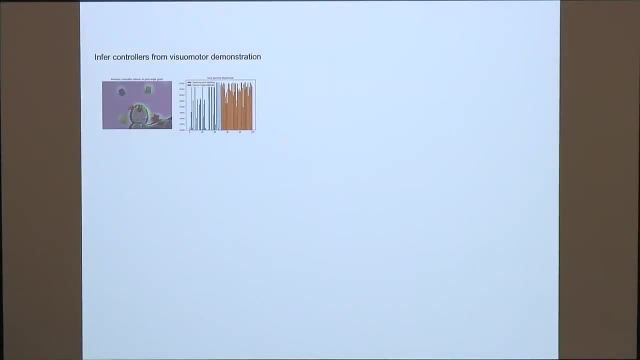 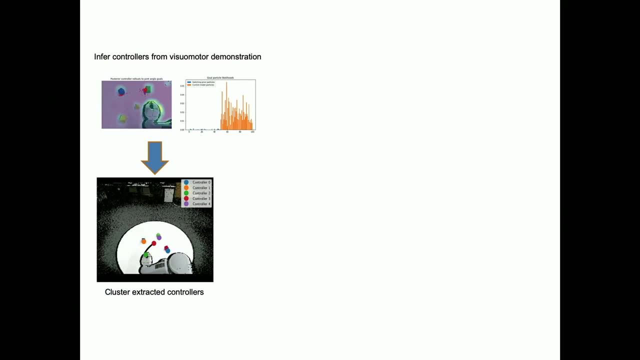 If all predictions line up, then actually I don't need to introduce switching. So from clustering those things, I actually get that in the underlying world there are that many objects and those objects are located here which I picked that up from that input. 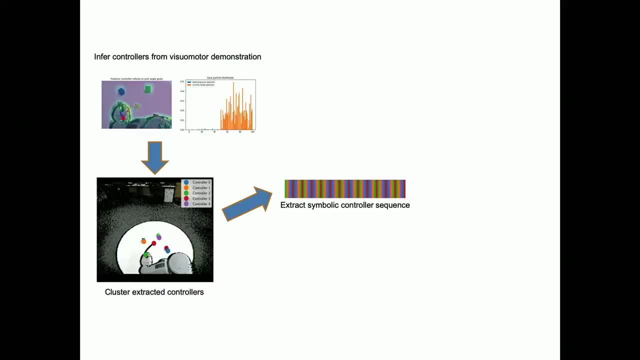 which I can reason about symbolically by saying: now there's only five objects in the world, So I'm looking at what is the sequence in which you visited those objects, which can be interpreted using your favorite string parsing or grammar learning kind of approach, to say that that's what the underlying task was. 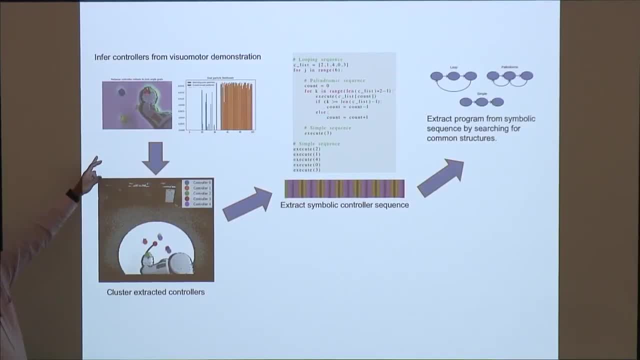 So we've gone from essentially just a video input of this, as the person is demonstrating, to a description that says: your task is to execute this sequence, where each sequence refers to one of those controllers. in my previous slide, Each sequence is a reach. 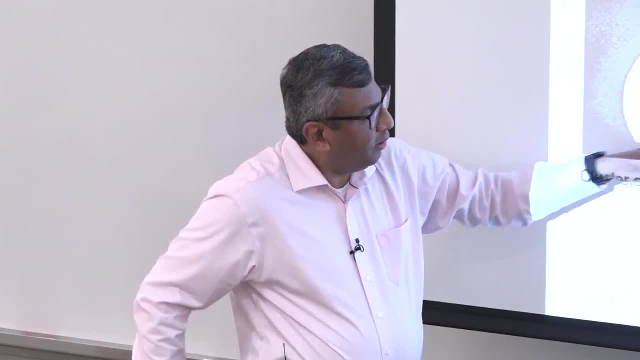 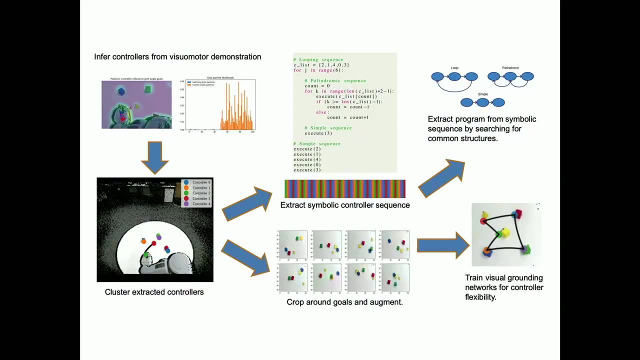 The one bit that I should say in all of this is that the original controllers learnt in terms of joint angles, So we train one more network that then grounds those joint angles into world coordinates, so that then this program that you've learnt can actually be. 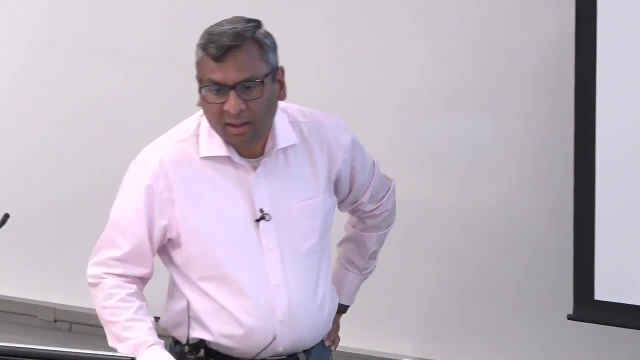 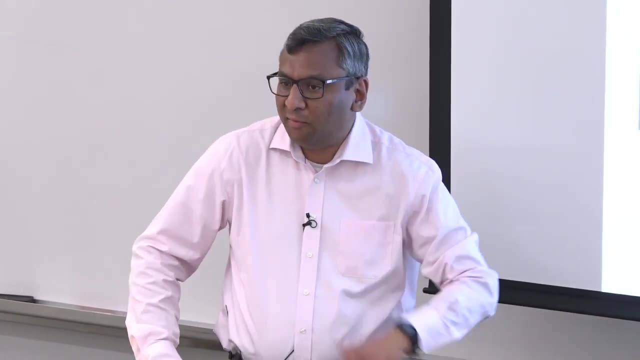 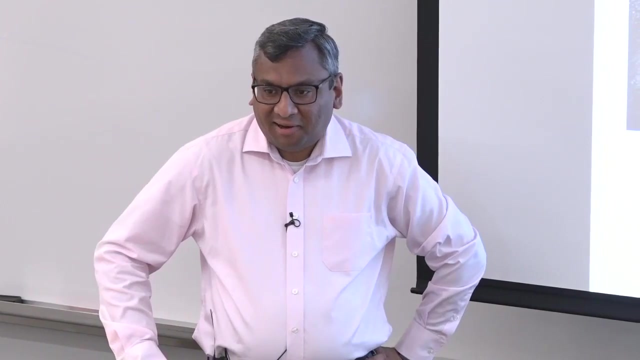 generalized to different orientations of objects. So here's a learning loop in which we have put in structure and our structure was specifically that this way of thinking in terms of sequencing of funnels is a useful description of control tasks. But then we've been able to be fairly general in all other ways. 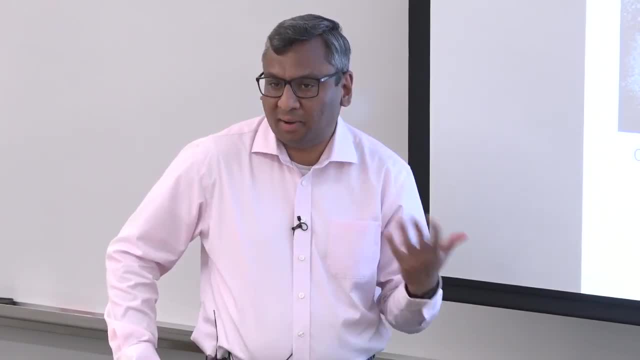 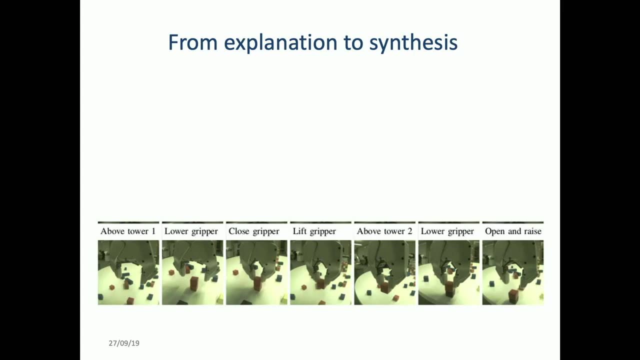 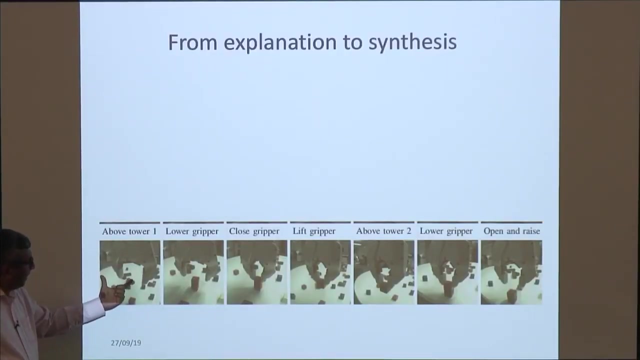 so that we can actually learn a switching control strategy from demonstration. Then we tried to extend this to a slightly more interesting task to us, which was to find ways in which you can pick up objects from a table and stack them up. So here are snippets of examples of 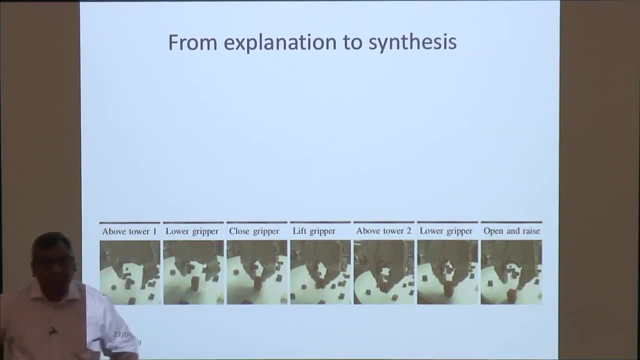 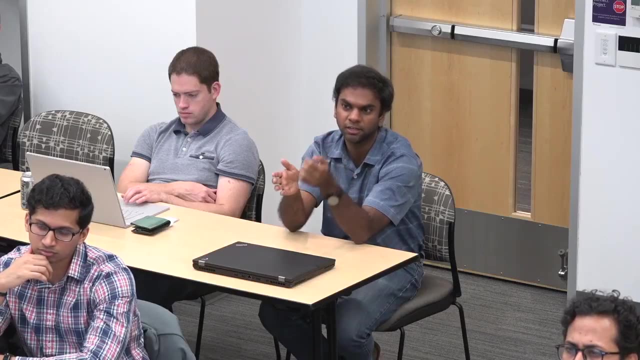 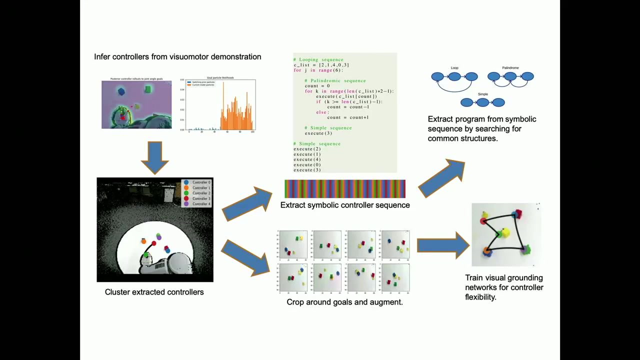 the vocabulary that we use to generate the demonstration In the previous slide. did you run into credit assignment kind of issues As in? if I'm learning this model, that's first time- to just predict, based on the visual scene, what's the action being taken. 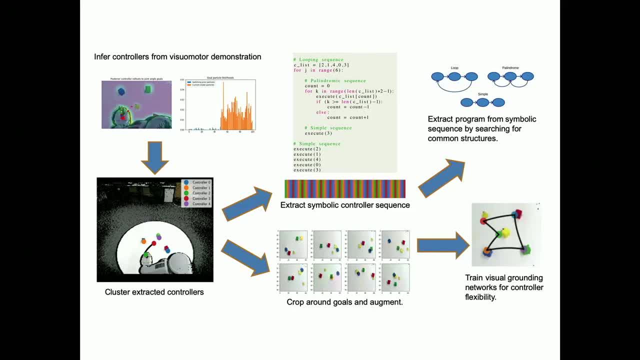 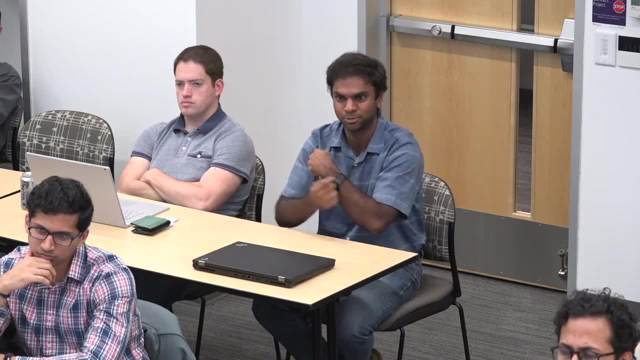 is the model bogus or is it the case that I've learned good models and I can trust its predictions, and the fact that it's getting confused and predicting two different things gives me an indication that I should be switching. So I would say that it comes down a little bit to. 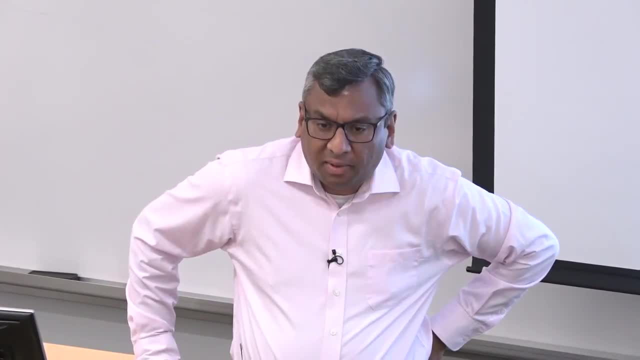 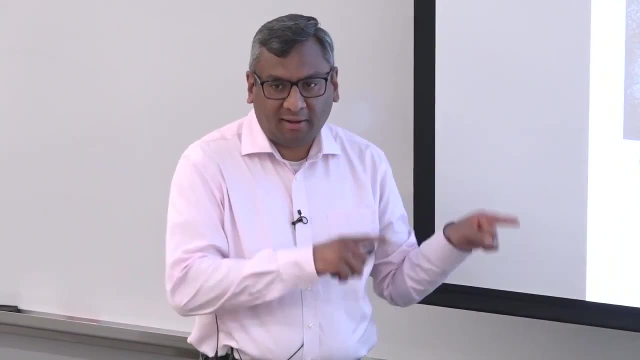 the same kind of thing as how you would think about a mixture model. So I'll come back to this question. So the short answer is, at this point in time, we are asking for a best description in terms of this vocabulary. Then what you're asking is: could there be two best descriptions? 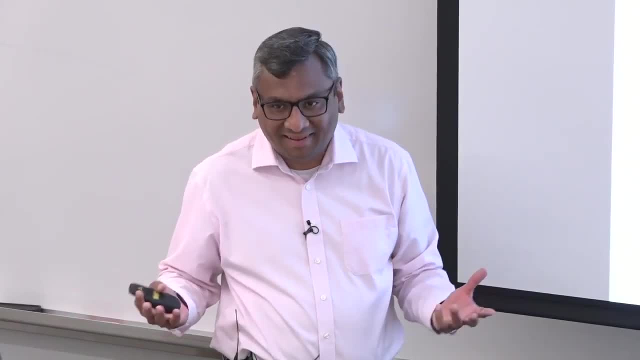 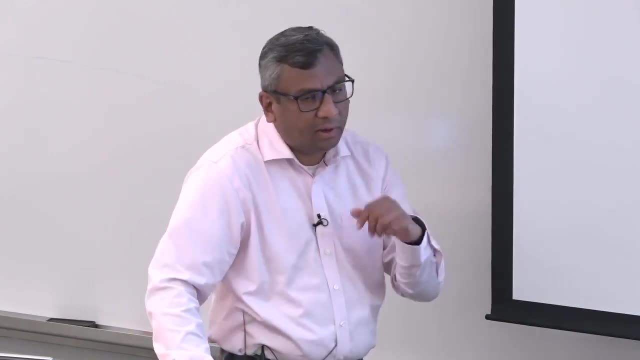 and you pick the slightly less interesting one. It could happen Then you would deal with it in the same way that you would deal with every other function fitting kind of paradigm. But I'll come back to it because I'll describe one more variation on this theme. 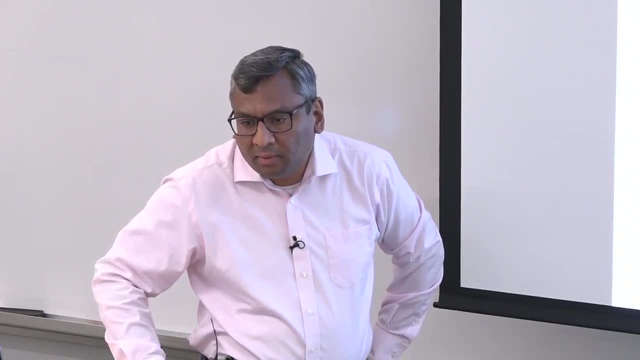 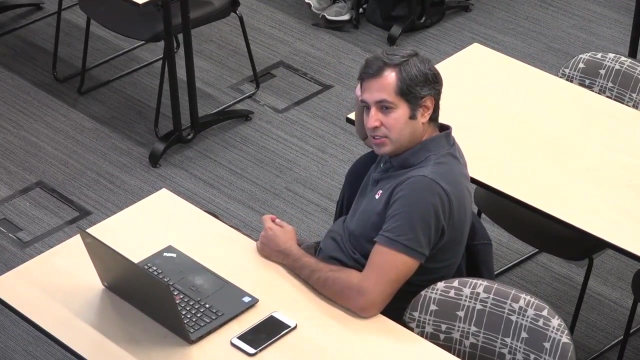 What would it take to extend this to hierarchical programs? So right now it's clustering, So you can write programs which are more like regular expressions. Yeah, But if I have infinite depth with compositions that are hierarchical, You have to find some way to chunk it. 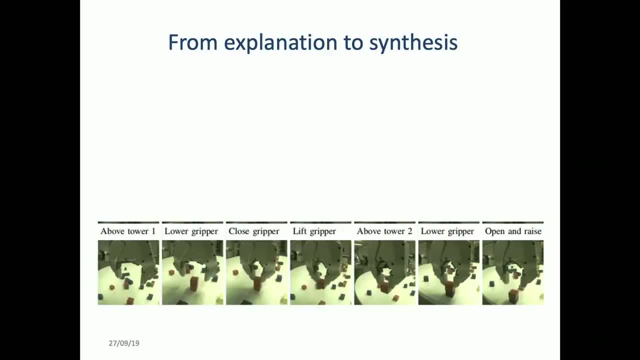 So let me go through one more section and then we'll discuss this point. Yeah, So it's actually leading up towards that. So the next task we looked at was hierarchical in the sense in that we wrote the program of how to demonstrate it using a vocabulary that looked like this: 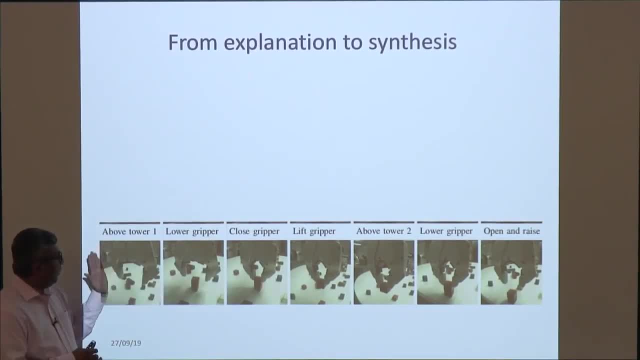 So we demonstrated to the robot that the way in which you stack is: you first go above the tower, you lower the gripper, you close it, blah, blah, blah. So this is what we told it and this was our internal hierarchy. 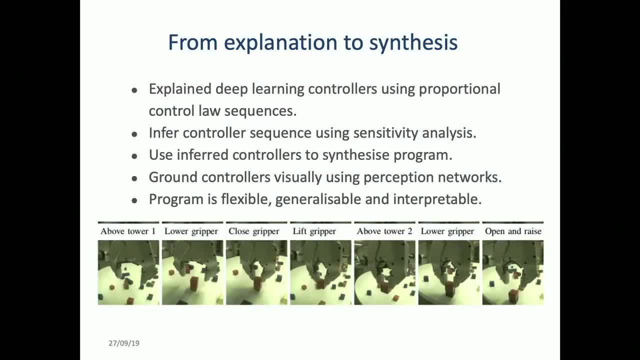 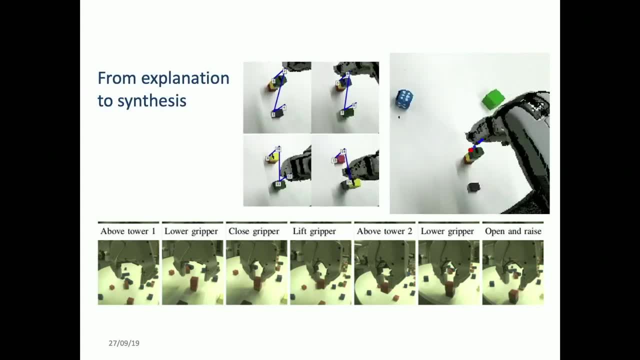 So we went through the exact same process that I'm telling you. So you start out with demonstrations, do the sensitivity, and then you ground them, and so on and so forth. Here's what the robot learned to do. So this was our input program. 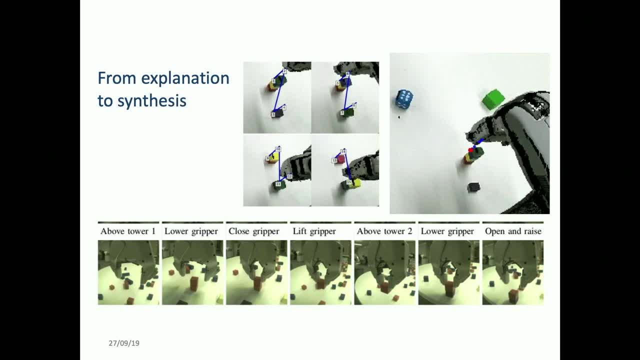 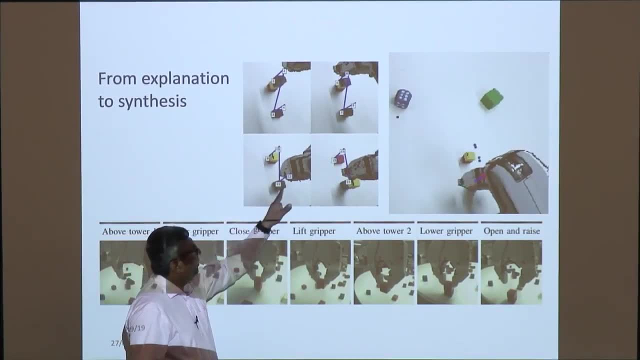 and what you see? there is a video and a depiction of the output that it has learned in its own internal representation. Really, what it does is it learns it in terms of these sequences, So it learns to put the sequences together, The bit that actually goes back to, I think. 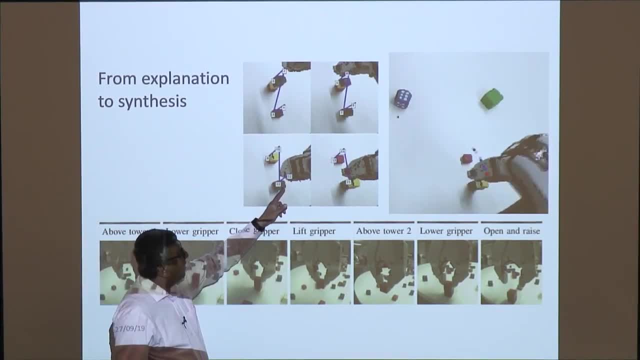 Sai's question is that actually the robot is not smart enough to figure out that this sequence is the same as this sequence. You still have to do some program simplification and things like that afterwards. So it says: this is one thing, this is one thing, that's one thing. 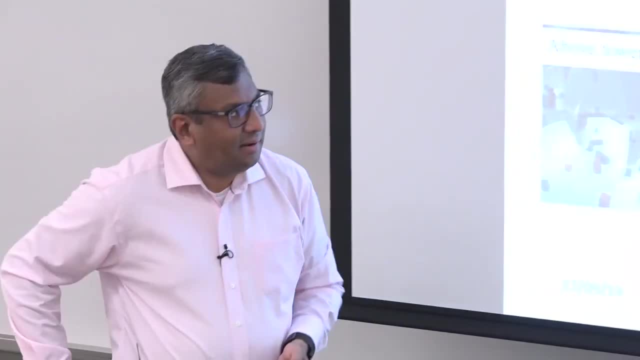 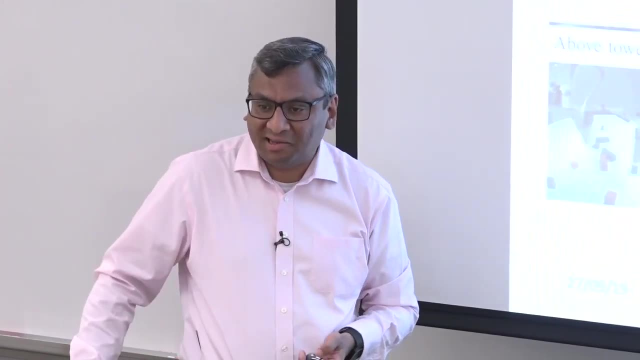 but it does learn that this is how you can sequence them. What's interesting here is that to a robotics person already this is a pretty sophisticated level of identification, because all the other things we knew how to do before this was just learning parameters in a single controller. 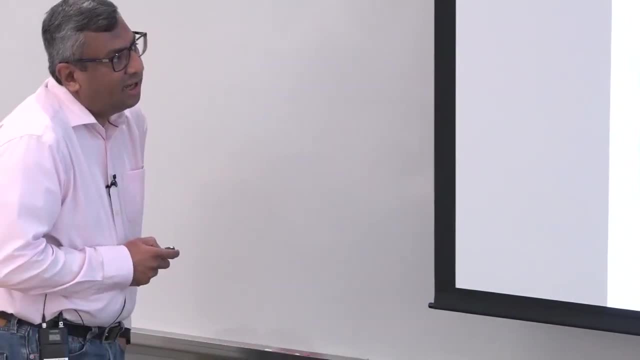 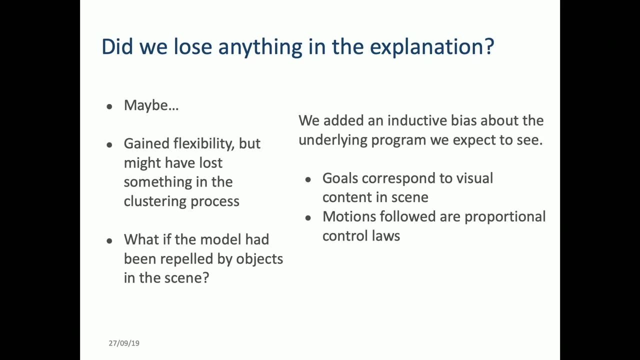 So now we are actually beginning to approach the system identification in a genuinely hierarchical sense. Of course, there are lots of questions you can ask. So exactly this generalization question of what have you given up because you said this is your parameterization? 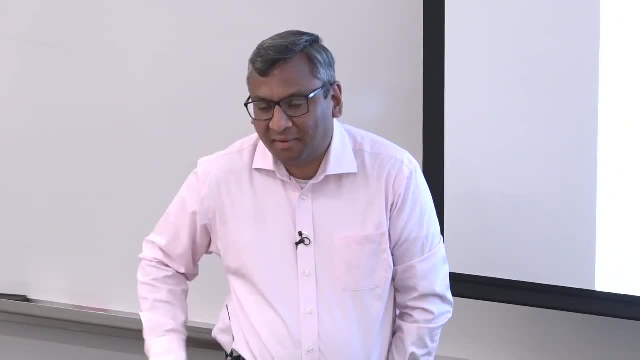 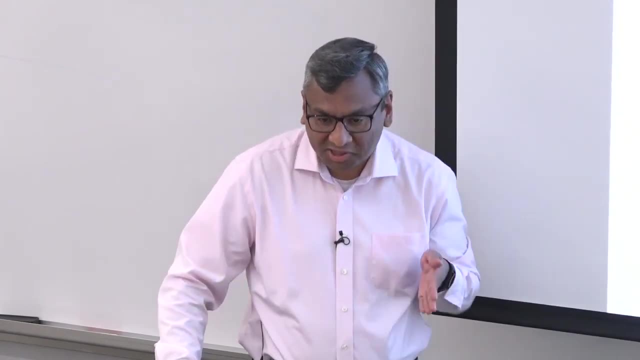 The most interesting one that only occurred to us after we finished the whole project- we knew about it, but we didn't consciously think- was that we were specifying that every local task was a reach task, Whereas you could have an avoid task as well. 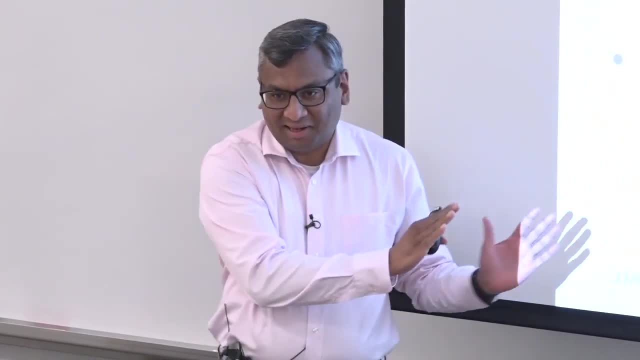 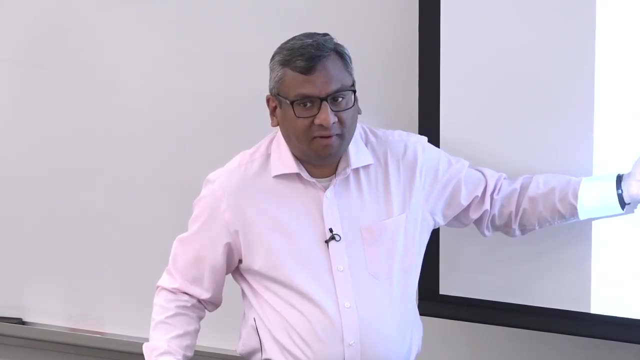 I want to reach here, but I want to avoid here and we weren't representing that. So there was no clean way in which you could take a reach controller and represent a void. So those decisions do matter. So this is a trade-off when you're trying to do model-based work. 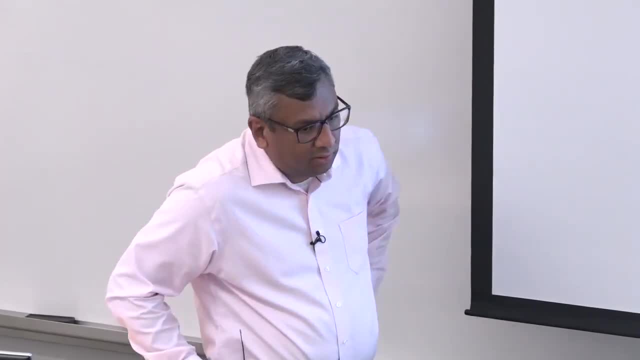 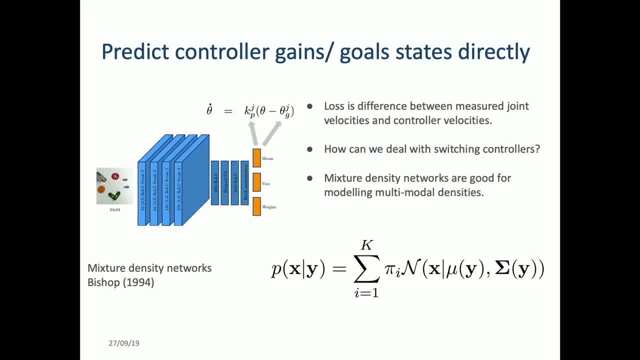 But then what I'm trying to say is that, to the extent that that is how the engineering design processes always work, we're trying to see how we can marry these two things together. So the next thing we did was to begin to take on some of the questions you're asking. 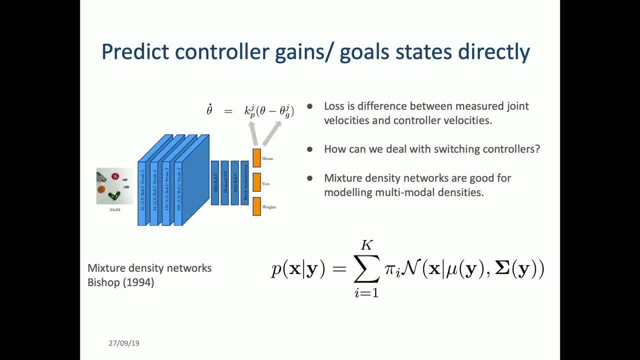 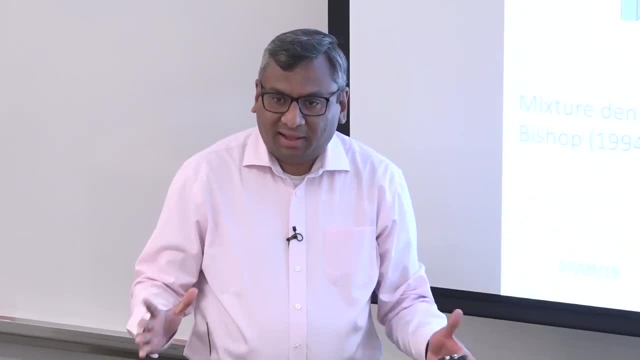 which is to say, can you keep this level of structuring, So can you keep this idea that you're going to have switching between controllers and so on, But then can you make the whole thing look exactly like how a typical neural network model would look. 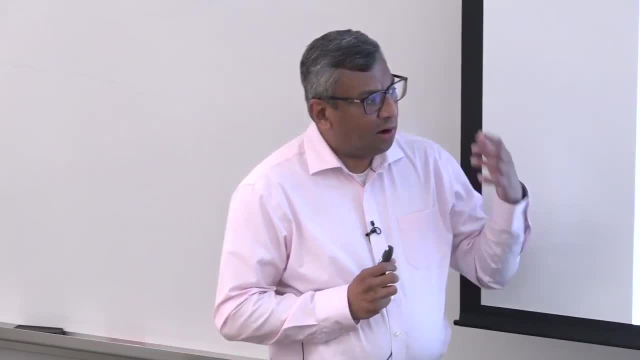 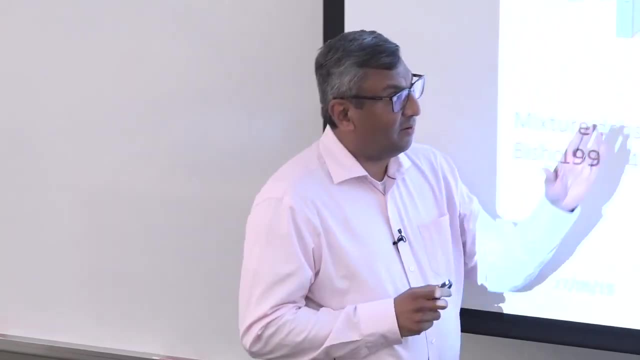 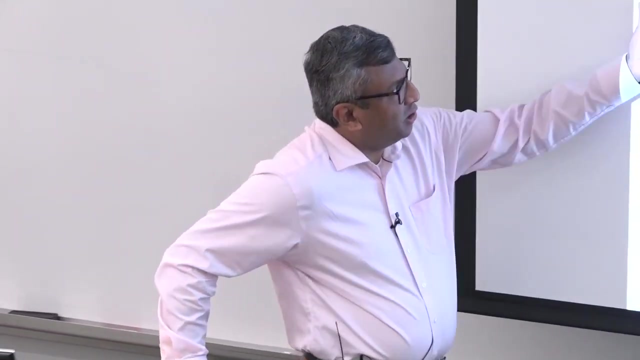 So what we wanted to move towards was to say that there's a lot of excitement about using things like mixture density networks within a neural network context. Can you somehow put that funnel representation at the end of this and describe one network that does this? So the network's job is 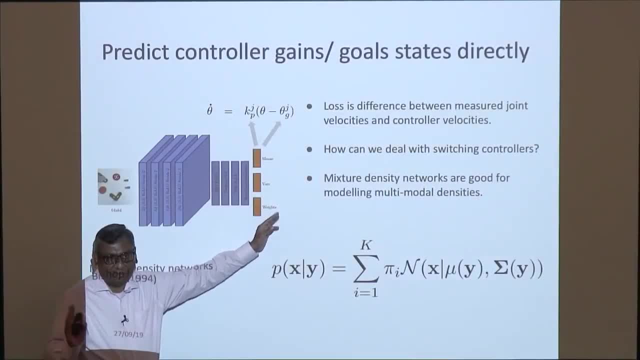 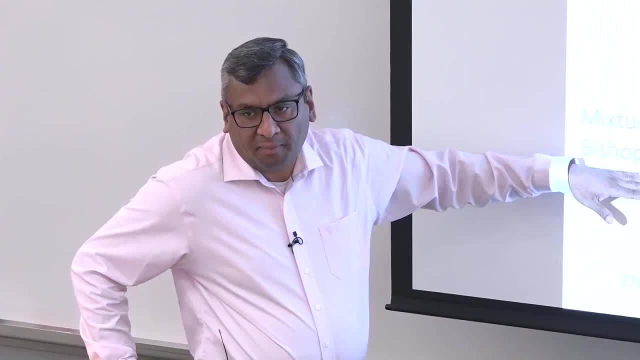 here's your input: just tell me what the action should be. So just learn the whole controller and then learn the fact that it's a switching model. So our starting point is the well-understood idea of a mixture density network, whose role was to say that I want to. 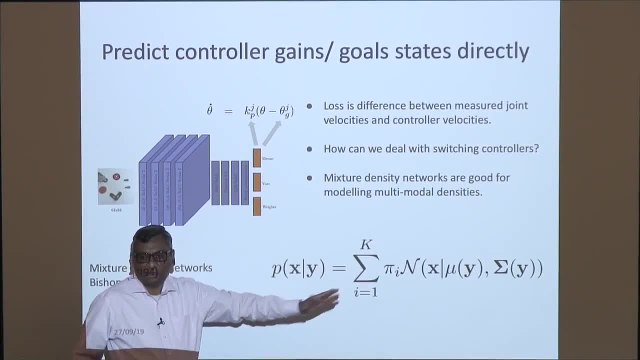 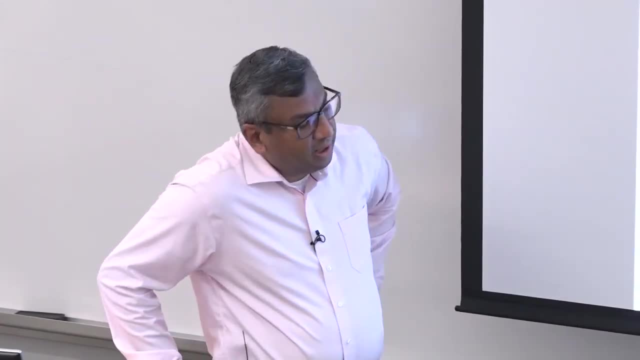 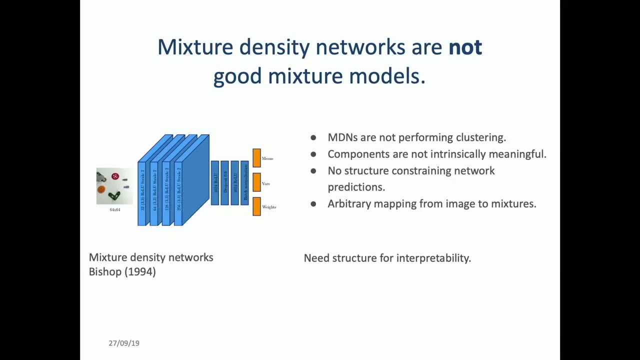 describe a complex probability distribution in terms of simpler components, and then I want to learn the weights for them. Now, in the way that mixture density networks were originally introduced, the objective was to solve the statistics problem of approximating a complex thing with a simple thing. 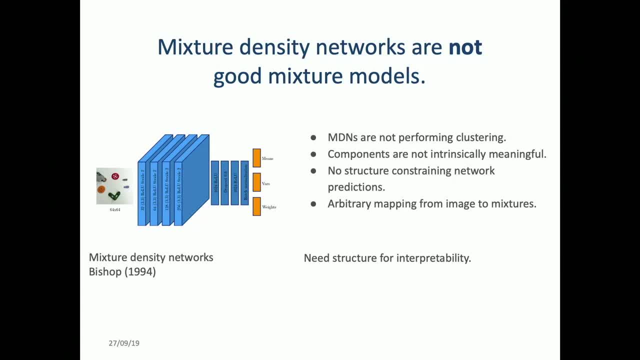 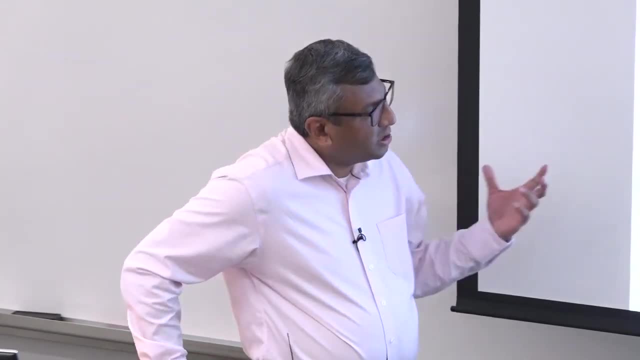 There was no requirement whatsoever that the simple components map to anything else. In fact, they did it because they were just carefully chosen simple components. So what we want to do is to somehow map them into an architecture like ours. So we introduced this variation on the theme. 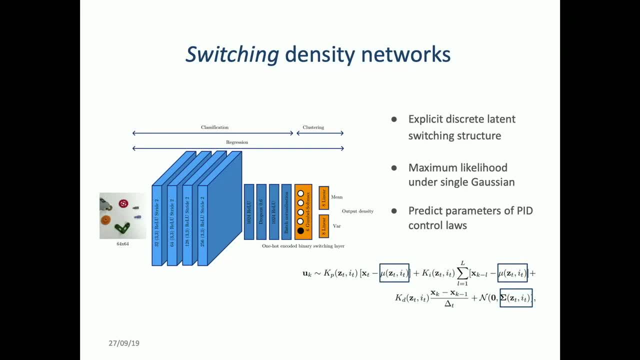 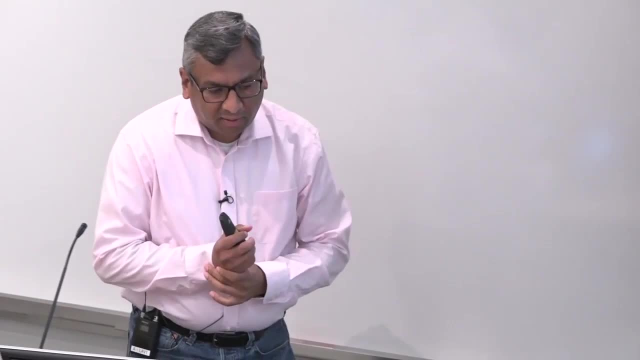 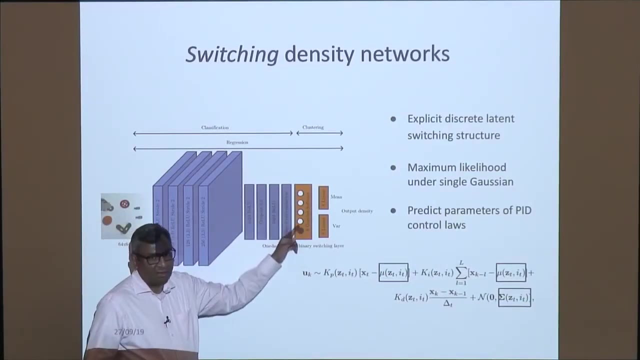 which still looks like the previous one, and the bits that we've introduced is actually this bit. So what we did is to create a different form of a switching network. So it's still a density network that builds from components, except that we are restricting it to switch using a bottleneck layer. 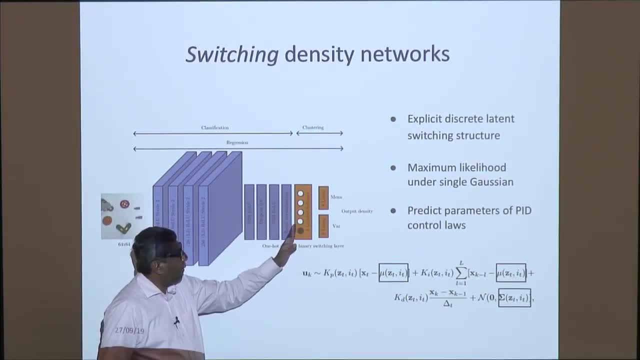 which is a finite number of categories, Then what it's going to output are the mean and variance of the goals, just like what I had before. So the goals were the points where the blue lines were ending up. So for those of you who played with these kinds of models, 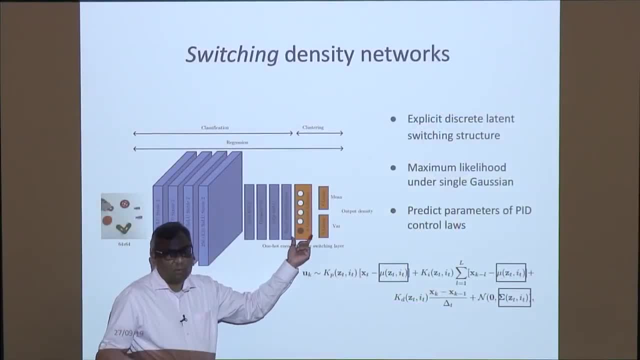 before the introduction of a Gumbel softmax. what it does is, as you change the temperature, it approximates a single category, but in the beginning it actually keeps a diversity of categories. What we want to do is to take the controller parameterization that is loved by. 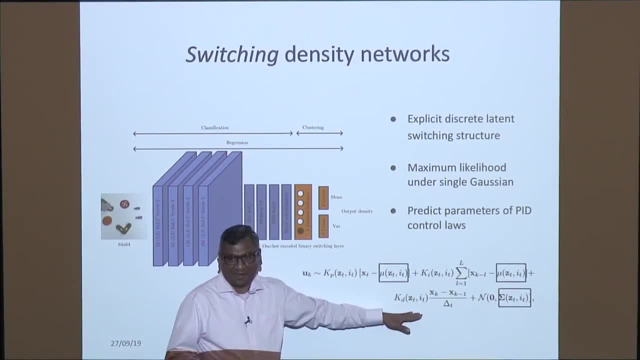 control theorists and 95 percent of the world's controllers look exactly like this, Except, what we've done is to take this structure, put it into here and then find a way in which we can just learn the bits and bits that we want inside this architecture using the network. 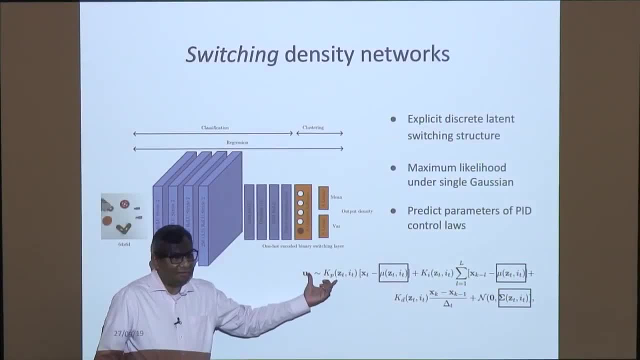 When I say, take this structure, what I'm saying is that this is a high-level description of the task. You still have to do it from pixels, which is what we are doing. So we're still doing all of this to go from pixels. 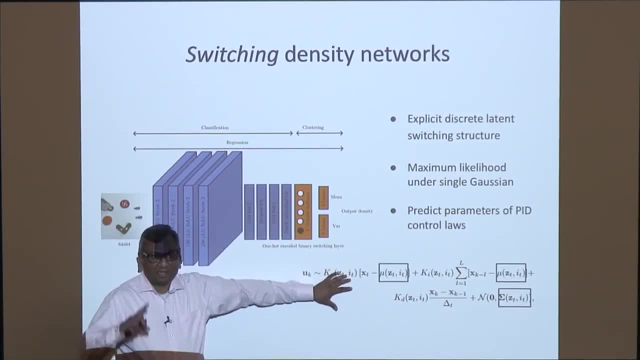 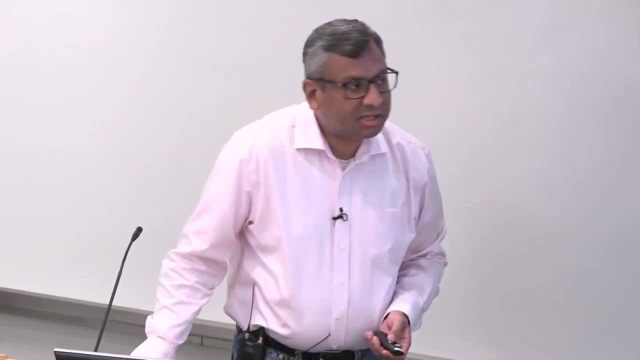 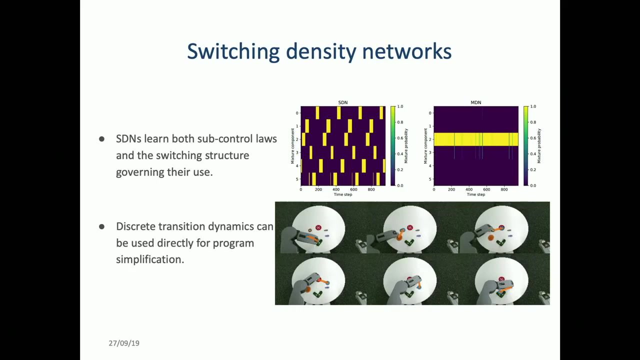 but then we're saying that the control bit, the bit that really matters for describing the task at that level, is not that complicated, So you can encode this in the network. Here's what we find, If you just did for the data that we are interested in. 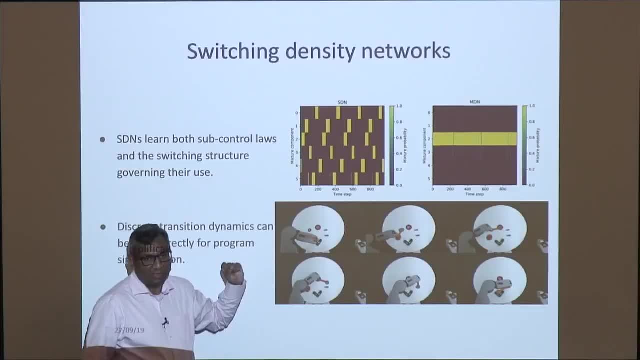 which is the tabletop manipulation task, which is a sequence of visiting these objects. if you just fit a mixture density, then what you get is something like that It does an averaging so that it just tells you that you're typically going to do one thing. 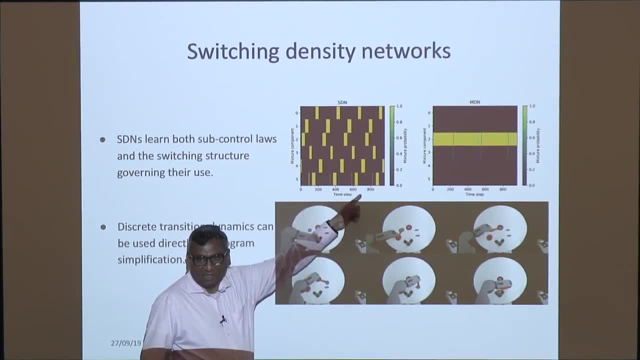 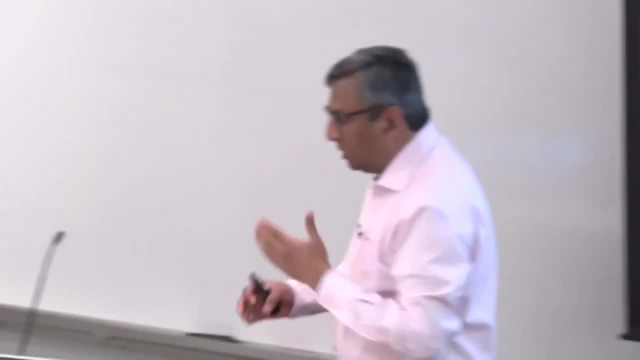 Whereas what we get from our network is a clean switching sequence, which corresponds to the switching sequence of you visiting different objects over time. So this is all learning from the data. So we're going from data which doesn't tell you what that structure is to. 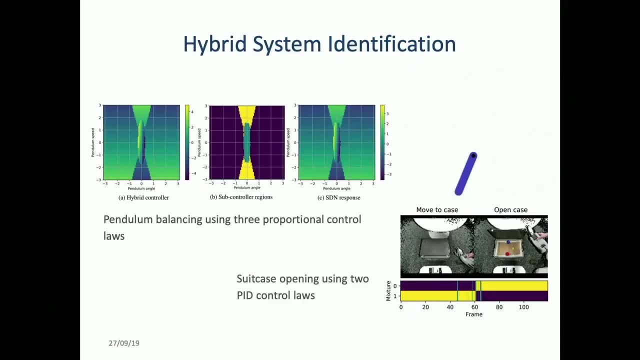 a model that tells us that this is the structure. We've applied this to a few other problems, So here's another problem that is very well liked by control theory people and reinforcement learning people, which is to swing up and balance a pendulum. 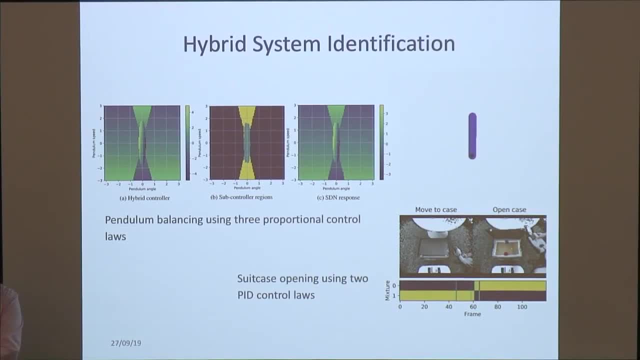 The interesting thing about this problem is that if you were first taught as a control theorist, as I was, then you will realize that this is elegantly simple and beautiful, which is that there's only really three things that happen here, and those three things can be described in terms of linear function. 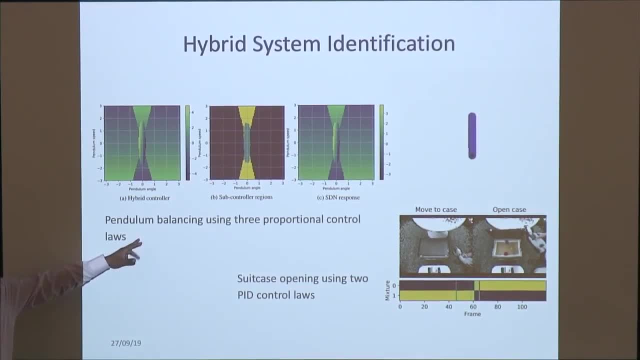 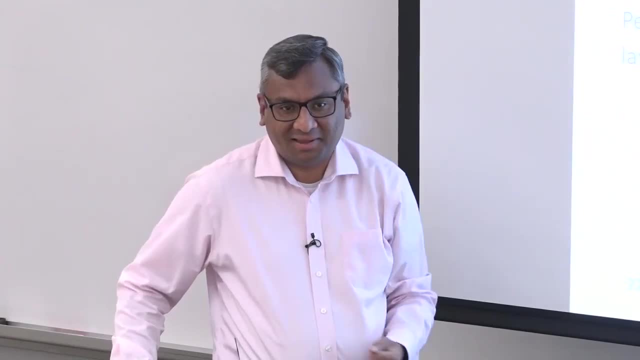 and if you do it like that, every controller you learn will always look like that. It turns out that those three things are discovered by our switching network. It discovers that there's a swing up phase, there's a balance phase, and so on. 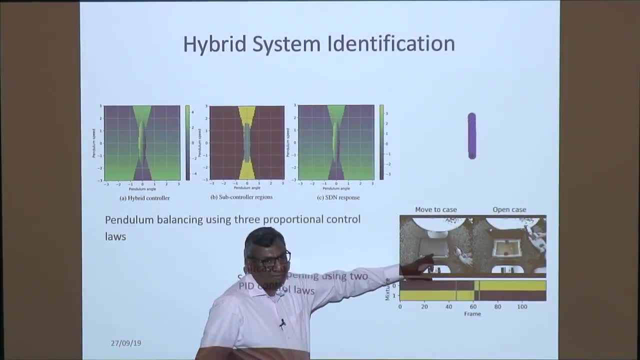 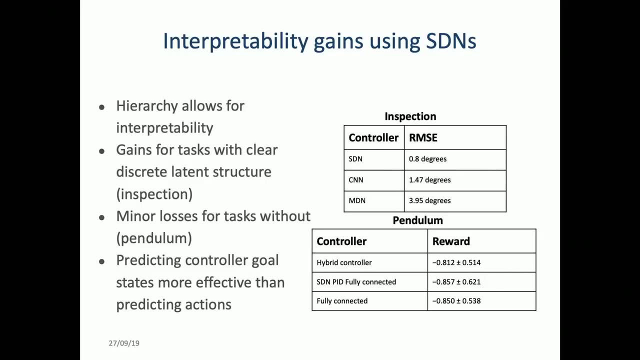 Likewise, we did another task which had to do with you switching phase, when you open a box and then it learns that you first have to reach and then you have to do something else. So what do we really get from all of this? There's an interesting observation. 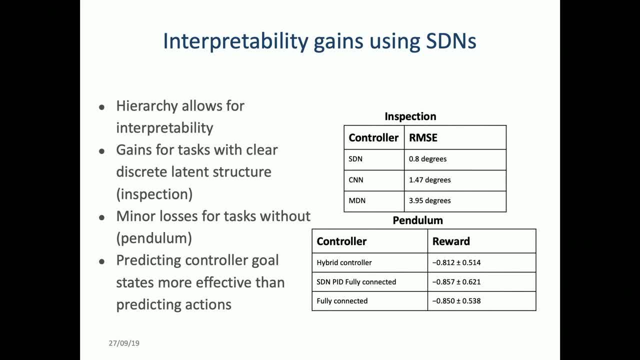 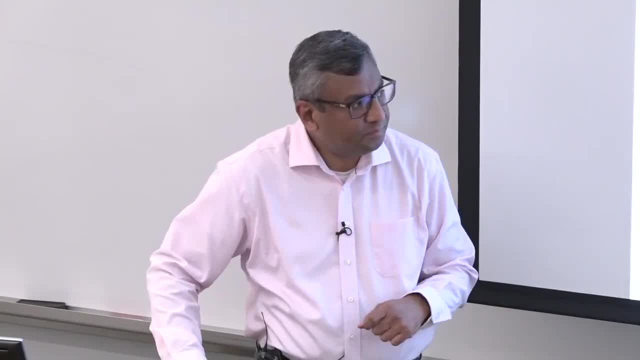 So we did all of this from the point of view that we are very much interested in interpretability, structured models, because those structured models lend to us the possibility of doing additional forms of reasoning, and that's what we set out with. But of course, you have to ask yourself the natural question. 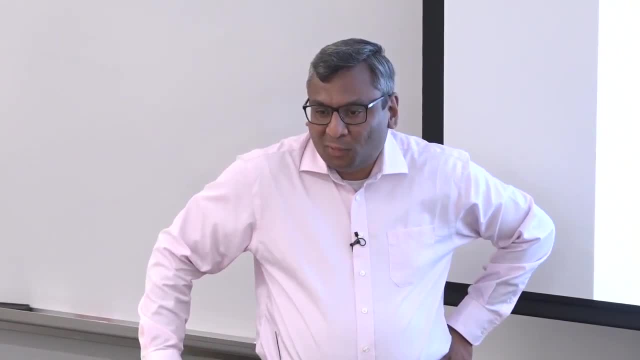 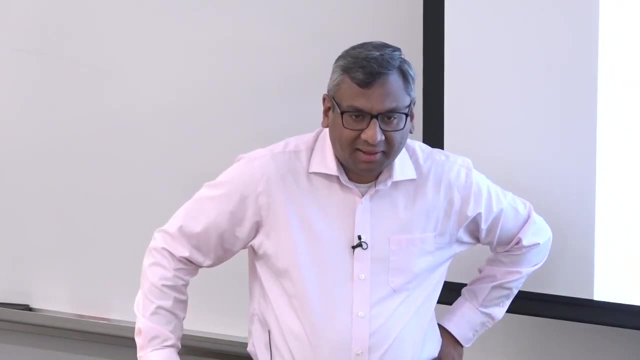 was all this necessary? Would the underlying model have done it anyway? Would some other model have done it? The answer is that if you have a straightforward controller task- and by straightforward I mean that there is no switching logic, there's only one state- 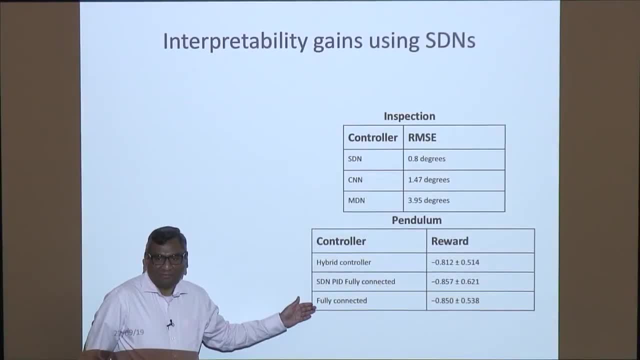 then our model doesn't do much better than anything else you could have done, which is also equally sophisticated. Subject to noise, we might even be slightly worse because of our training procedure, But when there is switching logic, that is intrinsic to the task. 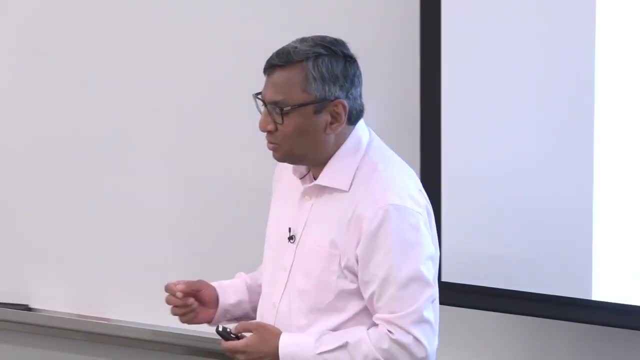 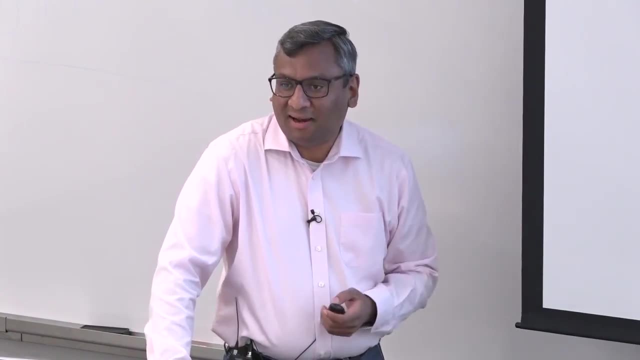 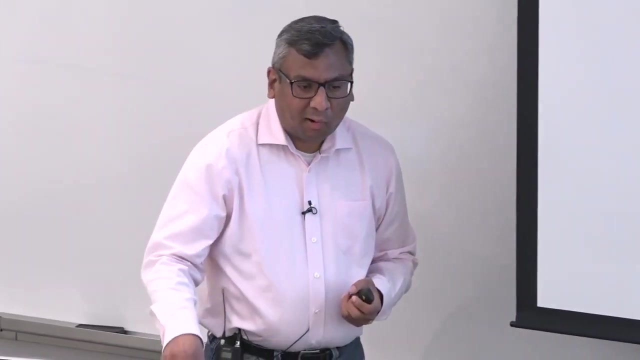 then we do substantially better. So this makes sense, because that's when most methods for training that I'm aware of actually struggle is when there is a deeper underlying logic that isn't being picked up by the network. So for us, the takeaway here is that the need for 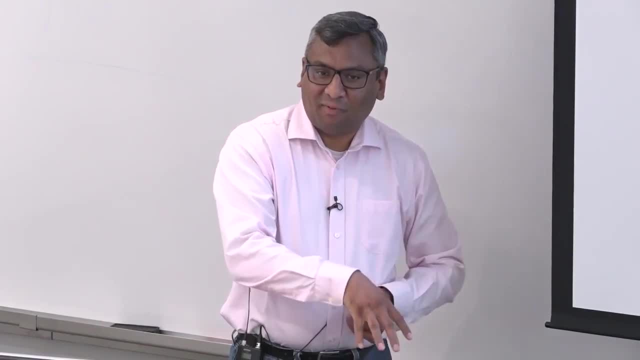 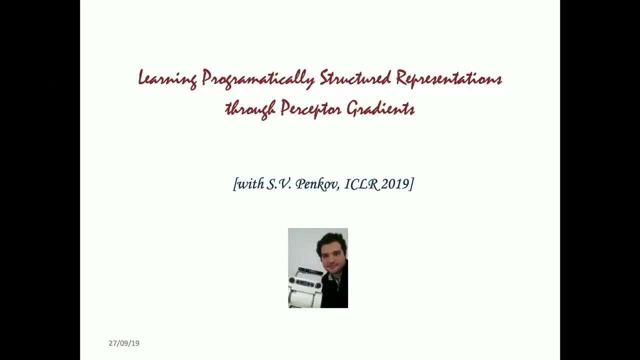 all of this structure is the fact that the world is structured like that, and we are just trying to find a way in which we can somehow bring that into our training procedures. So that's one direction on all of this, and if you mentally remember my arrows, 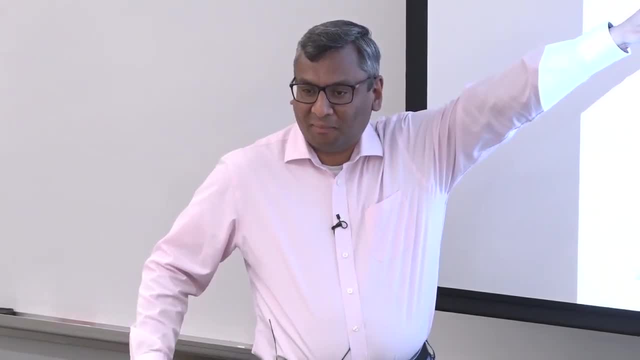 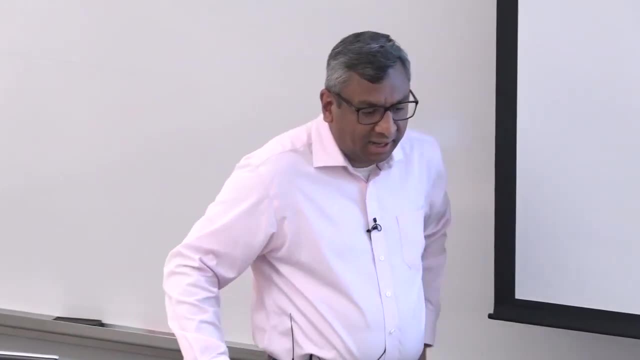 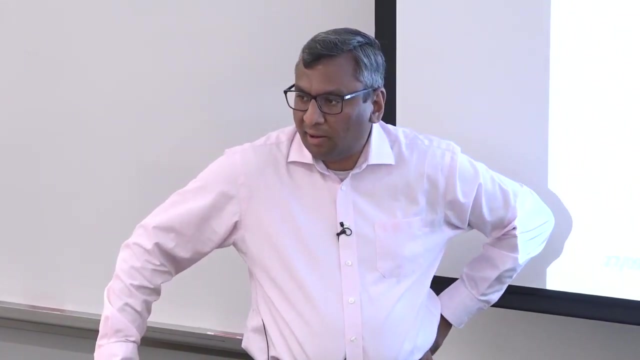 this is the direction of us, going from human demonstration to some slightly more abstracted description. Then we are curious about: can you also do a little bit more of the other side, which is, if you know that you have this kind of structure, can you somehow bias policy, learning or 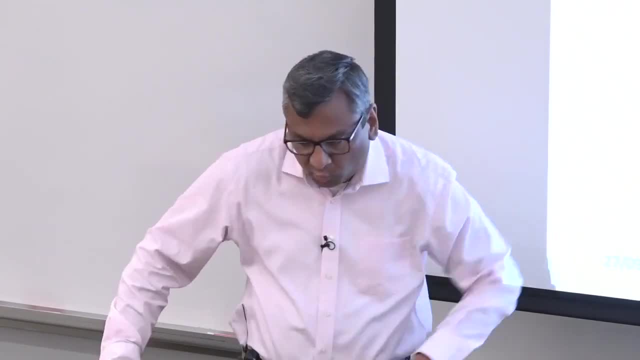 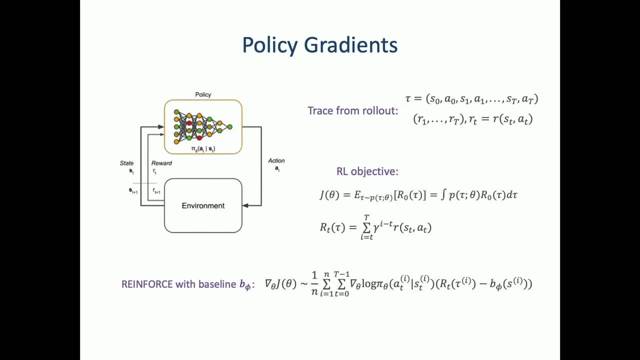 learning to act by using that kind of structure. So this is work that we did, which was motivated by this idea that. so, if you're familiar with reinforcement learning, there's a very straightforward way of thinking about lots of different control tasks, which is called the policy gradient method. 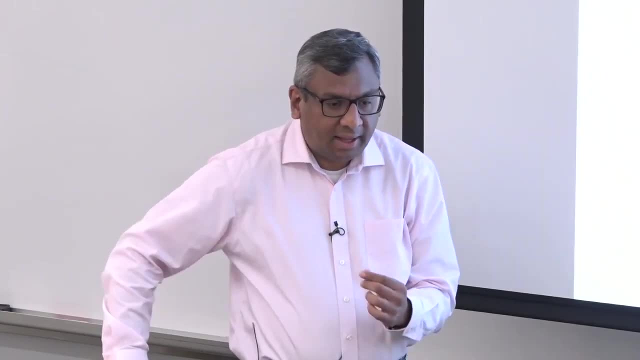 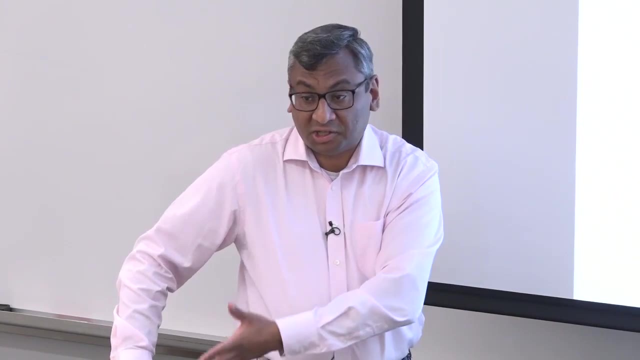 which, in simple terms, is the intuition that, most of the time, you can define a policy that takes you from state space to action space, and that might be much lower dimensional than even your state space. So what you're interested in is to represent that in. 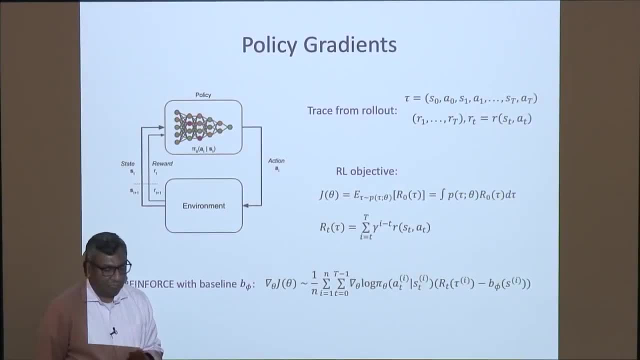 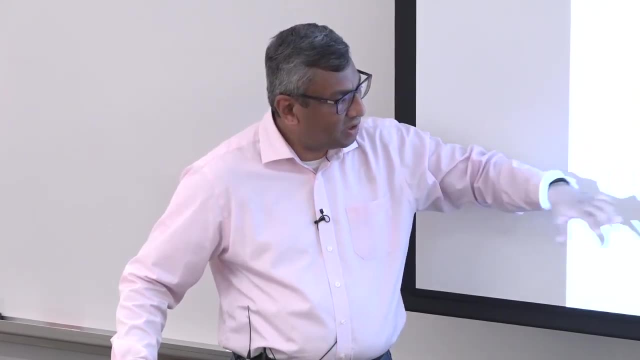 a certain way and then do gradient descent to try to find that policy. So one very simple approach to using it- and this is by no means the most sophisticated way to doing policy gradients- is called reinforce, which is that you simply take the cost function that's defined in terms of 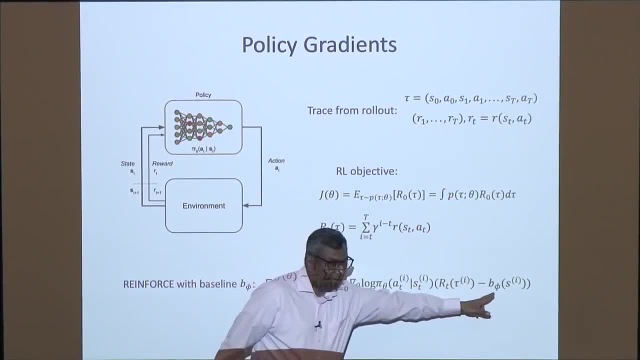 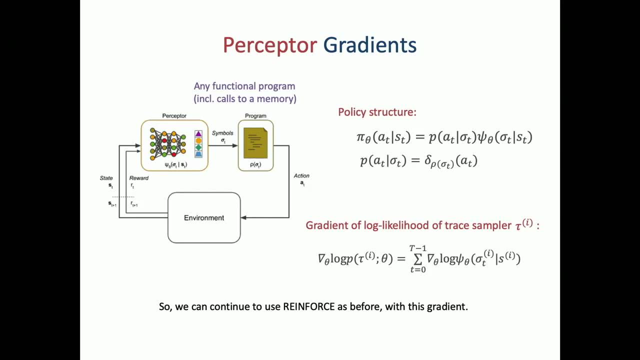 your long-term reward, and then you take the gradient of that and then you add something called a baseline which stabilizes the variance of this estimator. What we did was to say that you can take that same loop that we're all familiar with and we've come to love. 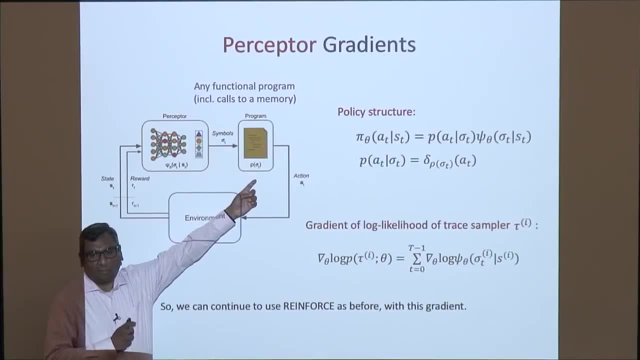 and you can change the policy to have a factored form. The factored form is essentially telling you that what I had- a switching logic or program- goes in here, and what I had is the interpretation from pixels to some intermediate symbols. that goes here. 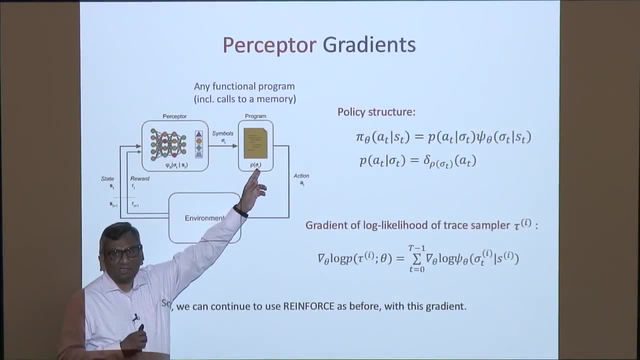 This bit I represent, there's a network. this bit I represent is just a program. So in my previous one the program would have been the bit that I learned that says you go from A to B to C and so on. What we are saying is that in a lot of tasks 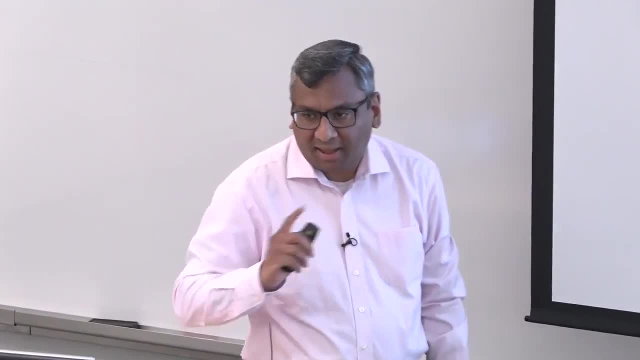 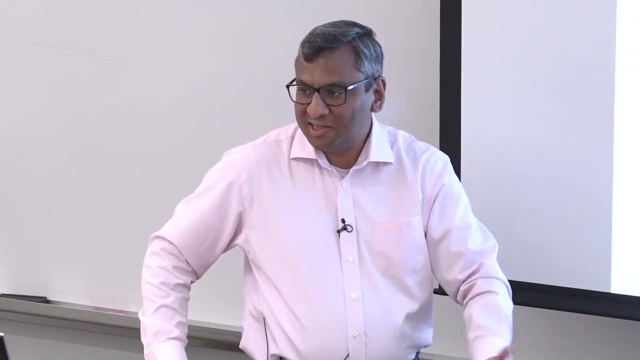 we actually have a pretty good understanding of what that program is. Not only do we have understanding, we might actually have very good technical analysis of convergence properties and stability properties and robustness properties of that side. and we are asking: is there a way to marry the two? 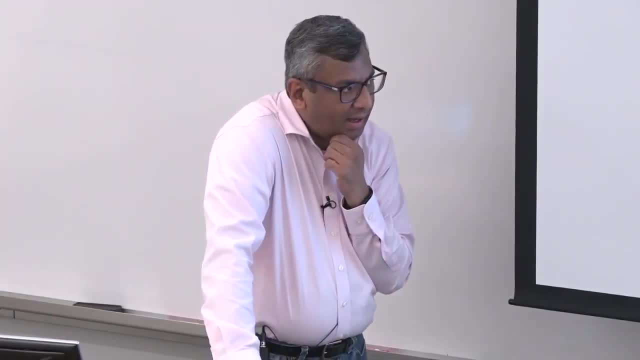 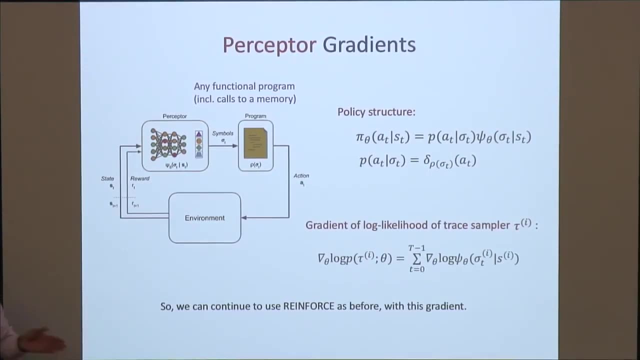 The short answer is yes. there is a way to marry the two. In fact, if you do it like this and if you set it up in a certain way, you can preserve exactly the same training procedure that Reinforce used to use. and then what it turns. 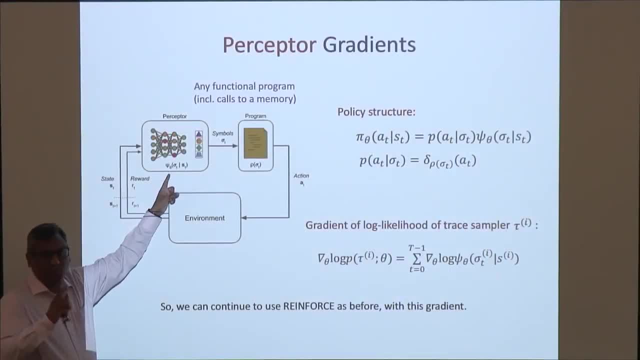 into is just training this network to produce the right symbols which have the characteristics such that this controller is actually useful. I've just defined reach and I haven't said reach to where and reach with respect to what. but if the network could learn those things. 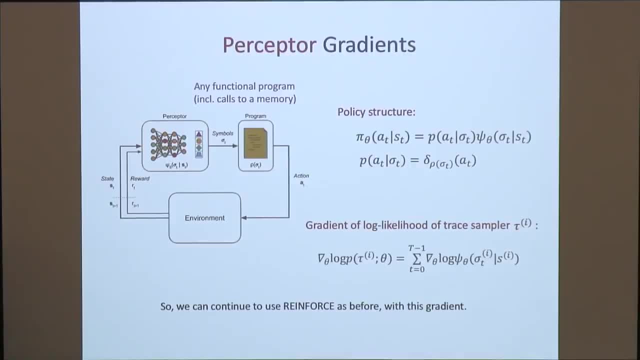 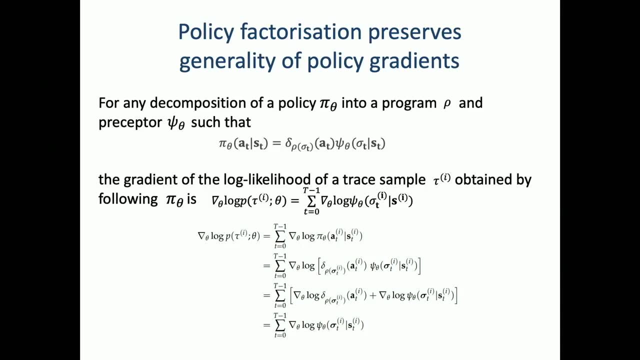 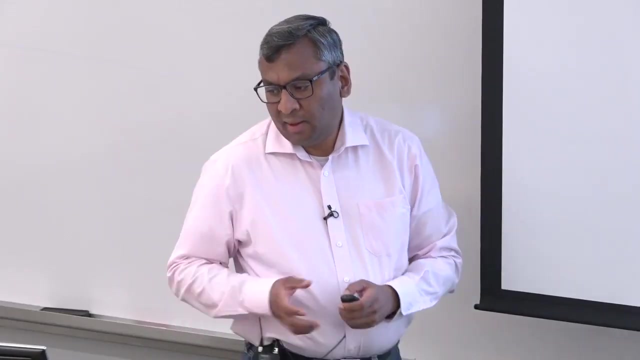 then actually reach is enough. I can actually do quite a bit and that's the intuition here. So there's a small technical result that actually says that it goes through. We haven't changed anything about convergence properties of policy gradients by factorizing it in this way. 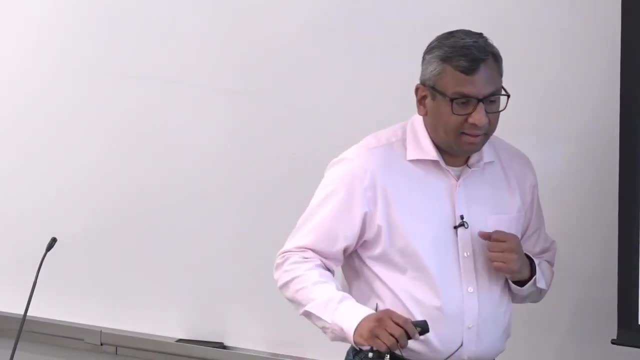 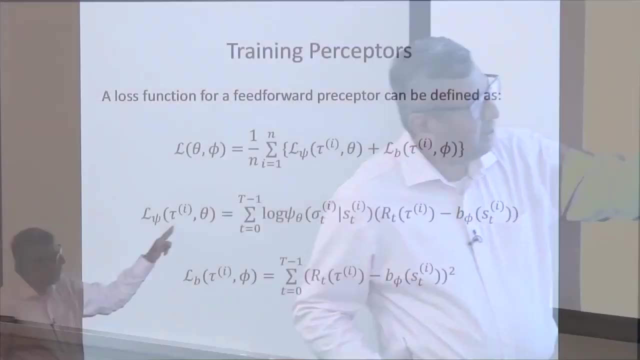 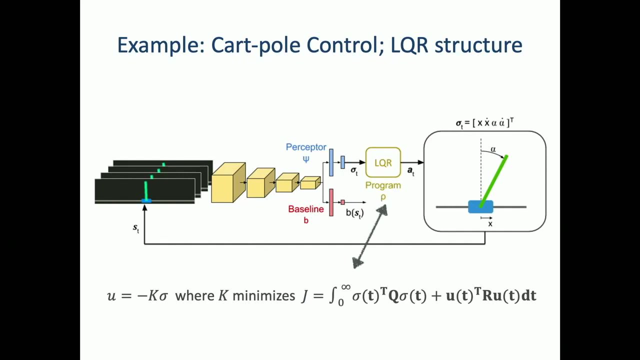 The training procedure essentially just becomes the process of us defining a loss function, where we just took that Reinforce gradient description and we turn that into a loss function. So we train the baseline and then we train the Reinforce loss. Quick question: what's about Reinforce that allows you to do it? 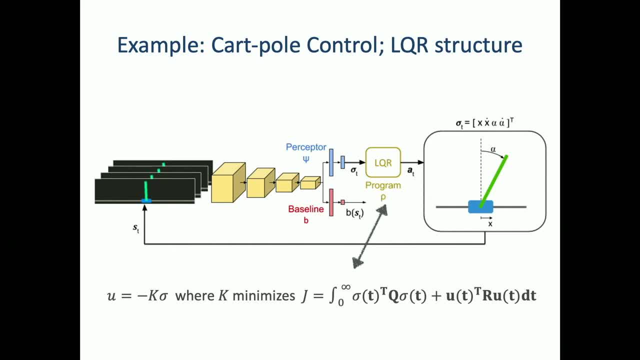 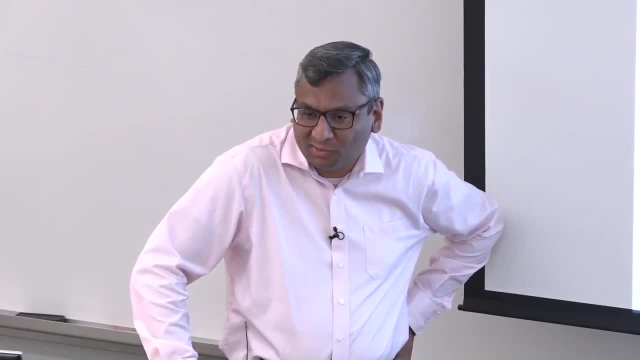 It's just the most general form. It's actually not the most sophisticated one in the sense that you can have much more sophisticated gradient estimators with stochastic mini-batch and so on and so forth. Is it similar to any of the policy gradient methods? 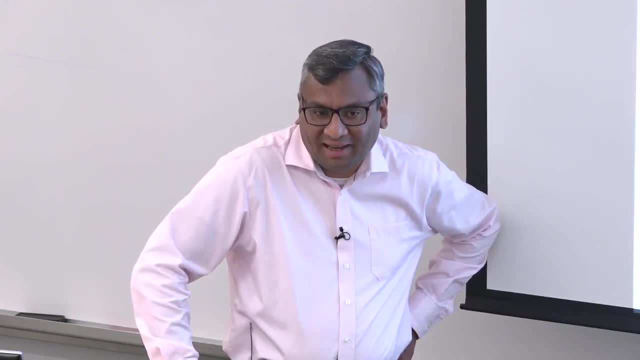 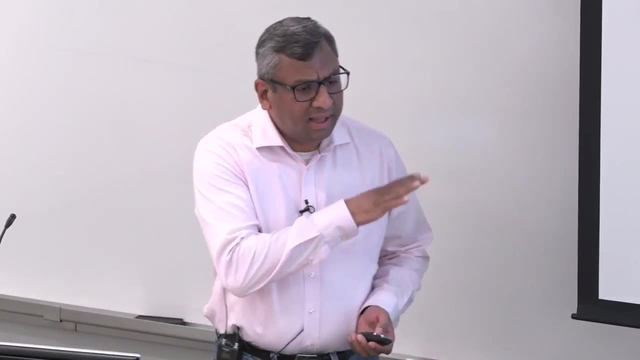 In principle, we could have done it with any other. In fact, if we did it again, we might try it with a more sophisticated version. Yeah, But the bit about what we are saying is more in the fact that you can factorize the policy like that. 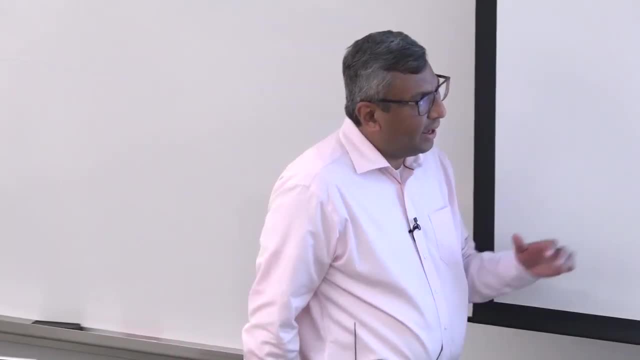 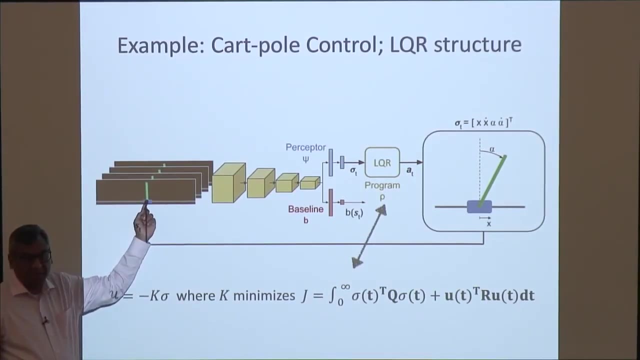 So here are some examples of what we've managed to do with that. So here's the pendulum swing up task. The task is defined in terms of go from pixel description, So we don't have a state space description, So we're just giving you the images. 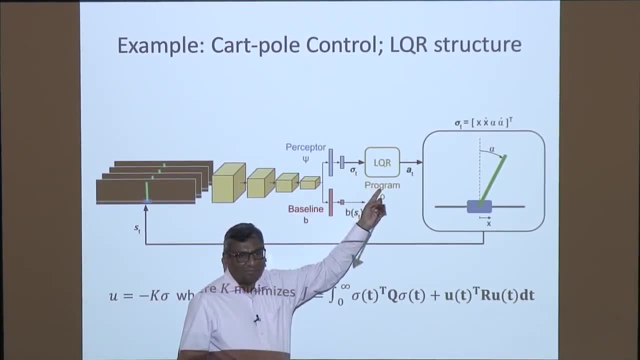 But what we are saying is: we know that this is the way to stabilize the pendulum. We don't know what the pixels map to exactly, but we know that that's how you do it In many domains. this is how it works. 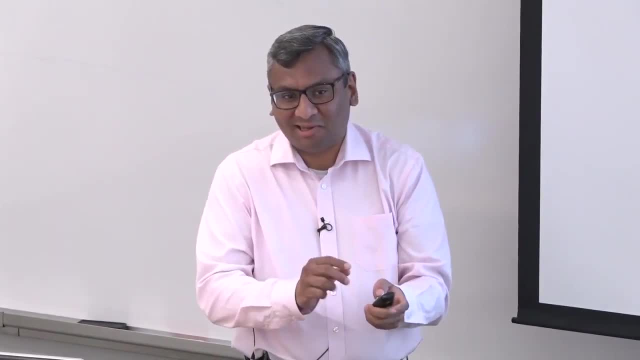 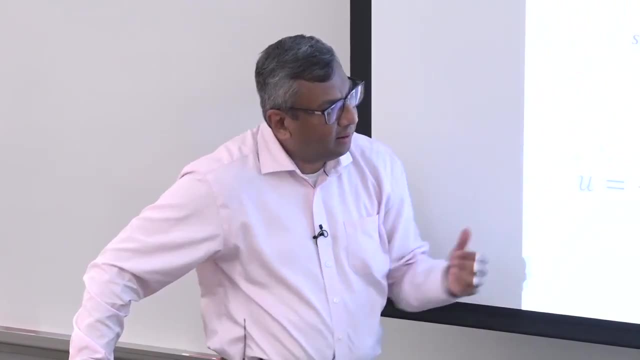 So specialists can tell you that this must be the general structure. What they get wrong is the embedding. So what our procedure allows us to do, then, is to train in the loop. When we train in the loop, we actually get improvements in terms of the convergence rate. 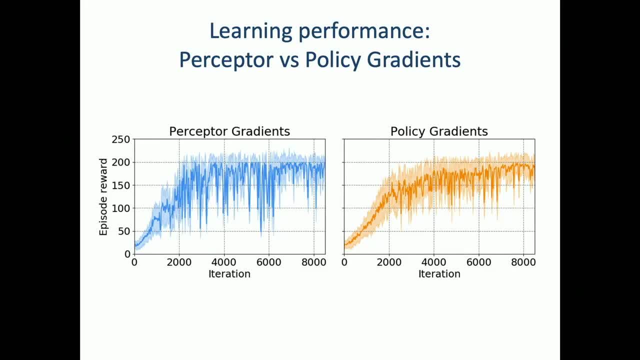 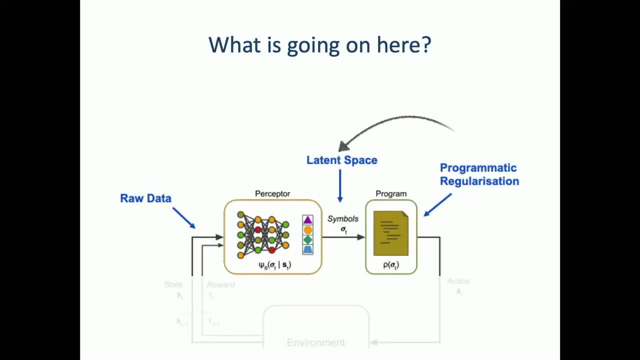 So if we did it without all of this structure, it takes much longer to reach the same level of performance than if you did have this kind of structure. What's going on in all of this is that we are really regularizing the latent space. 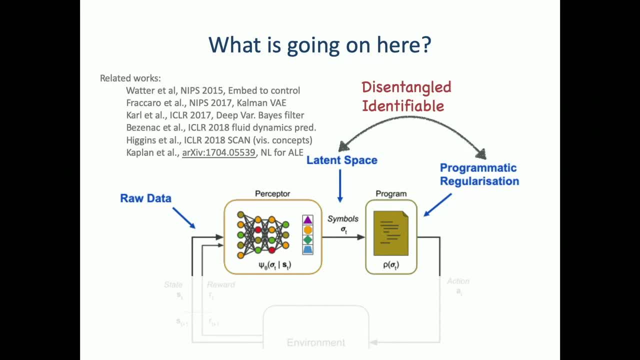 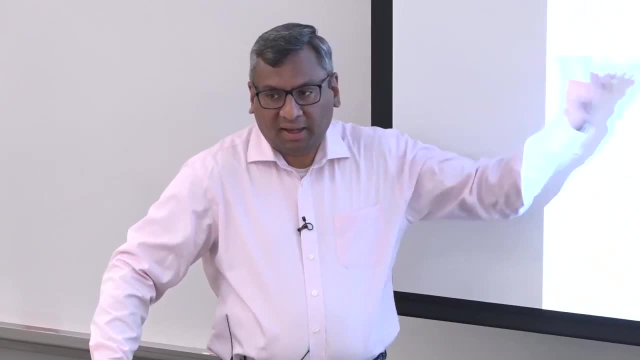 That's being learned. So when I'm just giving you the pixels somewhere, you have to discover the fact that there is a joint angle and there is a state and so on and so forth. That's being picked up in this process. But by telling you that it must fit, 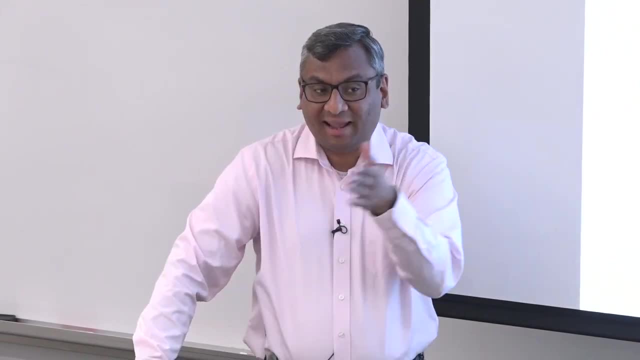 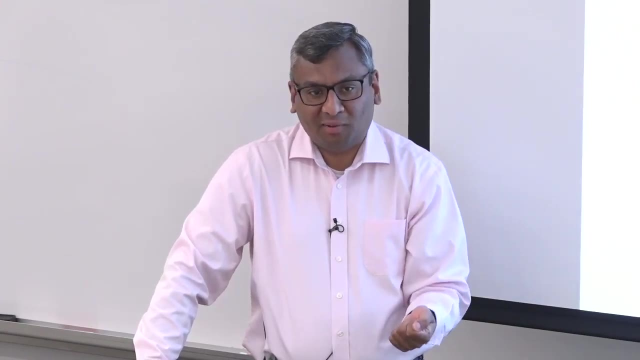 this program and the program must be useful in the task. I've actually regularized the problem quite a bit. I'm forcing you to pick up that because with any other variable that you pick up from the pendulum- like if I picked up I don't know- reflectiveness- 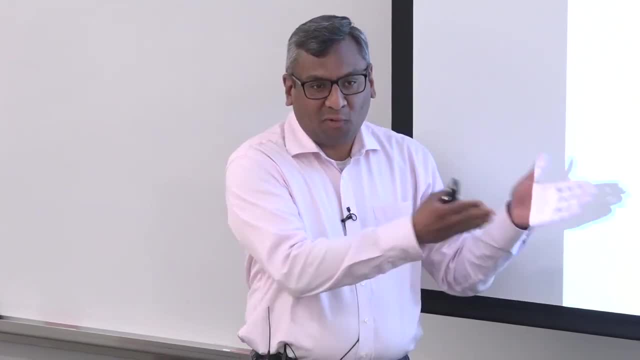 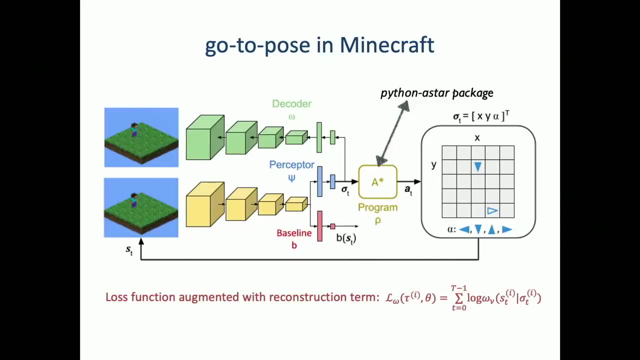 it will be useless when put into an LQR controller. So I'm forcing you by the task to do something like that. So we did this on a sequence of other tasks as well, just to see the extent to which it could be useful in planning. 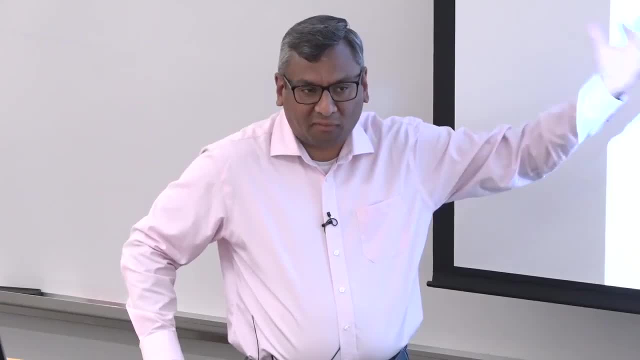 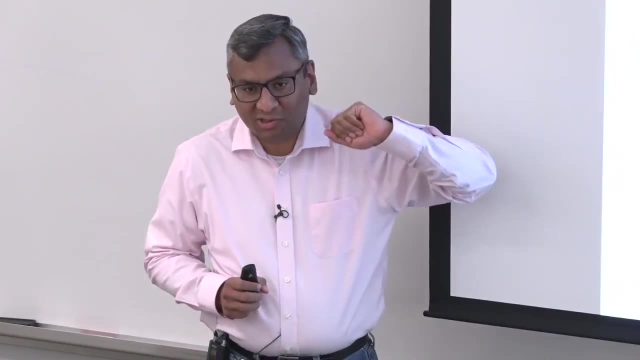 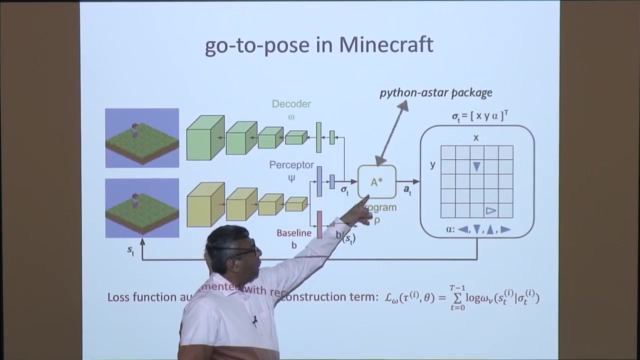 We did it with Minecraft and, of course, as you all know, this is essentially just an A-star style planning problem of getting the agent from one place to the other in one of its instantiations. For us, the important bit was that we deliberately just picked a library off the web for doing planning. 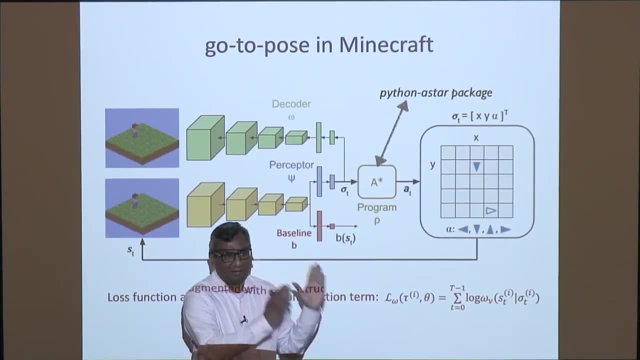 So this was literally a code library that we didn't touch in any other way. We plugged it in and we said we know that much. Then the network has to figure out what inputs to feed to that library from the pixels, using our training procedure with Perceptor Gradients. 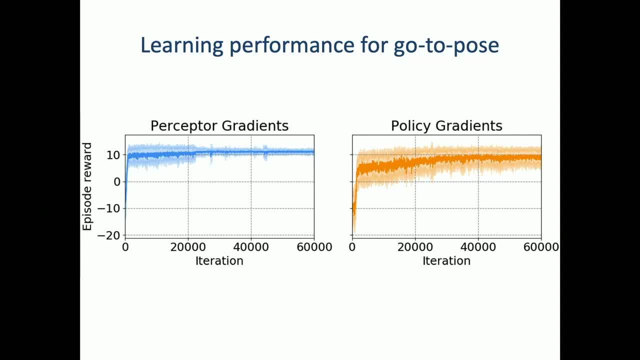 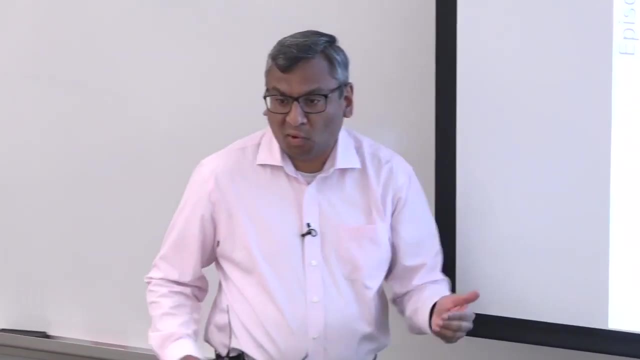 It does that, it learns to perform the task and it actually does it with a significant boost. Now the x-axis has actually changed from my previous slide to the difference between this and this is actually much more substantial. So we actually do begin to get more and more of a boost. 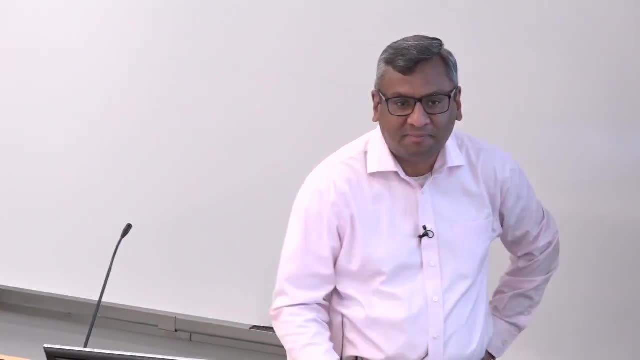 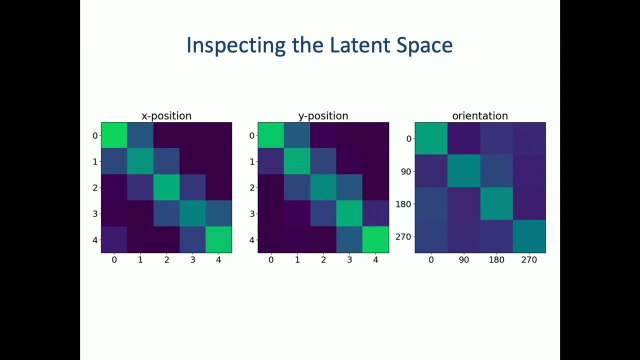 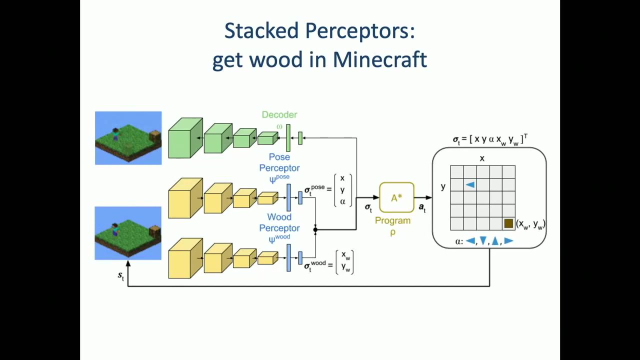 the more and more complex. the task is exactly like in my previous example. So then we can find out that the latent space has some meaning. So when we look at confusion matrices, our description and the discovered description lines up pretty well and we can begin to stack them. 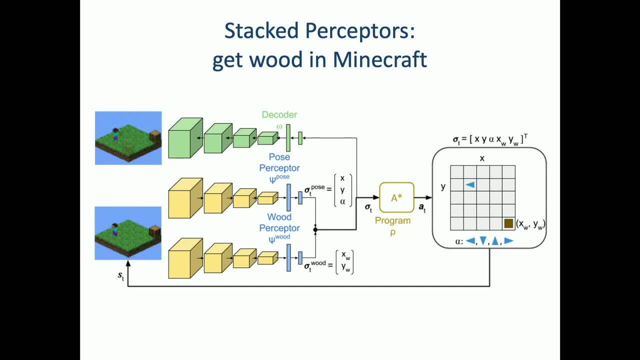 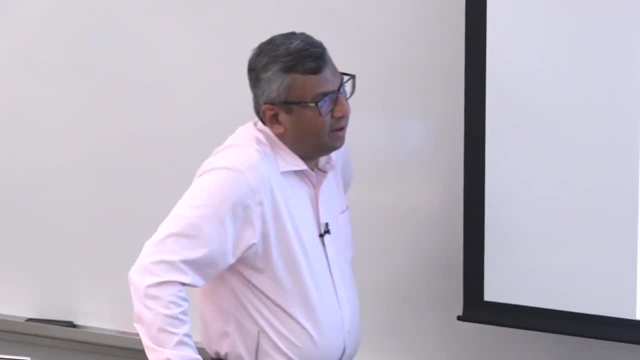 So, just like I can do it for one, I can stack them and then, along the way, I can try to do a closed loop with an encoder and a decoder so that I can make use of those kinds of representations By the time I'm looking at stacking multiple tasks and so on. 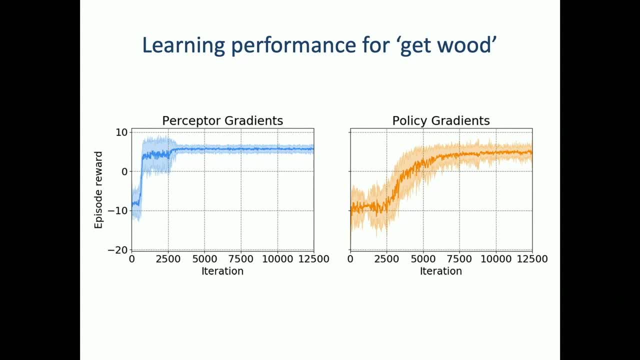 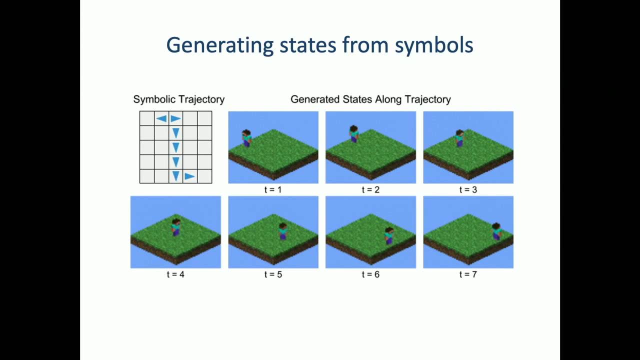 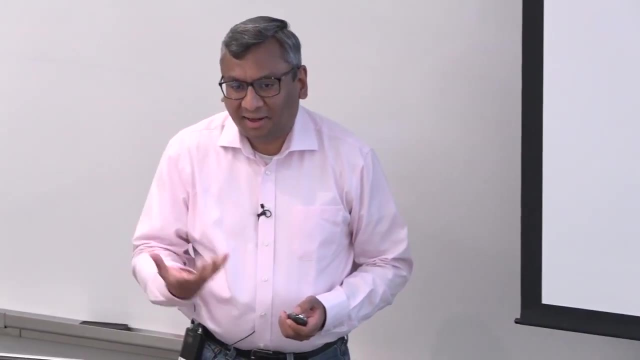 the learning curves begin to look substantially different. We're beginning to get substantial improvements in learnability. The most exciting bit of all of this result is that the symbolic descriptions that we are learning along the way in the bottleneck layers actually are useful. They tell us something about the task. 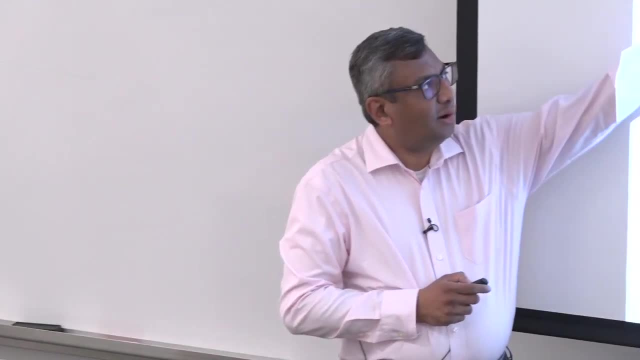 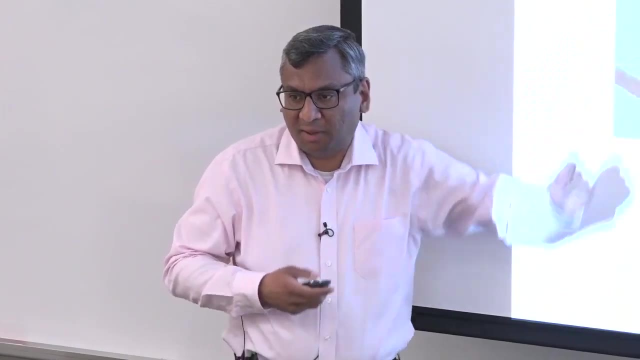 So it's discovered that actually, the underlying task in all of this is just a grid world task. It's not obvious if you look at it from pixels, but the underlying task is a grid world task and that's been discovered in this process. 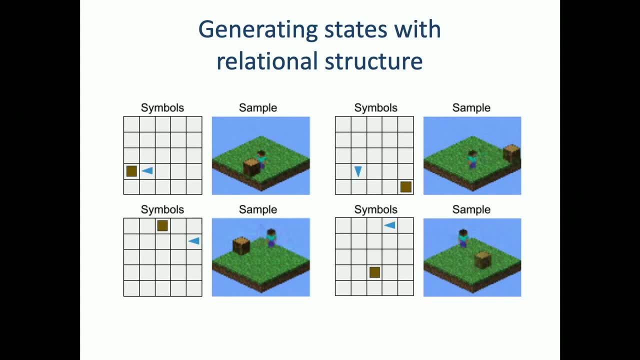 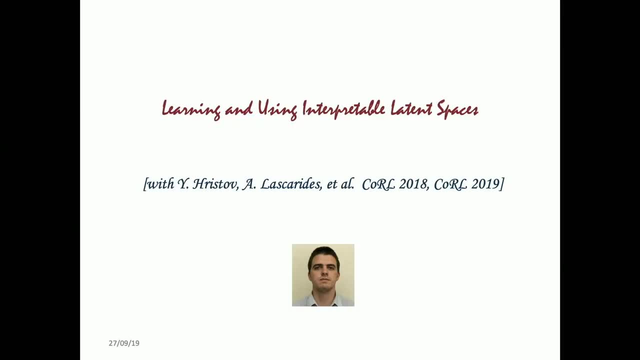 So we can describe the task now in terms of relational labels instead of just the underlying state space. So we've gone up and down the loop now. So first I showed you some results that tell you a little bit about if I've given you demonstrations. 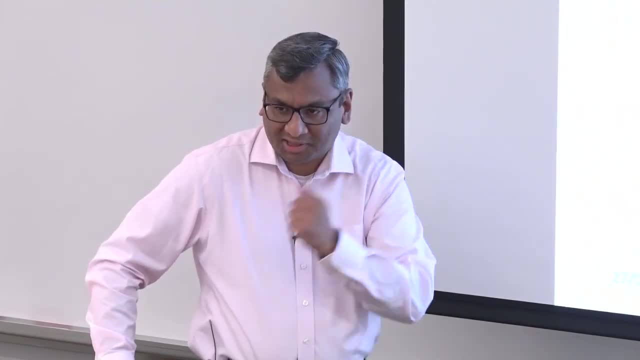 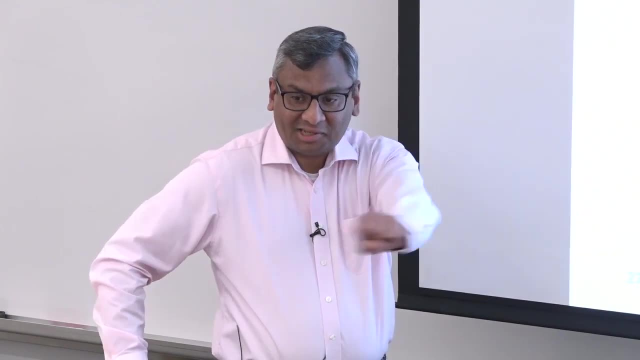 then how do you go from demonstrations to useful abstracted descriptions that are compatible with engineering ways of thinking? Then we looked at if you had some description from the engineers, how would you put that back in? In both of these we are doing more and more. 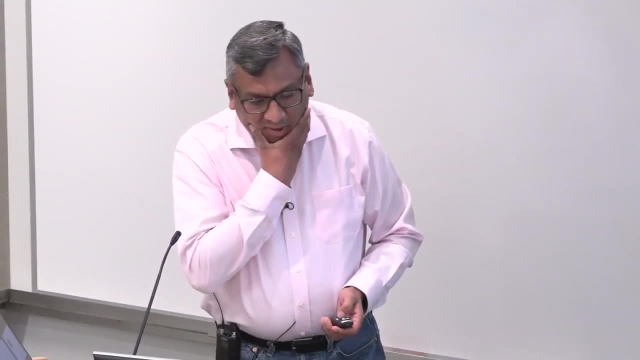 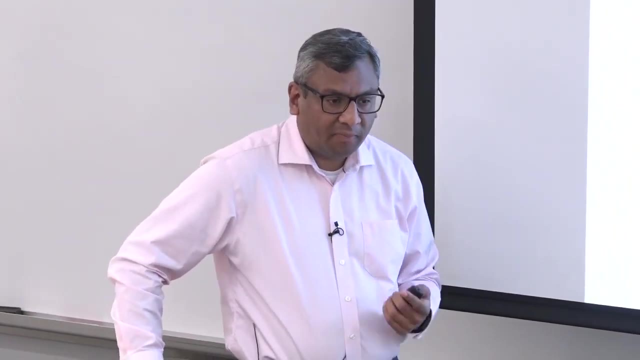 So I want to end in maybe the next five minutes or so before I come to my concluding remarks, By giving you a glimpse of some work we've been doing about more explicitly playing with the latent space. This is the bit where I said I have more slides than I want to cover. 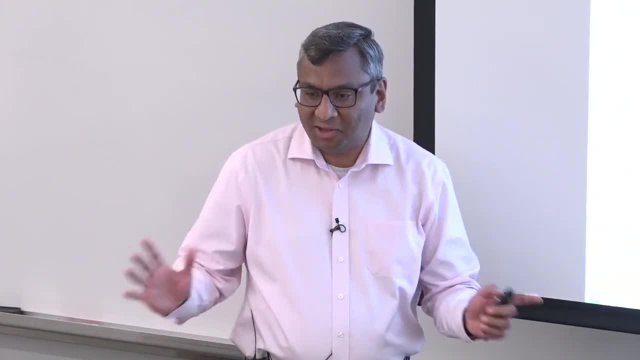 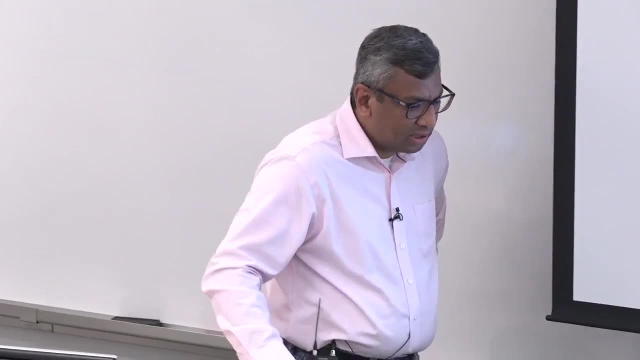 So I'll go through it quickly by picking on the highlights, but I'm very happy to discuss all of the details with you if you have specific questions. So the thing we were interested in when we started doing this work was still thinking about the learning from demonstration framework. 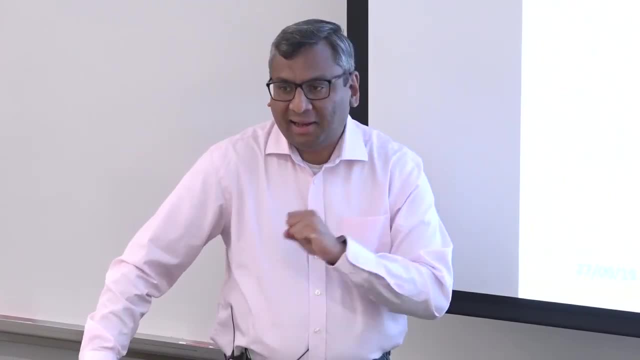 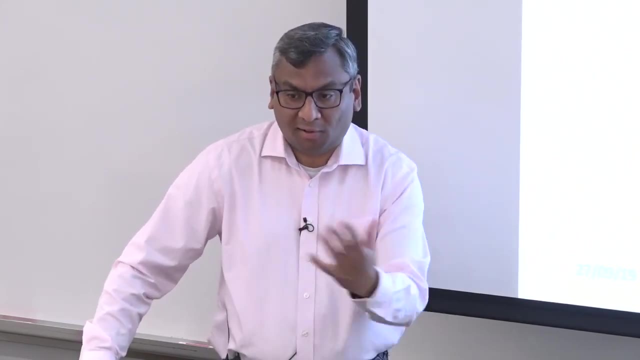 of people giving us instructions. We wanted to ask: how high level can the instructions get? So if you really want experts to give us information, like your typical car mechanic or your typical brain surgeon- actually, they both speak in very similar ways from the point of view of the machine learning model. 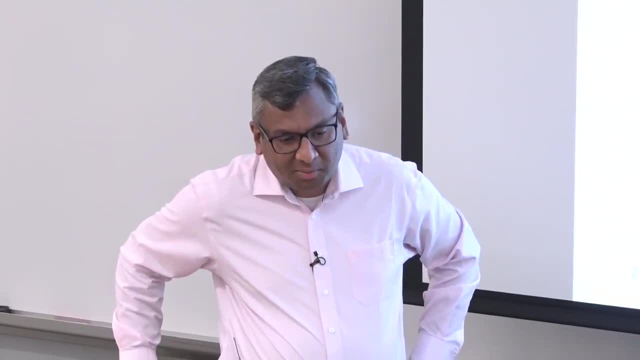 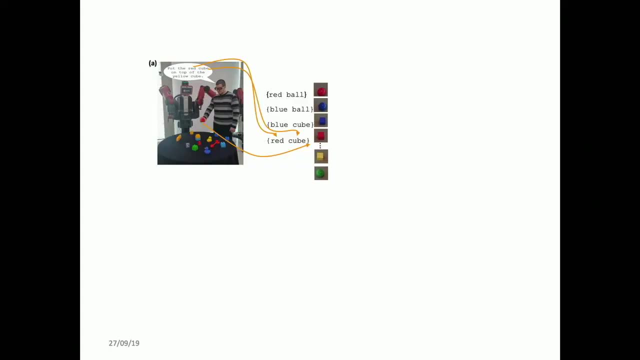 Then they're going to give you a very high level information, such as: when this is a bit soft, then insert it like this: You have to ground everything else about this. You have to figure out all of the rest of it. So we were interested in this question of how do you go from. 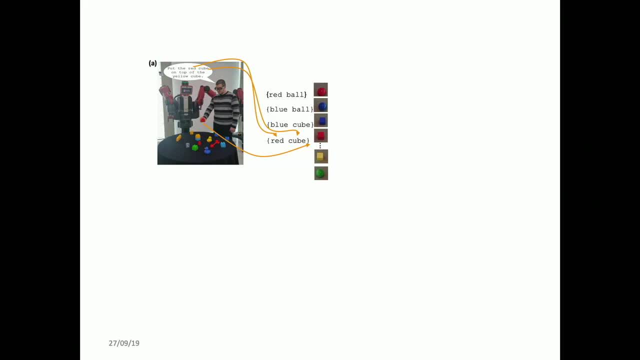 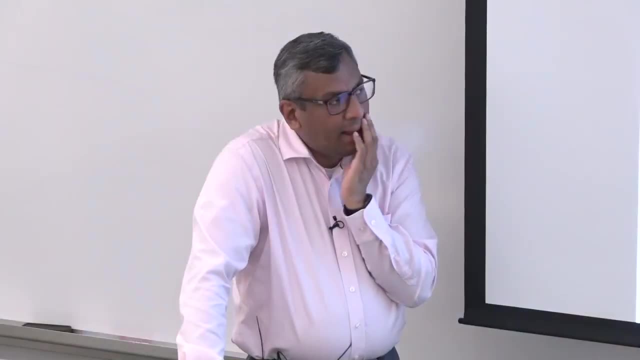 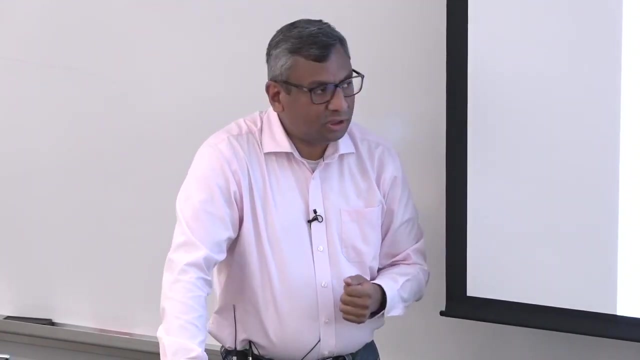 high level descriptions that are matched with otherwise unlabeled data and go through a labeling process so that you figure out that all soft meant this. So in our first experiment we were playing around with things like color and size of objects and shapes of objects. 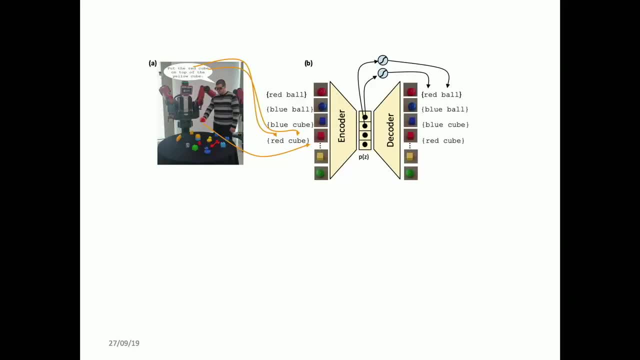 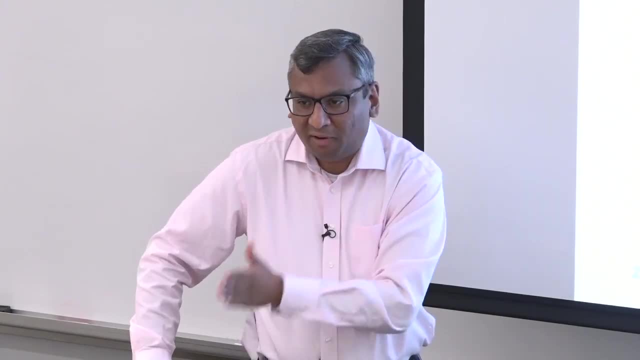 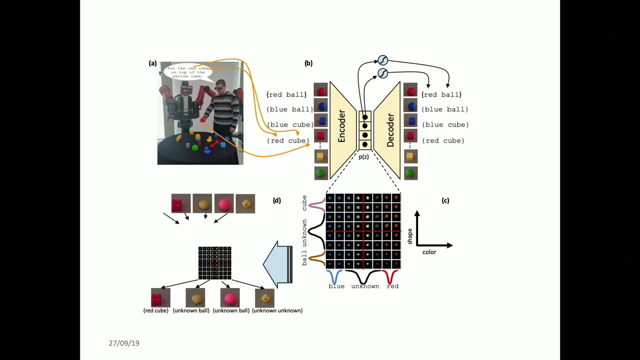 So what we did was we took what is, by now, a fairly well understood and well used architecture, which are autoencoder models and, in particular, disentangled versions of autoencoder models such as Beta, VAEs. Then what we did was to force these models to. 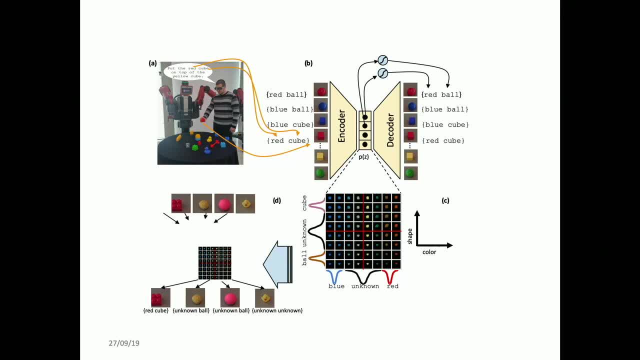 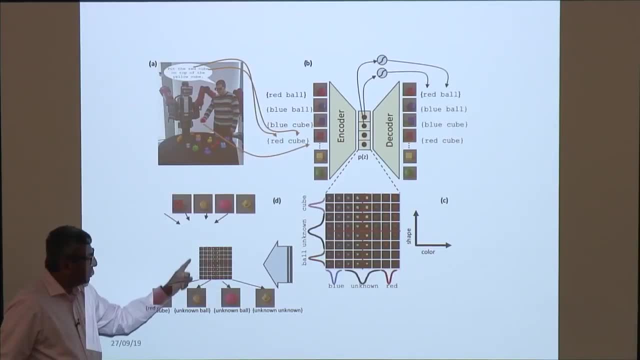 perform a classification task. as the end result, What we want from all of this is that I'm giving you a collection of descriptions of objects, So what you see in this matrix is just like kind of sprites with different colors and shapes. What I want to force you to do is to organize them in. 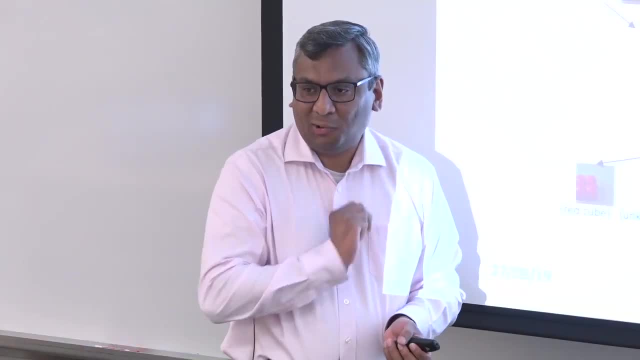 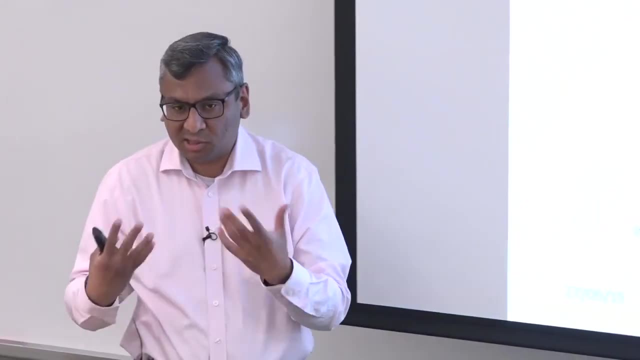 such a way that if I forced you to classify using one axis, then you do a sensible classification. The only way to do that is to then get size this way and shape this way, and so on and so forth. This is to make the basis vectors be. 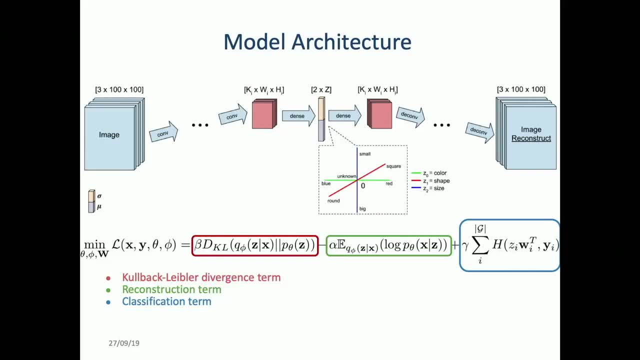 meaningful. So the way that we construct a model looks something like this. So this bit- it's a fairly classical description of how a Beta VAE type model would work. What we've done is to essentially add the classification term at the end of all of this. 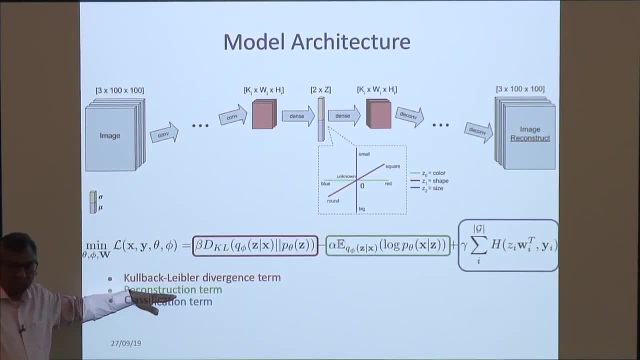 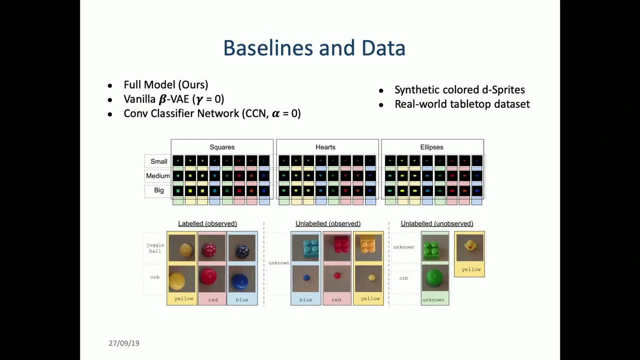 So we're saying that you still have to look at the KL divergence, you still have to reconstruct except, I also want you to do a good job of classifying using your basis vectors. If you do that, then what you end up with are classifications. 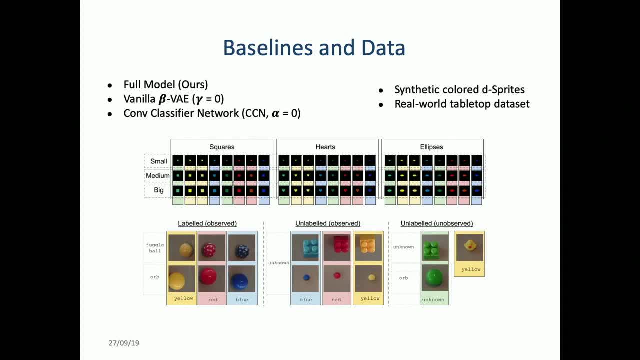 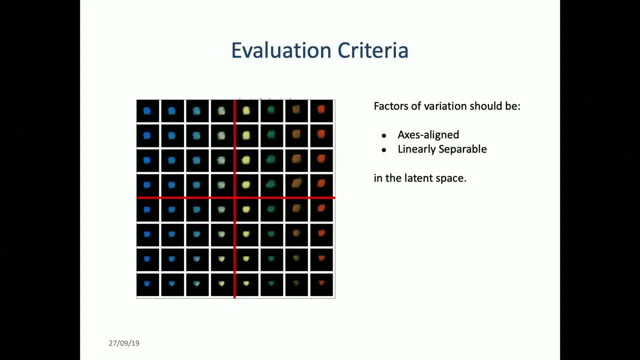 that pick up the labels we really care about, which is size descriptions, color descriptions and so on and so forth. So we did that and what we found is that if you do it the way we've done it, then you actually get pretty good classification performance. 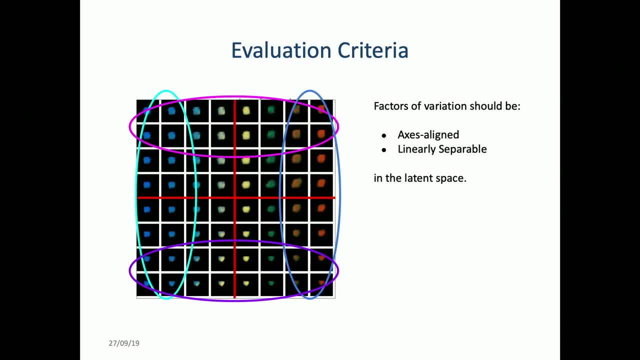 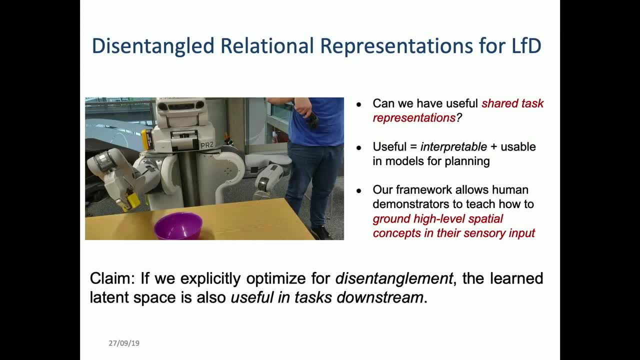 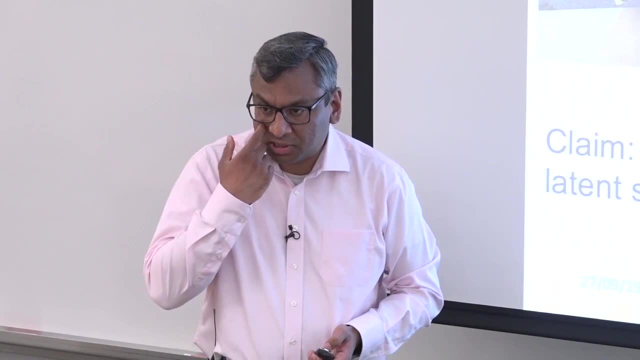 and that actually gives us human interpretable output. But then we went on from that and in our current work what we are looking at is to try to use these representations inside the action loop. So we want to learn disentangled relational representations. 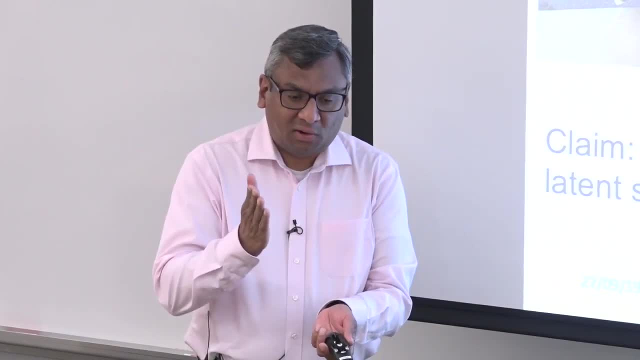 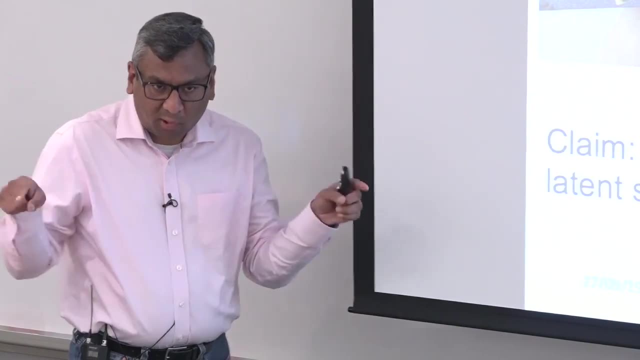 where the relations correspond to things like: is an object on top of another object, is the object in between something else? These are all labels that we want to learn, and we want to learn them as axes in this latent space, so that we can then map that onto planning later on. 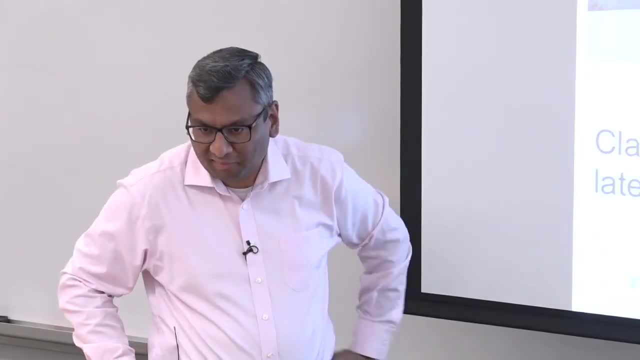 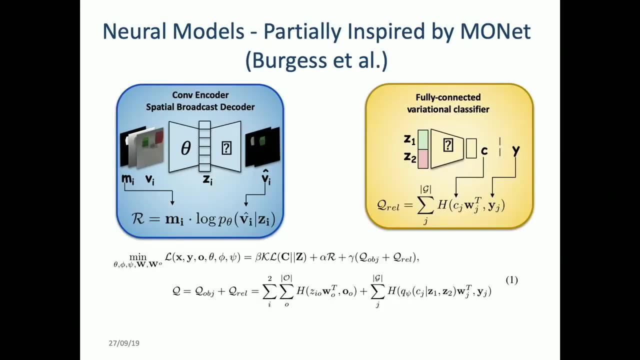 So, without describing the model to you, in the interest of time I'll just show you the videos of what we are able to achieve from this. I'm happy to talk about the model with you if you're interested in it. So here's what it lets us achieve. 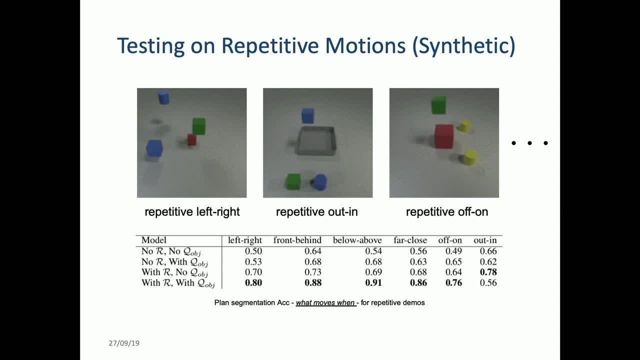 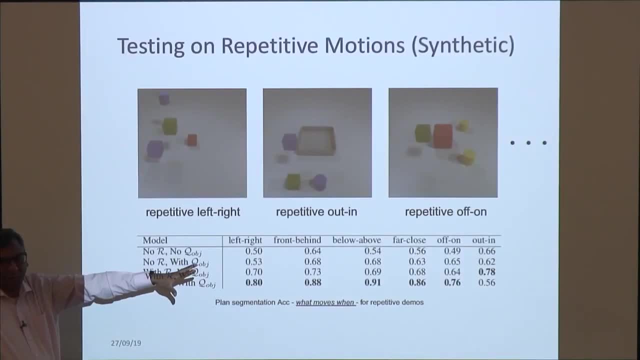 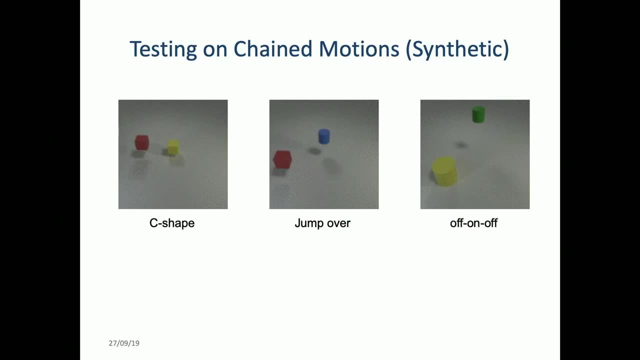 So it lets us cluster things in terms of when the description has something to do with moving an object from one region into another region, when the object has something to do with putting one thing on top of another thing. So these are all, for us, basis vectors of descriptions of a concept. 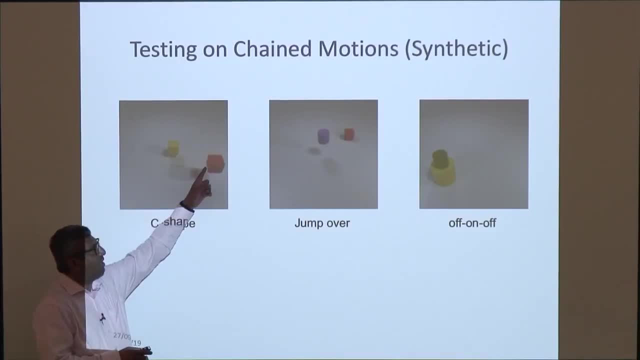 so that when the person says, put it on top of, it's invariant with respect to what the object is, it's invariant with respect to the position. but you've discovered that there is this notion of on. So we've learned a number of these things, such as jump over something. 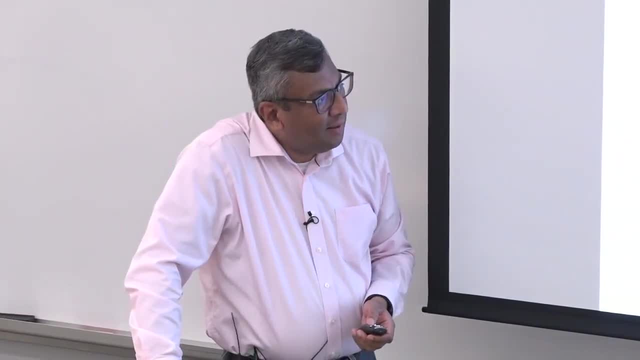 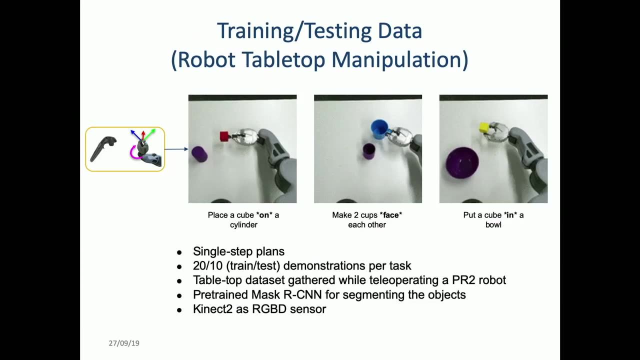 go in a C-shape, go from one thing to the other, and all of that is now allowing us to do things like this, So we can take an instruction, such as: put a cube on a cylinder or make two cups face each other. 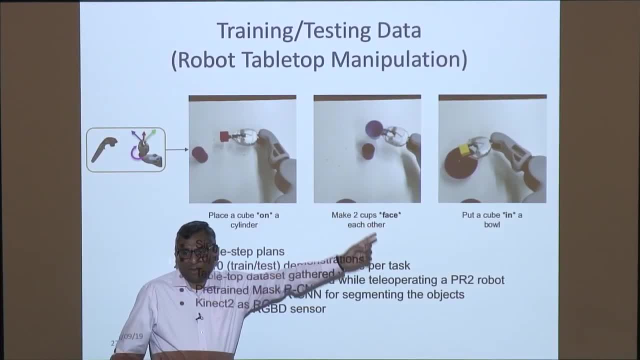 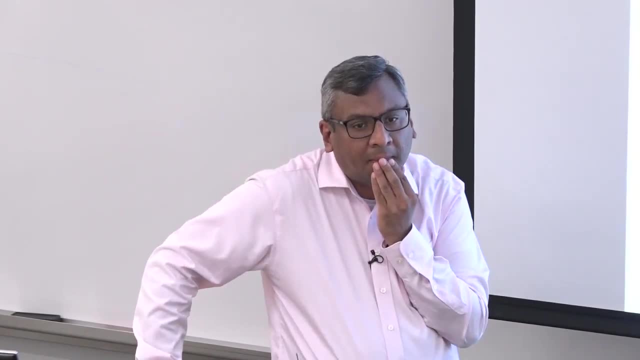 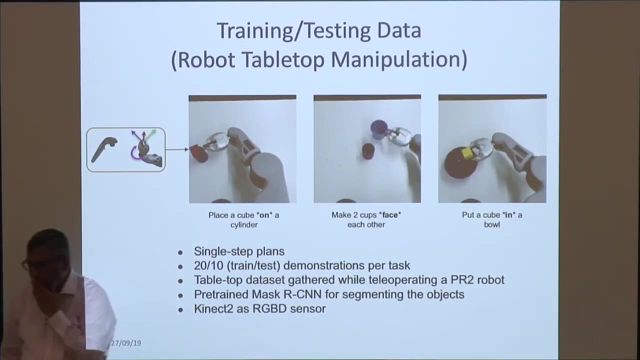 and then the robot actually performs those tasks when we're done with it. So I just want to ask you a question. in the previous slide those were just exploration of one dating variable. That's right. So the objective there is to use the model in a closed loop like this. 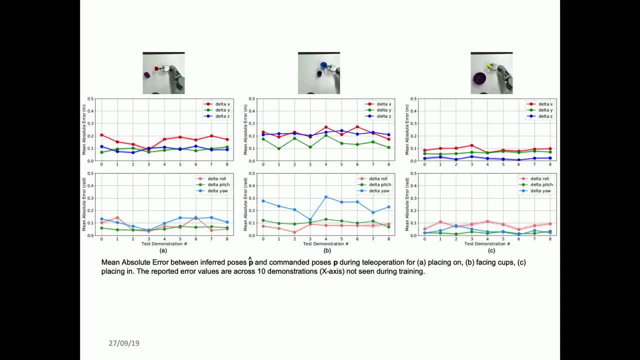 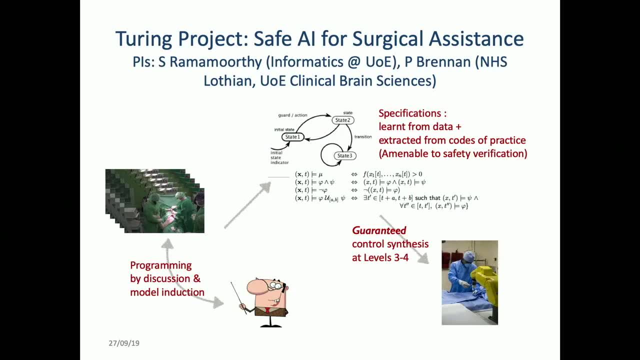 So I want to end, then, by bringing all of this together and reminding you that, for me, as a roboticist, when I look at all of these problems, what we have to do is to solve a collection of interrelated problems, where each thing drives the requirements of 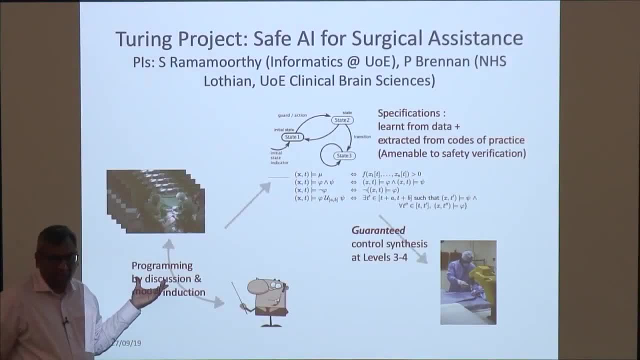 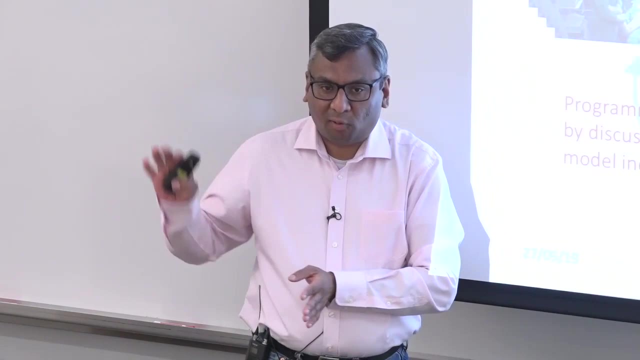 another thing. So we want to do learning from data in its very classical sense, except the data is relatively limited and the thing we want to learn typically is to extract what look like specifications. We want those specifications to map to representations that other people in the domain have. 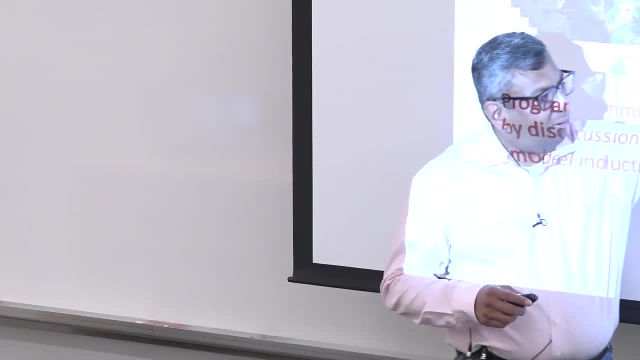 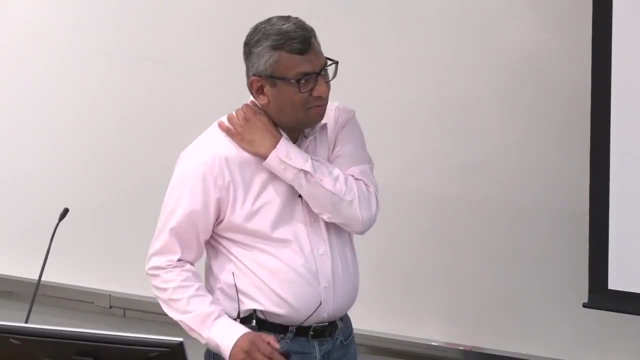 already thought about before and can do reasoning about, Then we want to find ways in which we can somehow enforce that in the policy learning loop, So I wanted to end, then, by showing you an example of some current work that we are trying to do. 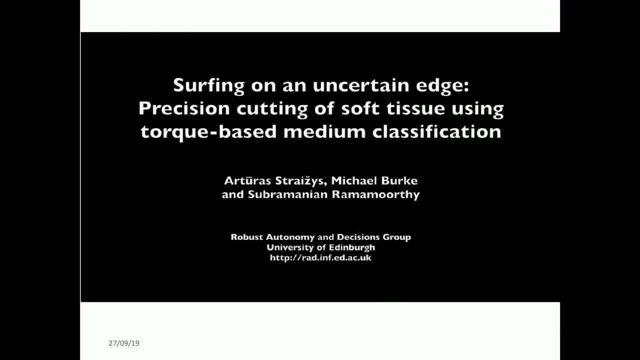 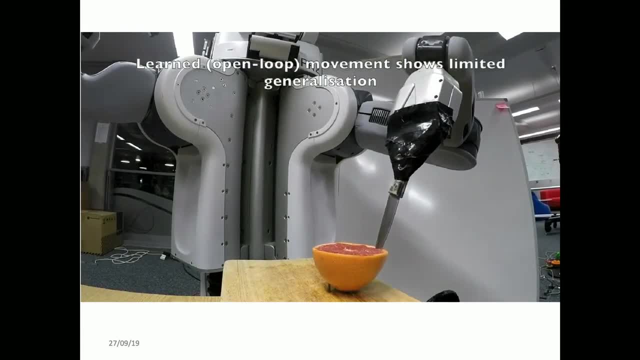 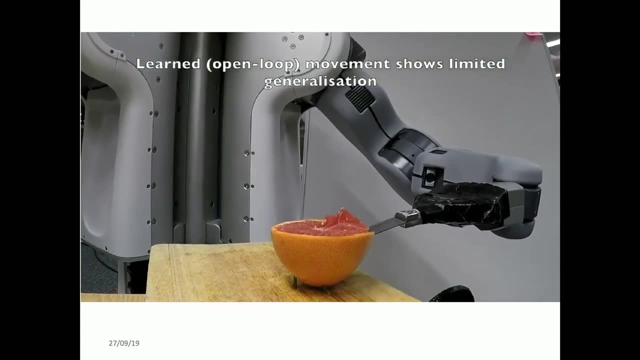 So in this video you see that fruit cutting task again. So this is what the person is showing the robot. If you just naively copy what the person has shown this robot, you find that actually it does pretty badly, which is good for a machine learning person. 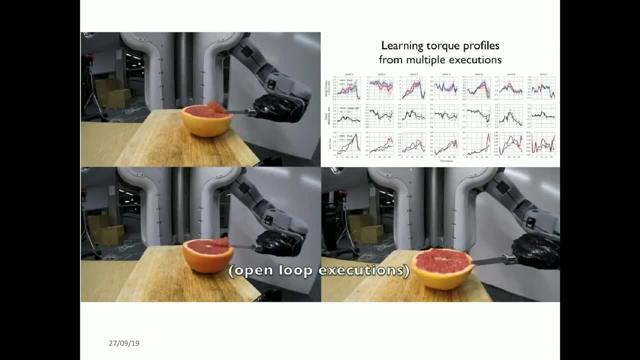 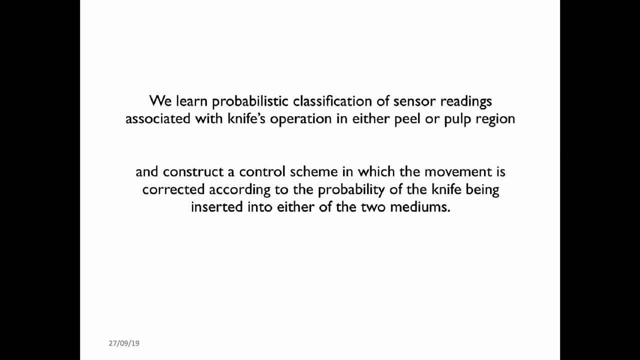 because it says there is some need for learning here. So these are just naive, open loop learning. So if you just said, okay, I'm going to learn how to do this, then you find that that it's actually pretty hard. So the way we solve this problem, 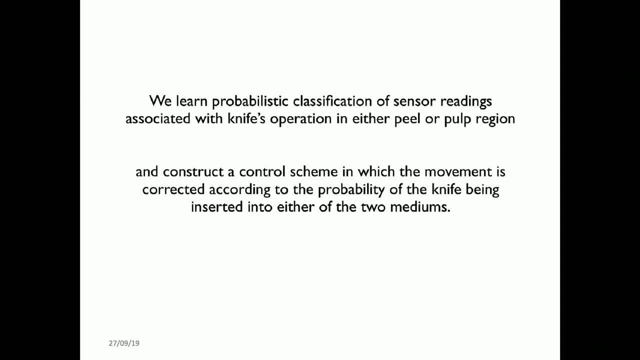 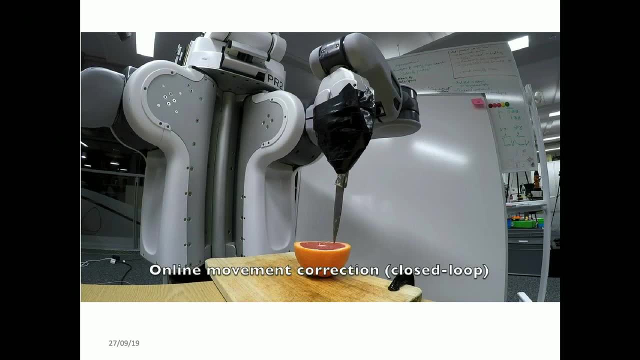 it's quite interesting from a cognitive perspective. So, because we have no other perception of where the fruit is and where the peel is, the way we solve the problem is that the cost function that the robot has is to classify whether the trajectory is going to get stuck in the peel. 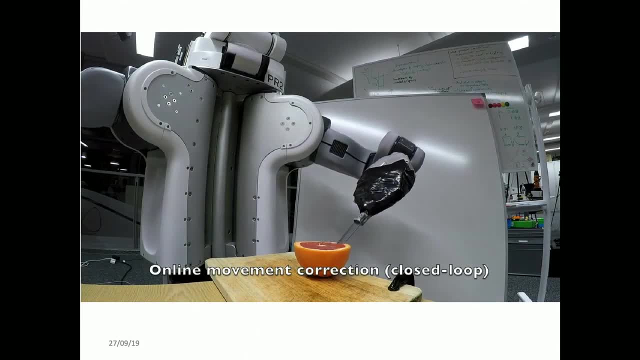 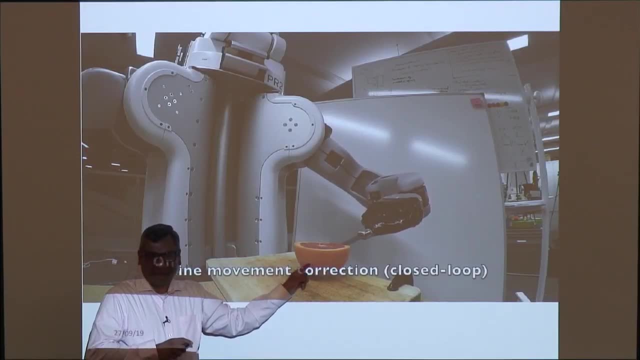 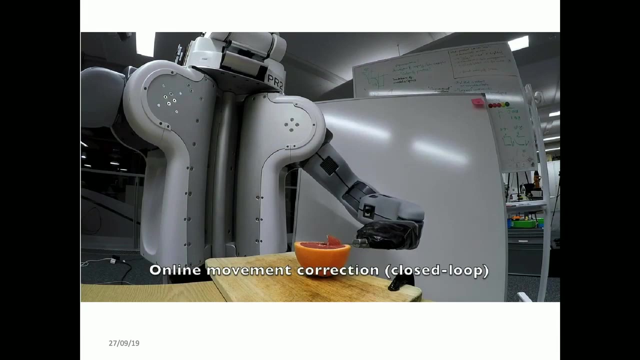 That classifier, by the time it gets good at predicting whether it's going to get stuck in the peel and get a bad reward, will end up giving you implicitly the shape of the peel. So then, if you give that as the parameterization of what this robot has, 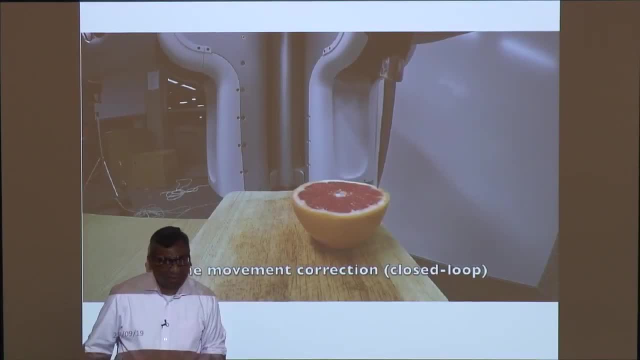 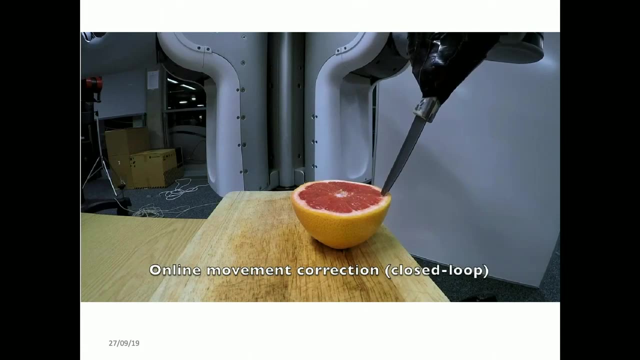 it figures out pretty well how to exactly scoop only that bit, and it figures out all the other stuff about how to control the forces and so on and so forth. So this is a typical task that we are going after. It's fairly challenging from. 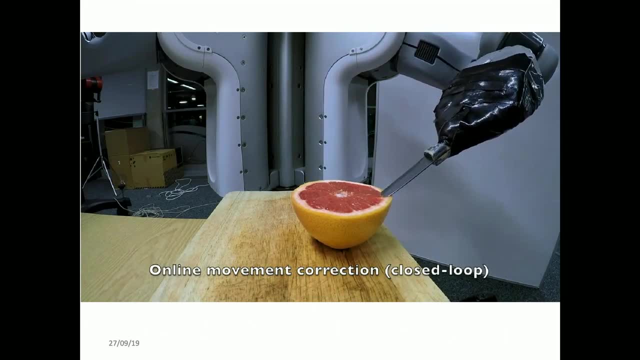 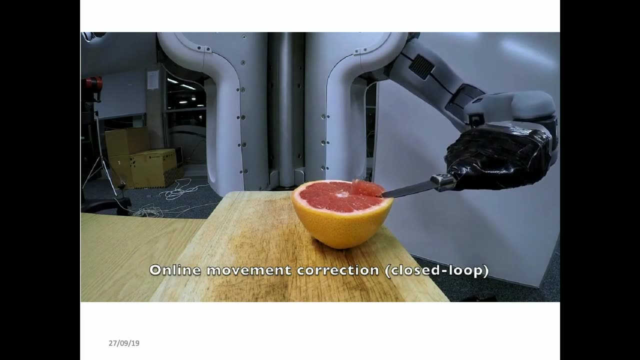 a robotics point of view, because the object is quite high-dimensional. The underlying physics are quite interesting in that it's not immediately obvious what to parametrize and what not to parametrize. So we're playing with all aspects of what simulator to use, what descriptions to use, and so on and so forth. 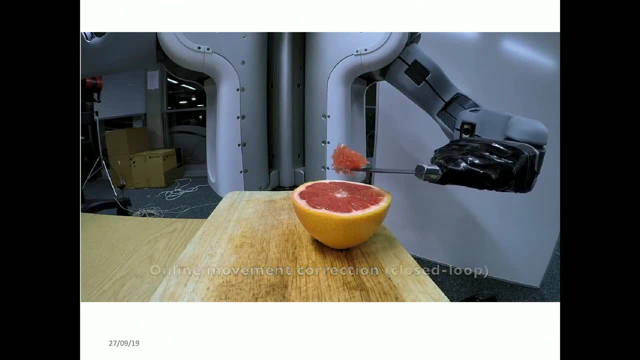 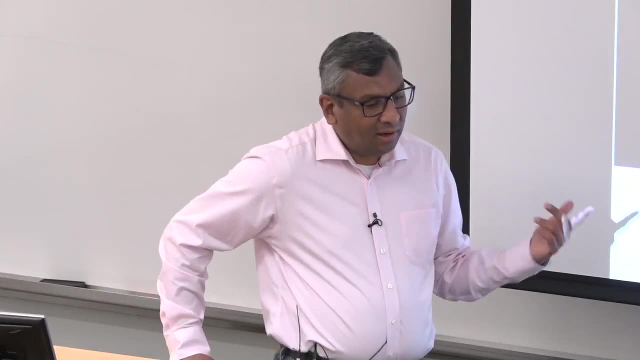 but also what specifications to use. So, as I said, we are only playing around with fruits because we haven't gotten around to phantoms of brains, which is what we really want to do. So our end goal with this project is to work with 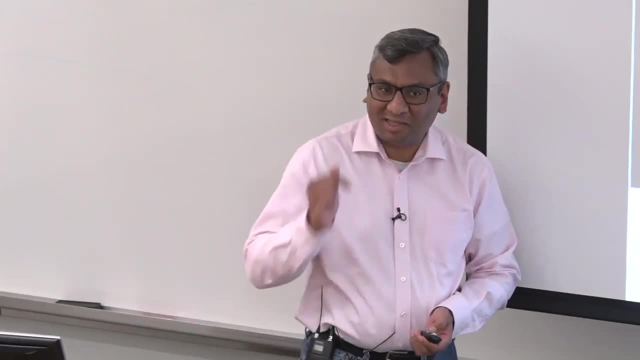 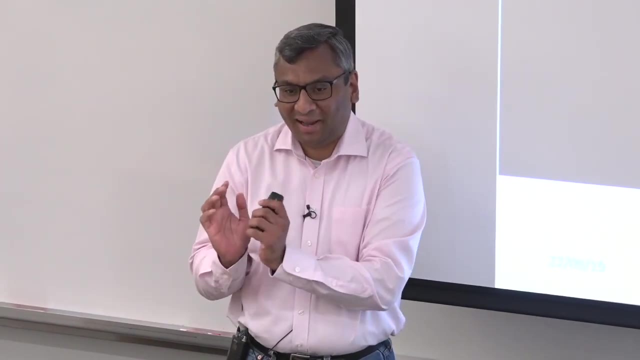 actual surgeons who are doing tumor removal and to do exactly this process and the objective function there is to try to take only the tumor and not the rest of the healthy tissue, which if it's in your brain then even one millimeter matters. 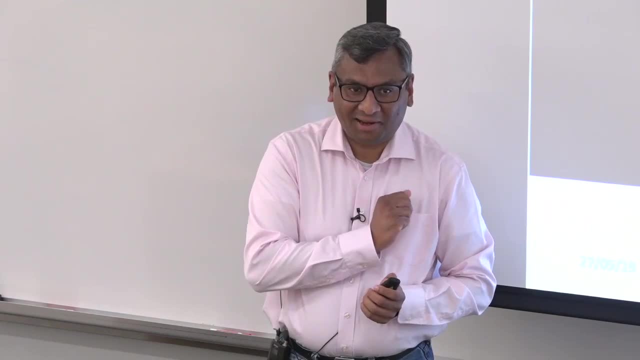 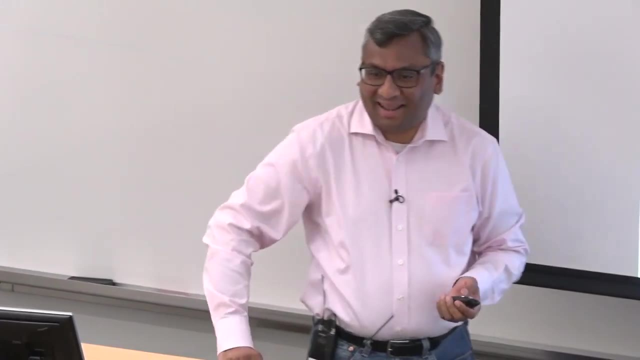 Safety specifications are important, so don't go near a certain artery. it's literally a life and death matter. So one day, when we reach something like that, which might be 10 years away, all of these problems are going to play a role in that. 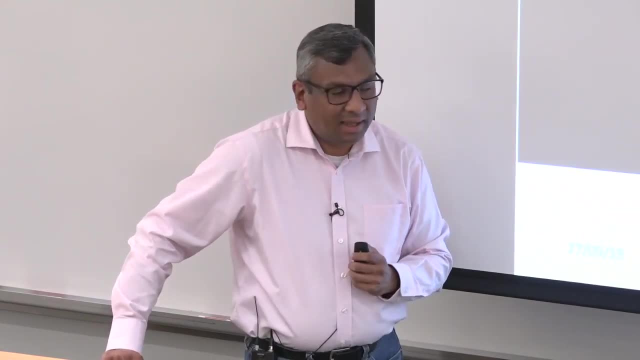 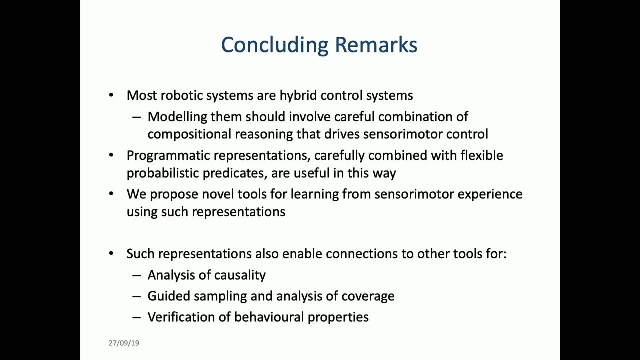 So we're taking baby steps towards that and trying to see how we can line up all of our robotics technology towards it. So I wanted to end with a few concluding remarks, which is that, having worked in this area for quite a while and having looked at lots of different problems, ranging 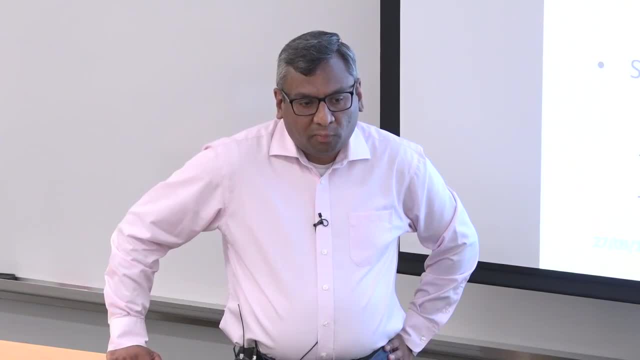 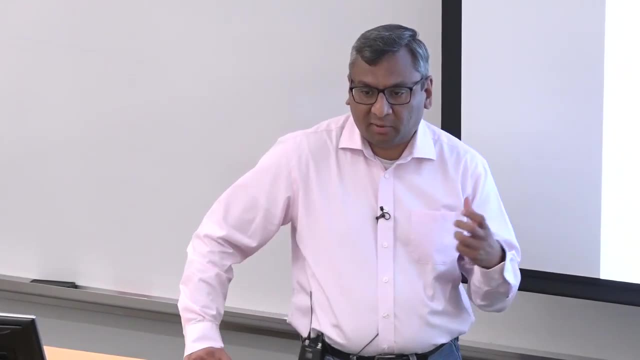 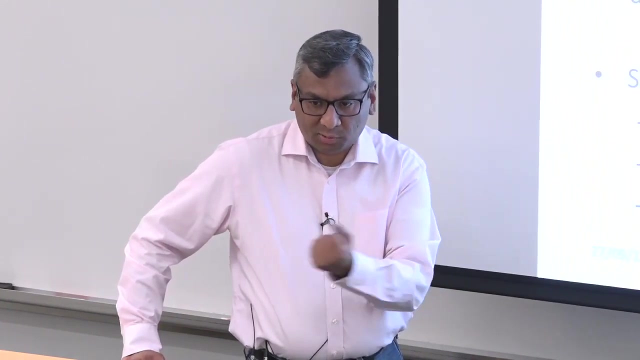 from locomotion to today, manipulation. we believe that representations like hybrid control systems are fairly powerful with respect to describing what you want in the task. So the hybrid control representation is a marrying together of low-level controllers with higher level switching or programmatic structure. 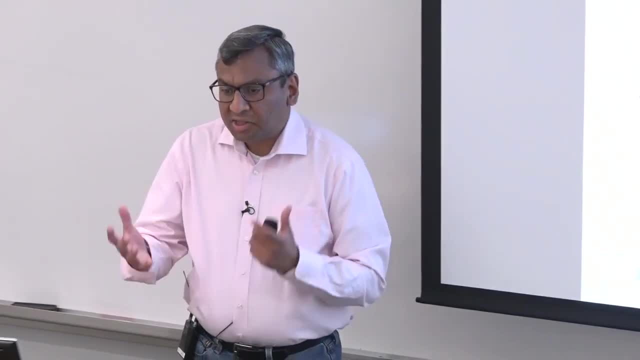 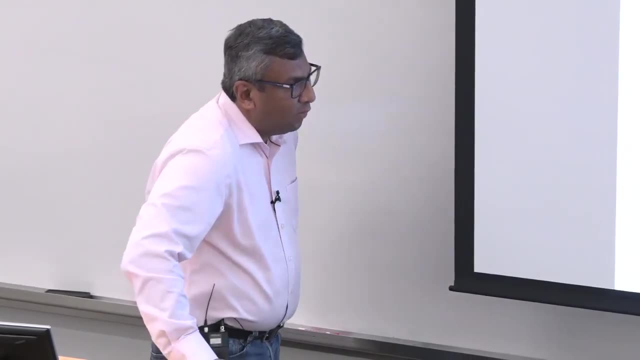 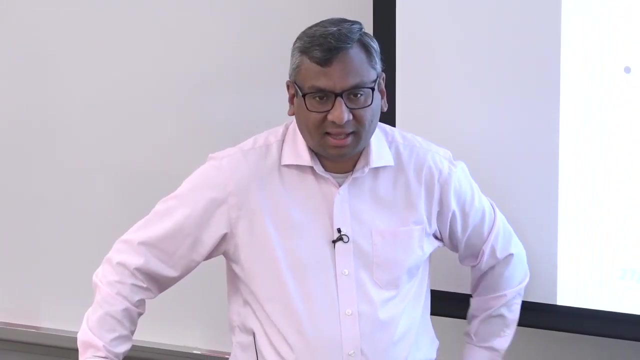 So if you look at it, then all the results are presented to you. in one way or the other marry these things together in different ways. So what we're looking at is ways in which we can define models that can do a good combination of these. 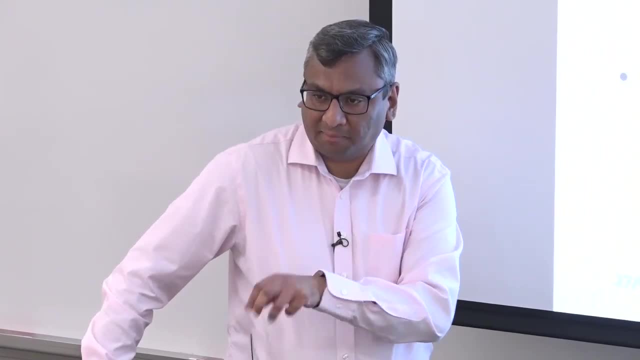 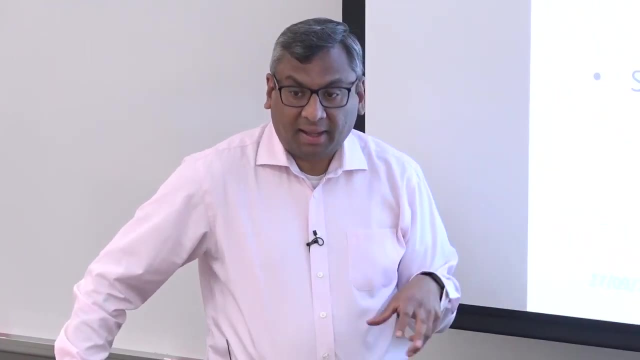 and then asking the question: what are judicious choices around them? The reason we want models like this is because we want to do a number of other things that, from the application domain point of view, are absolutely essential. You want to be able to reason about causality. 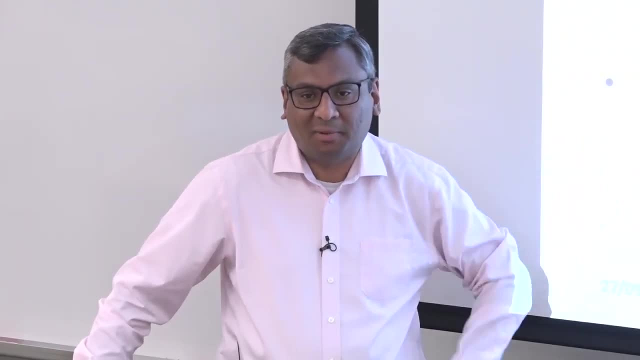 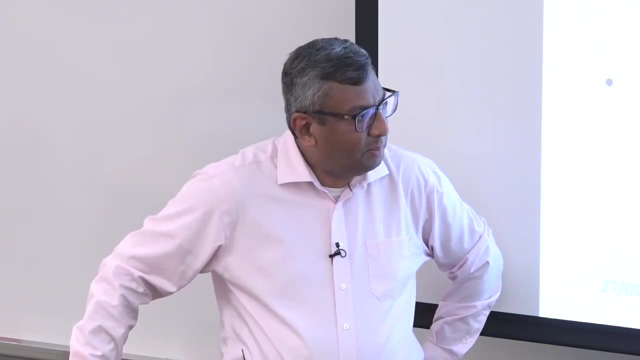 You want to be able to do coverage-based verification. You want to be able to ask about long-term behavioral properties such as: will this controller do this or how often will it do this? So there's no way you're going to deploy serious applications without answering these questions. 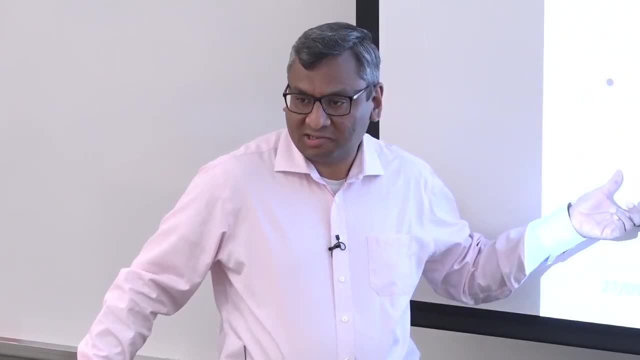 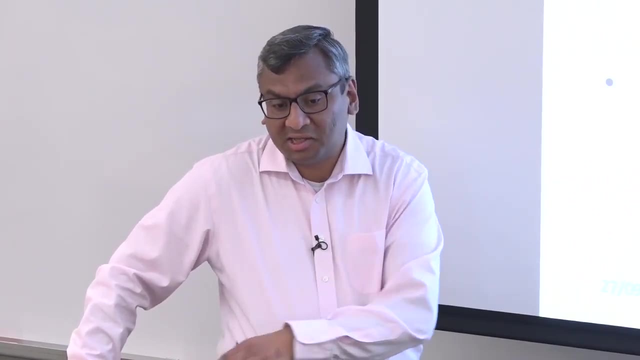 Having representations like this allows you to answer such questions. So what we are trying to do is to come up with tools that gets us there, while still doing everything else that we love about data-driven ways of thinking, about model learning. So with that, I'll stop. 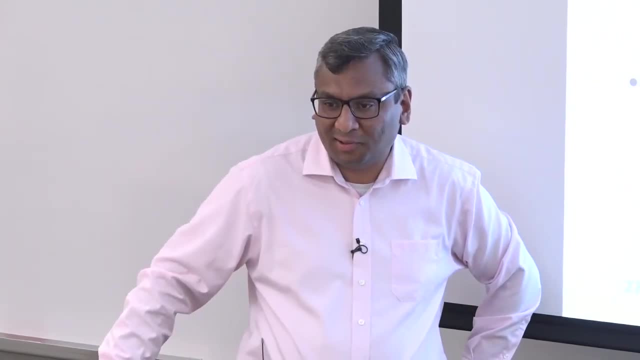 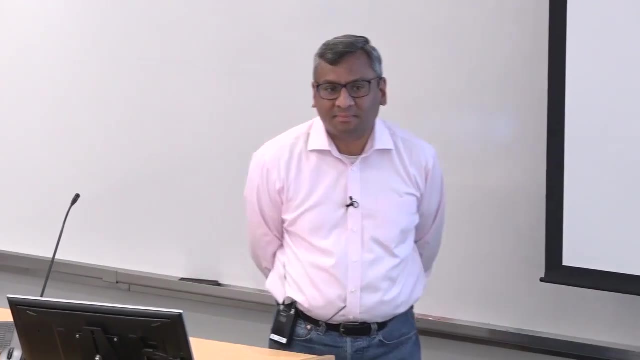 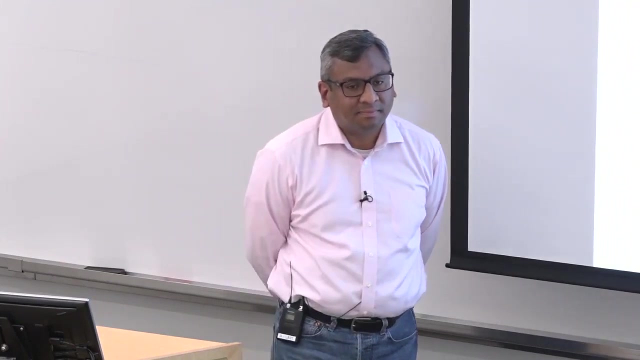 I'm happy to take questions now and also to chat to you during the rest of my visit, So we have a few minutes for questions. So I mean, I would like to pick your brain in terms of what do you think is the right visual representation for generalization? 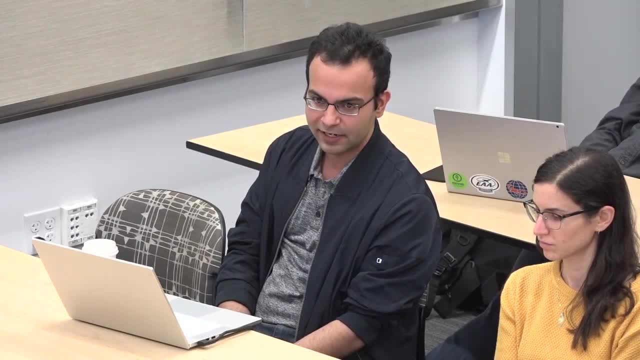 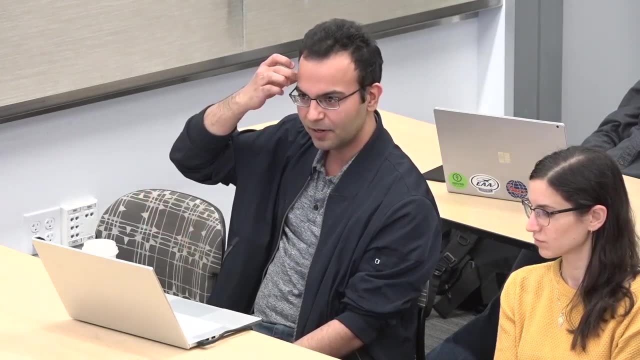 For all these tasks, because inherently all of these are sort of 3D and also I think the approach orientation matters, because you want to grasp something right. So it's a six-step course, But I think at least in the first two. 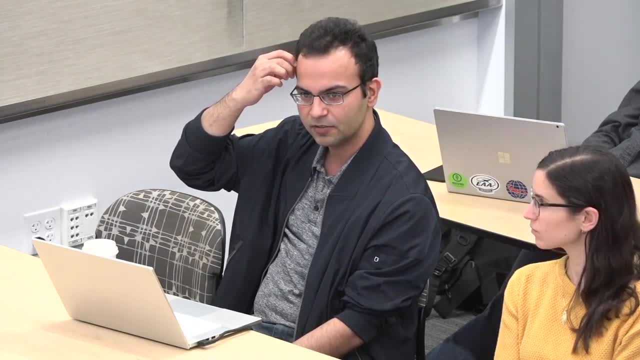 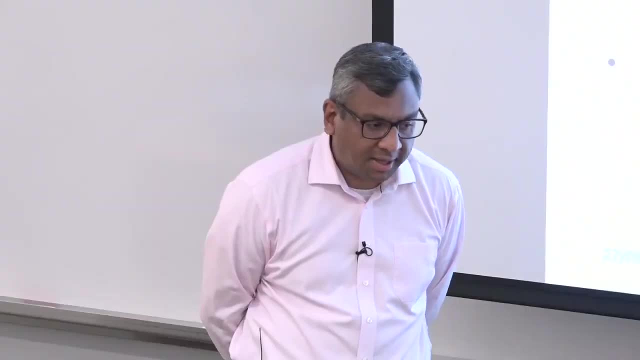 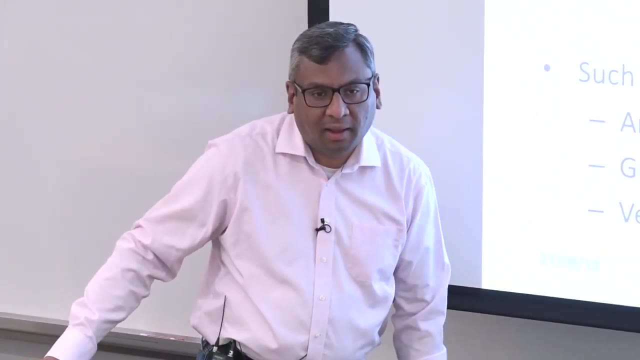 three books. it was 2D coordinates and also with a fixed camera view, So I'm not sure how well that would generalize. That's absolutely true. We do them with fixed coordinates simply because our focus of attention has been on other things. We could quite easily get our robot to move around. 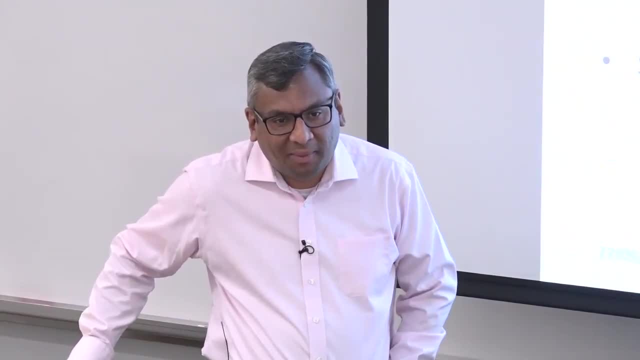 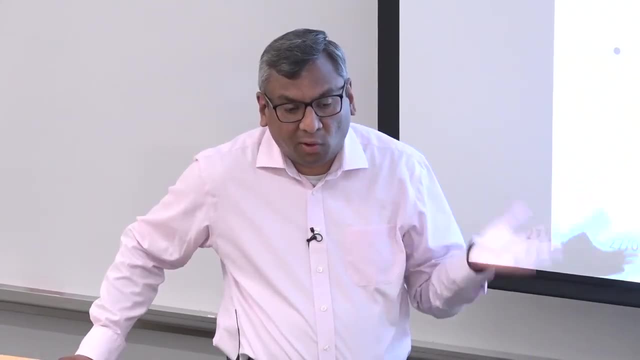 In fact the robot we use, PR2, does move around, So we could easily make that be a multiple coordinate view kind of problem. But you're exactly right. So in almost all the problems we are working with it has to be a three-dimensional representation. 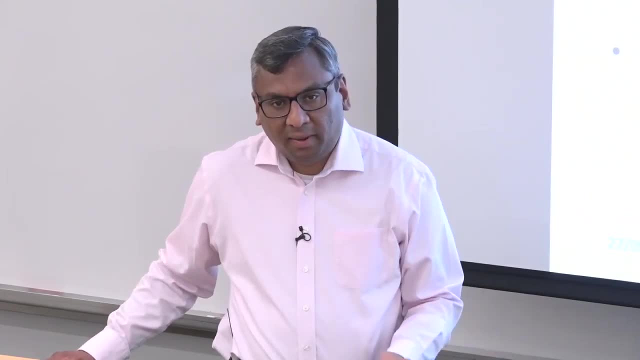 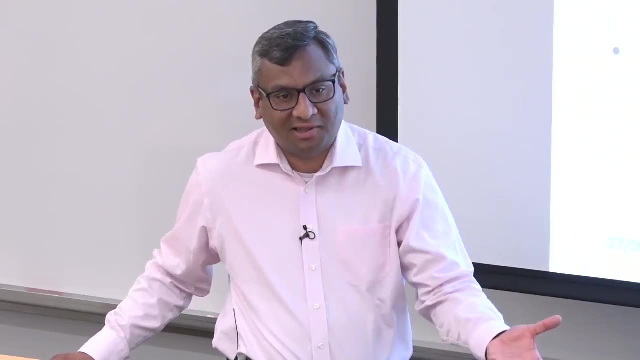 and it has to be a representation that can somehow be correlated with the rest of what you know about physics. So if you have a 3D representation, you can reason about physical laws and the way that you're comfortable with. So there's no getting away from that. 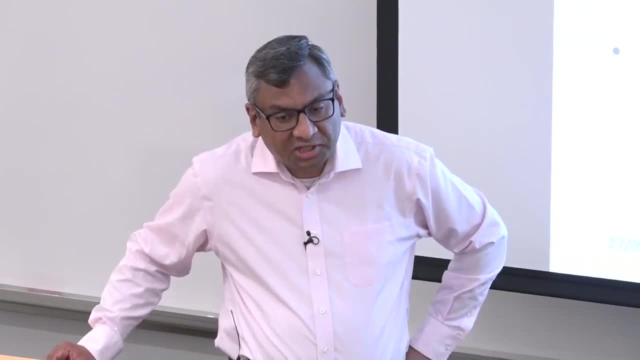 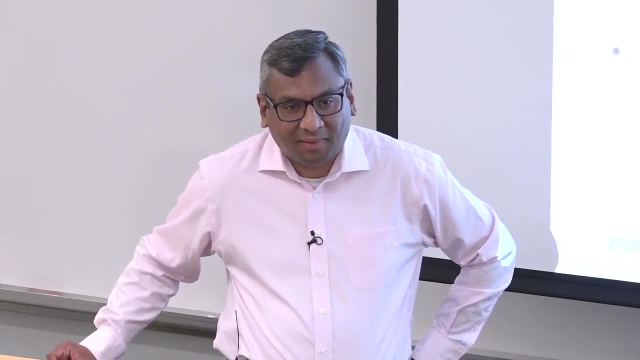 The bit that's really thorny for us at the moment is that vision is probably the best understood and best research modality, but everything else we want is not in that channel. So all of the haptic information is missing from vision and the correlation is very weak. 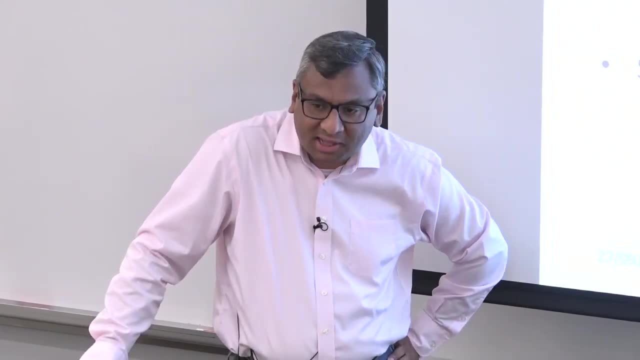 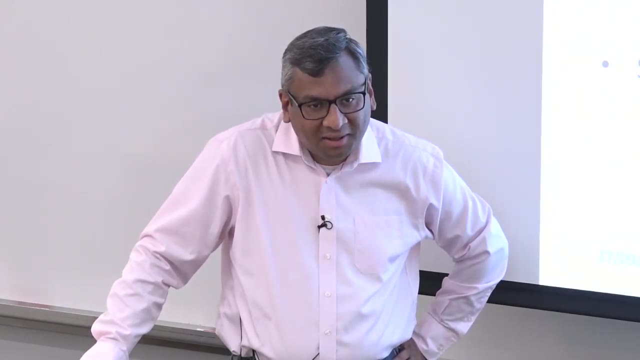 So that's something that we're thinking quite a bit about, and we're looking at new sensors and so on. Then that brings us to the question that there might be many, many properties. you want to learn about objects. If you had mass asymmetry in a ball? 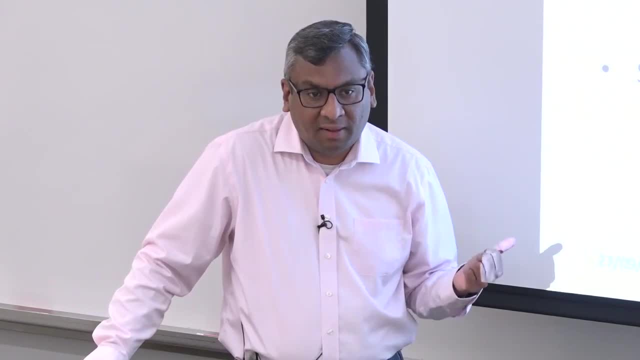 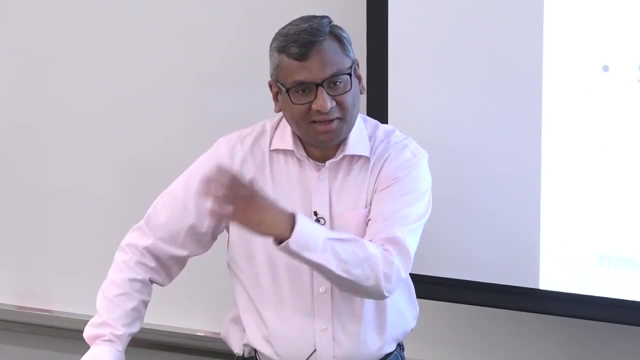 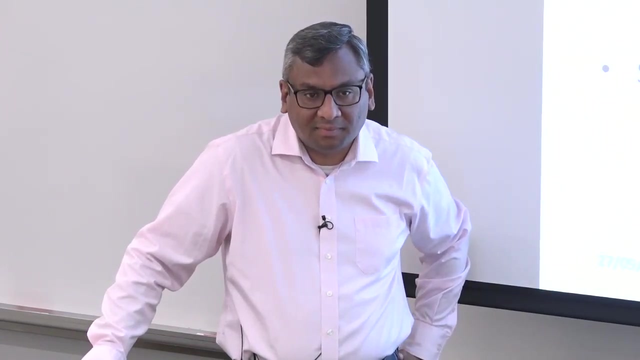 it can only really be picked up from a dynamic exploration. So there's business of going from single-frame labels to exploring and having a mental representation that's almost a full simulator is where the big challenge is, in my thinking. Yeah, I guess you care about things like stiffness and all that. 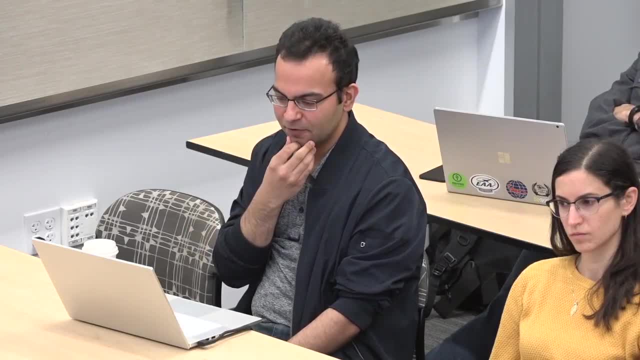 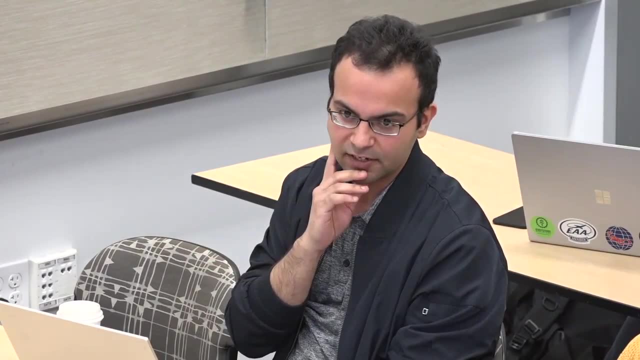 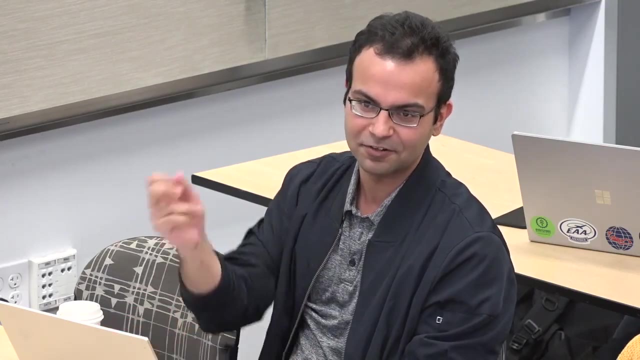 Yeah, Meaning like forces. So I guess my other question was for physics: what is what have you learned from, say, playing with all these different physics engines? I guess, because none of them, I guess, would really represent reality. So at the end, some people are going to learn residual physics or just like. 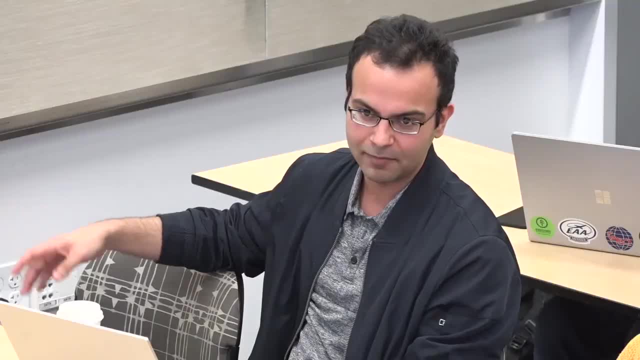 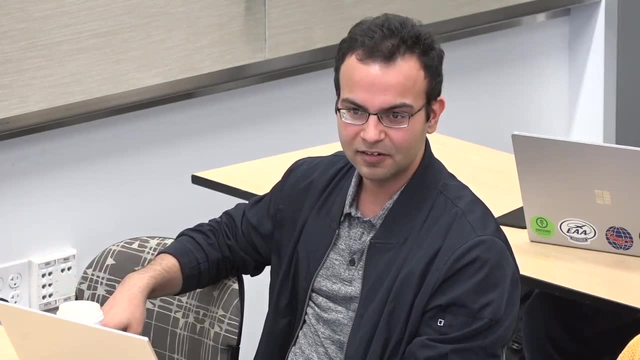 if you have some intuition and you pick the top three top-end parameters which matter for your problem, like I don't know, viscosity or something else, and then doing really up on that, Yeah, So at this point in time I would say that if you have, 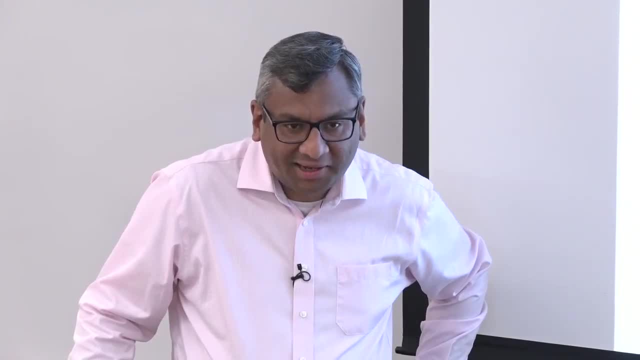 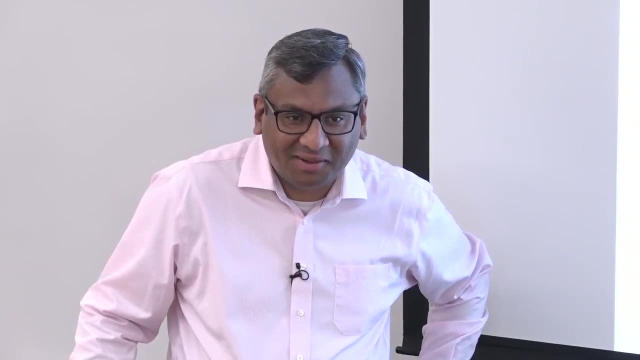 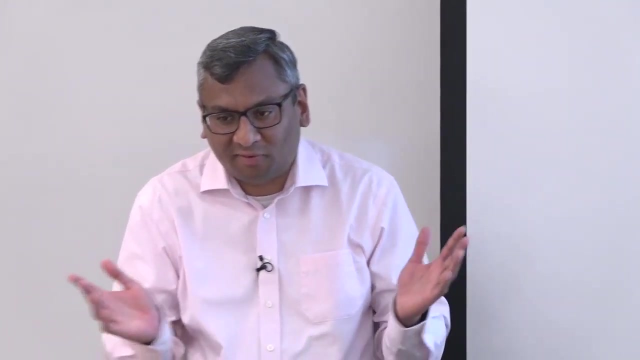 not too much. physical contact interaction simulators are better. If you have a lot of that, simulators are not good. We are in desperate need of much better simulations of that side. Simulators seem to be tuned to the tasks that they were originally invented to solve. 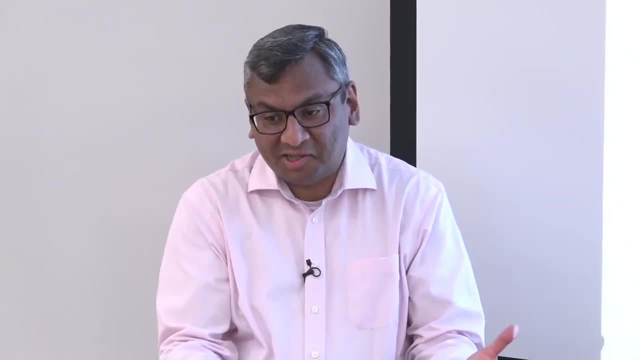 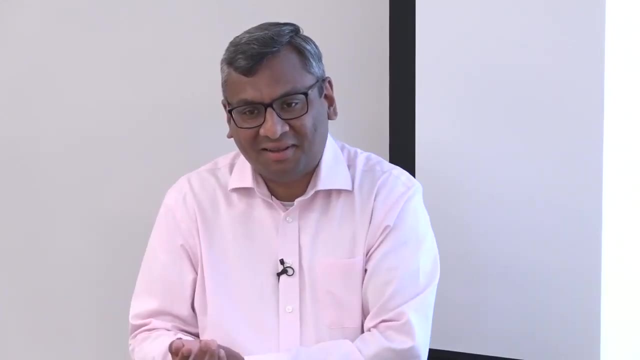 So I mean Mujoko came about from the DRC experience of Totoro. They're extremely good if you're modeling locomotion robots, not so good if you're modeling other things, Then other people. today they're trying to build manipulation simulators. 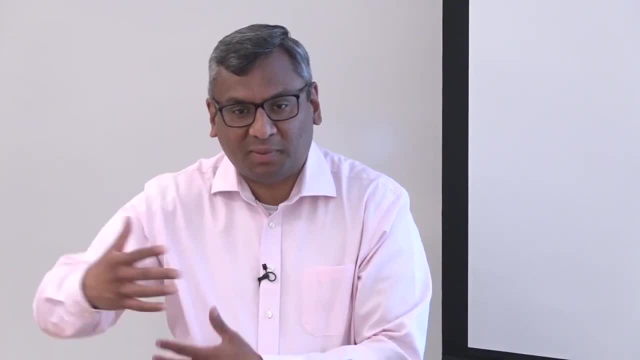 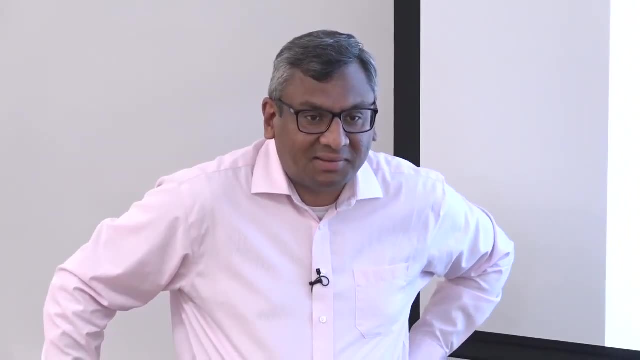 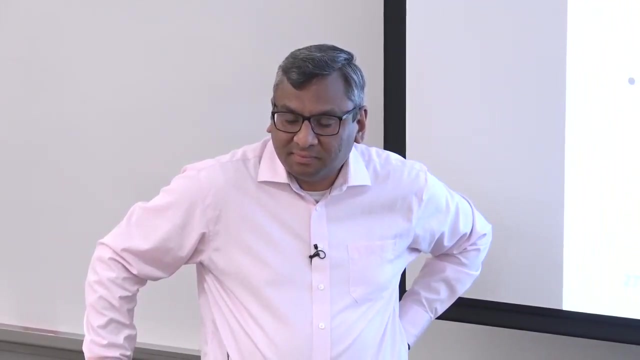 and they're still struggling with. am I solving grasping? am I solving general object properties? So it seems to me like we're still in early days and there's much more to be done. So one comment that struck me was you say how involved the vision is. 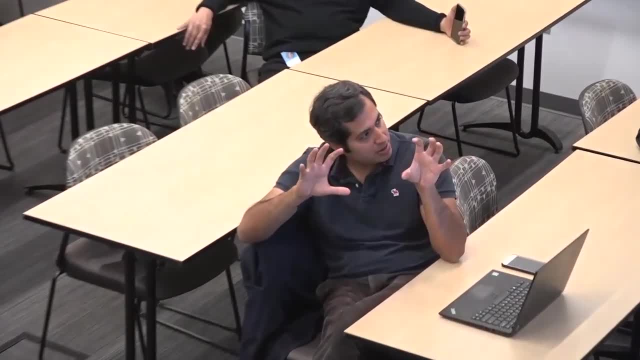 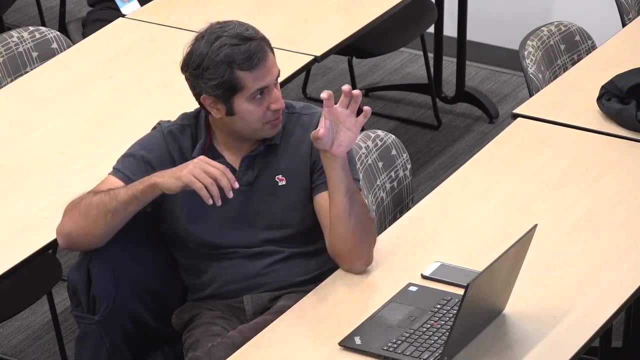 so, for instance, the work that you're doing, where you have a preceptor and you have a policy- I mean given- Exactly in this era of pre-training models, it makes more sense that we fix the perceptor but do learning on the other side of things. 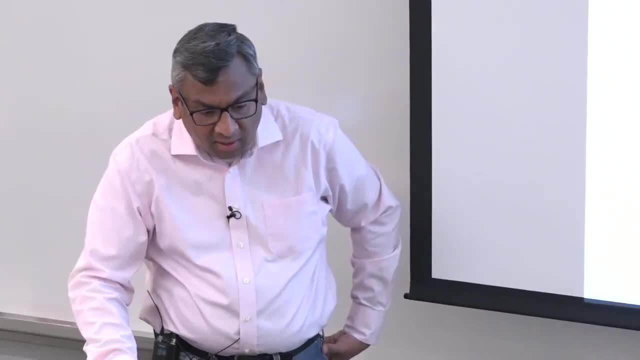 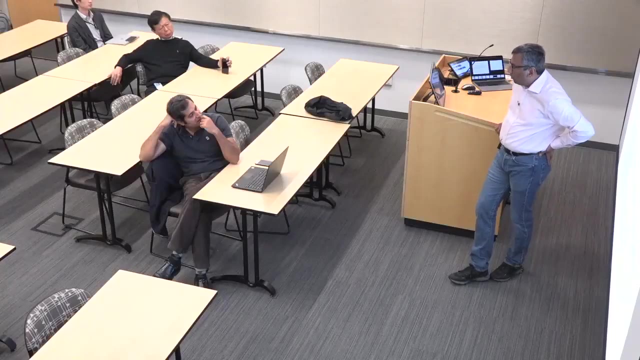 We could do that as well. It's a very good observation. At the time when we did that work, we were more trying to explore how you would put in specifications, So the question came from there. But you're right, I mean in. 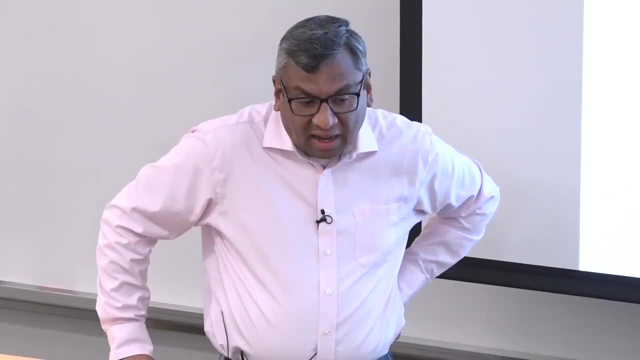 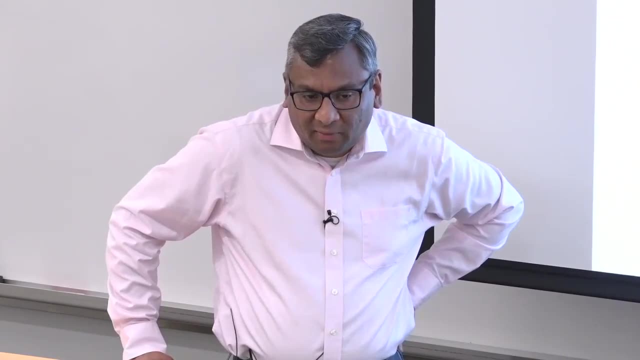 this era of pre-trained models and so on. if you could have, I don't know, very good object detector networks trained over millions of objects all over the world, it would make a lot of sense for that to become standardized and to use it. 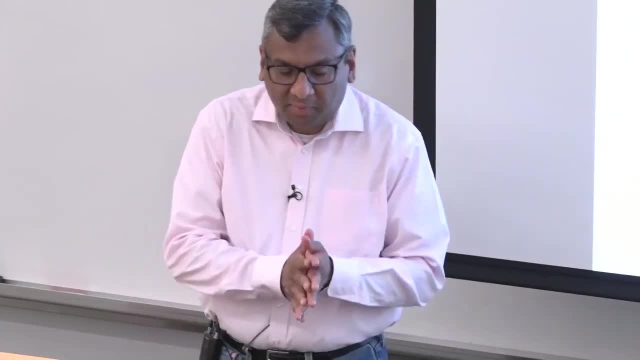 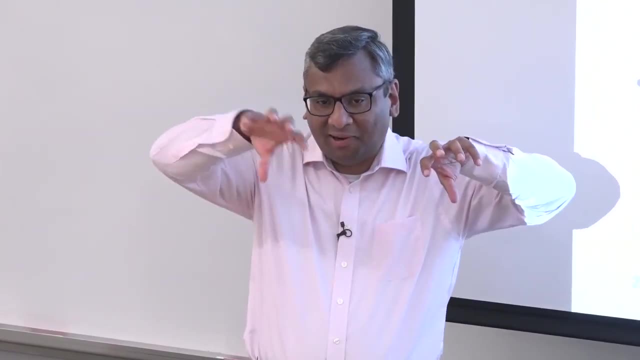 So, in fact, the immediate next thing we were toying with doing with perceptor- which we haven't done- is to then factorize the policy even more and say there's a vision component, there's a learned component, and then there's a structural fixed component. 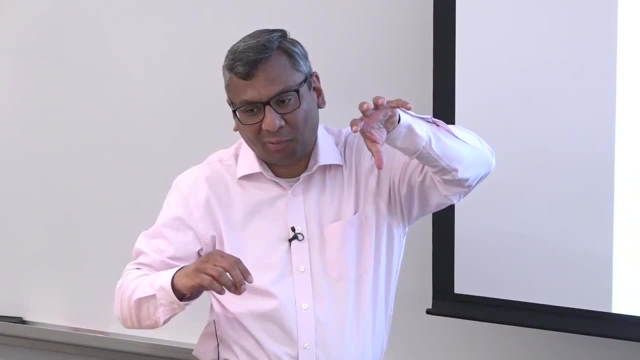 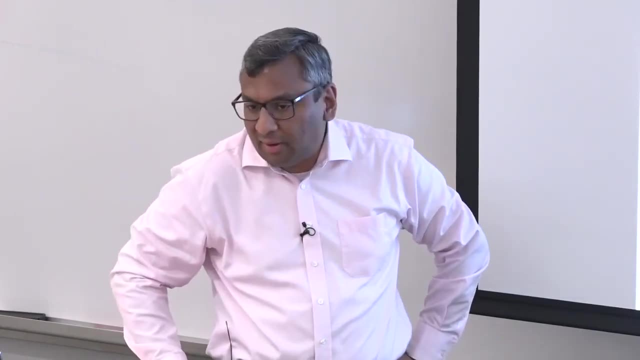 That would look more like what you're saying. So the vision component would be a pre-trained network. there'd be a small level of post-training on the job and then there would be fixed structural insights. That would make perfect sense. Yeah, Also, I'm just wondering how much it. 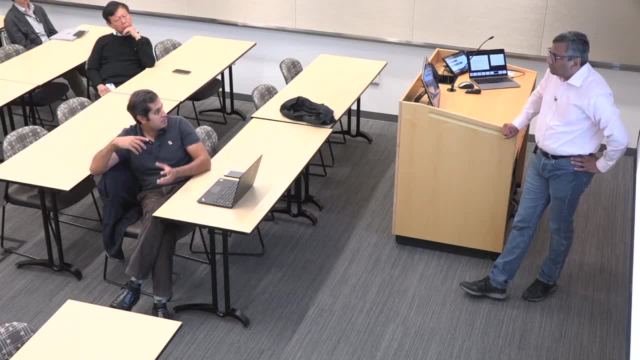 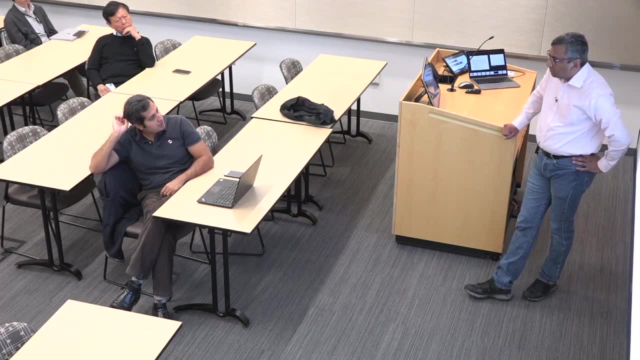 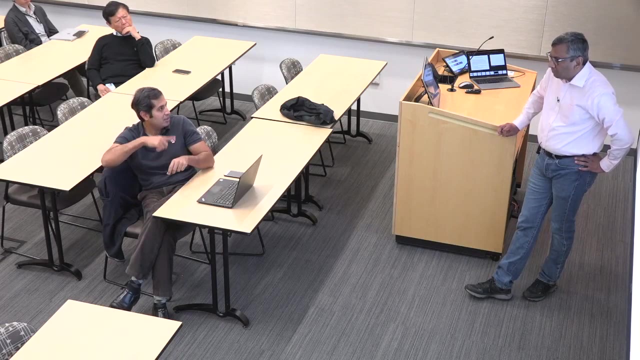 makes sense to train a perception in a reinforcement learning, Because perception I mean sure there's task specific things, but if you can put some human intuition or knowledge into it, you might be able to just do it using supervised learning and then just a little bit of fine-tuning. 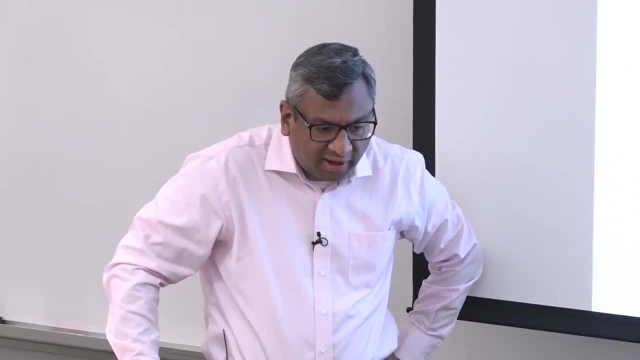 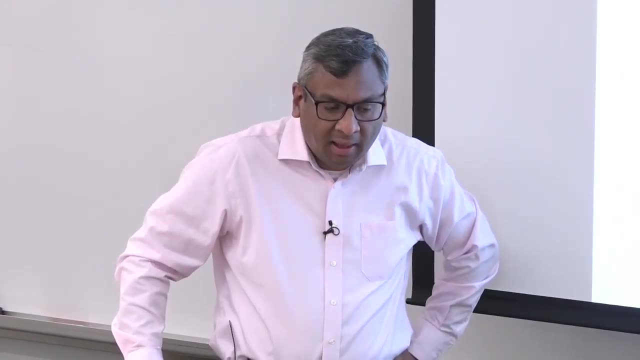 Possible. Yeah, It's possible, Yeah. So in our experience, it's not so much that you're learning perception from scratch- Although, yeah, we did that there because we wanted to show something- But going forward, for me, 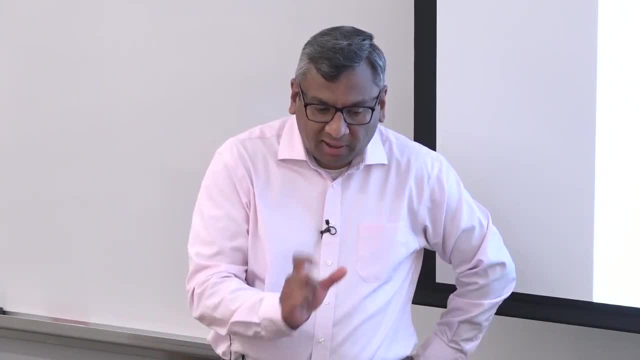 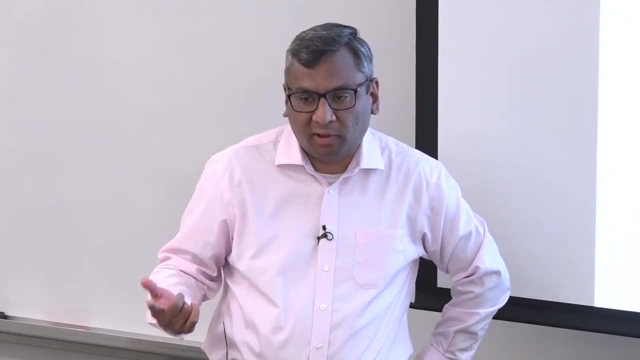 the more interesting thing is you have to leave a little bit of leeway to decide which bit of the perceptual channel matters to your description. That has to be left for the later bit. But how that channel is processed could well be pre-trained. 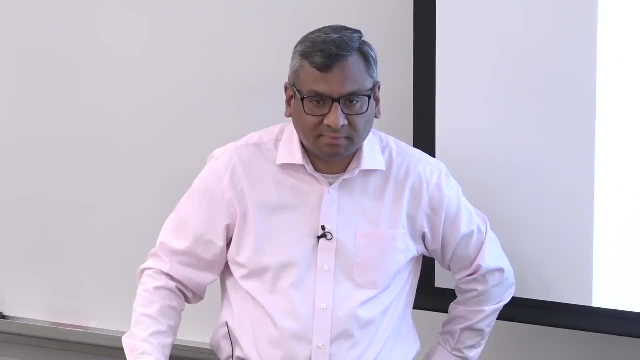 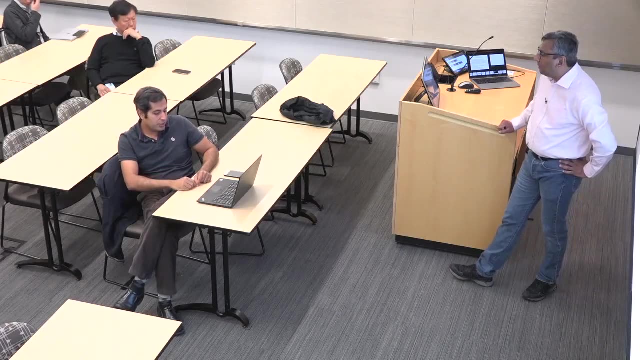 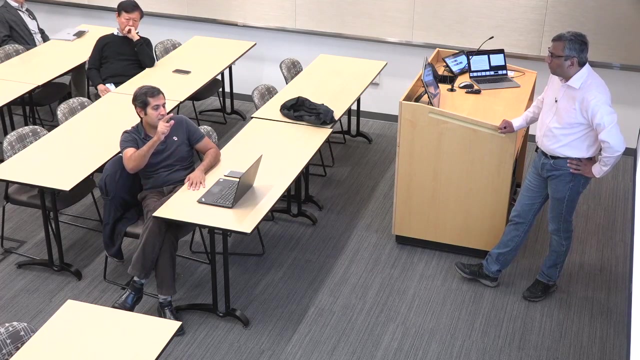 Yeah, Right, Well, there's no other question. I have one more question. Yeah, So the work where you're learning these base level controllers and a sequence of those base level controllers, So a simple task. for instance, if I ask if the task is to draw a square, 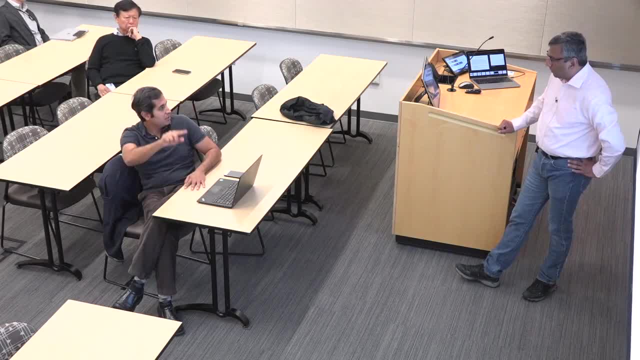 and if I only have demonstrations going one way, Yeah, Right. So basically you are now biasing your controller to adjust to the task, Right? There's no way it's going to find out that you can do a square like these. 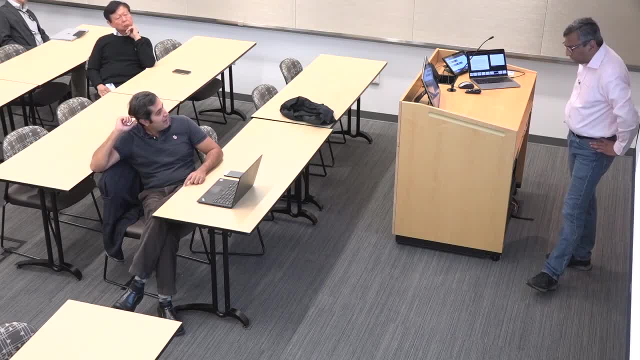 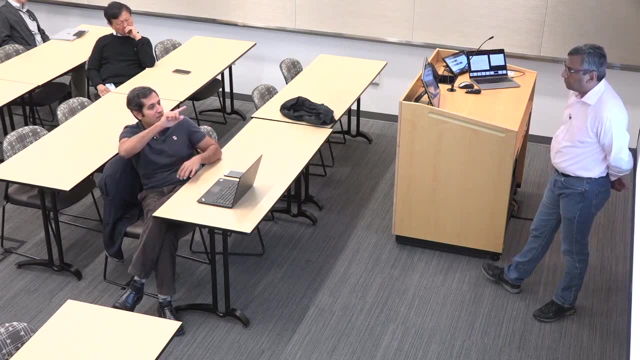 or go the other way or draw. I see what you're asking. I'm just wondering, like those kinds of things, that comes very naturally to us. It's not really about how the movements are done, but it's the context, the complete context. 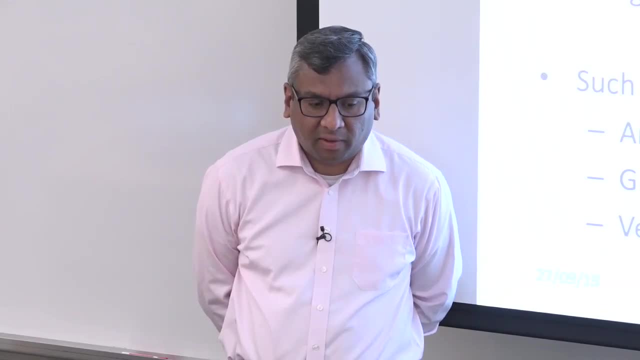 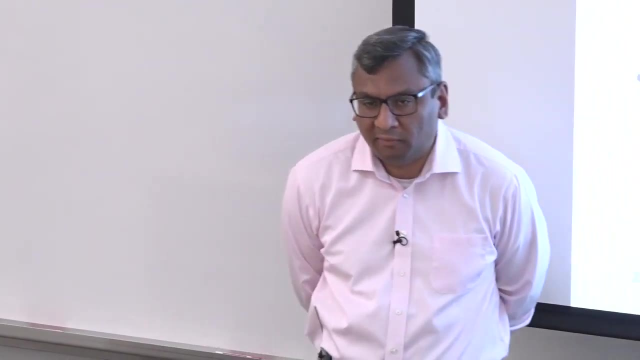 Yeah, So I think that the argument I was making it's in two steps. One is that the learning of the original square is where you do a lot of detailed sensory motor stuff. Yeah, The later reasoning doesn't need that anymore. 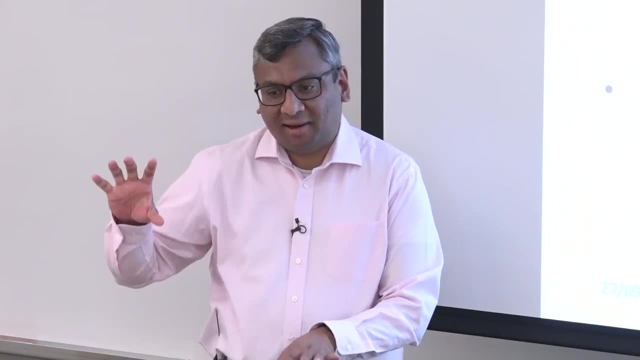 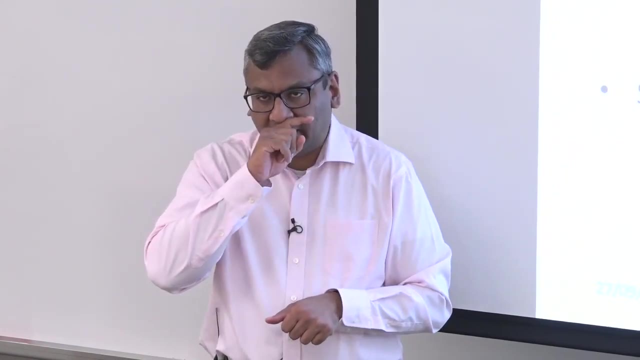 If you've somehow learned all of that, you can reason at this higher level. So if I've learned lots of these, exactly like in my tower building example, where it has learned that there are these four, the observation that those four are the same is.